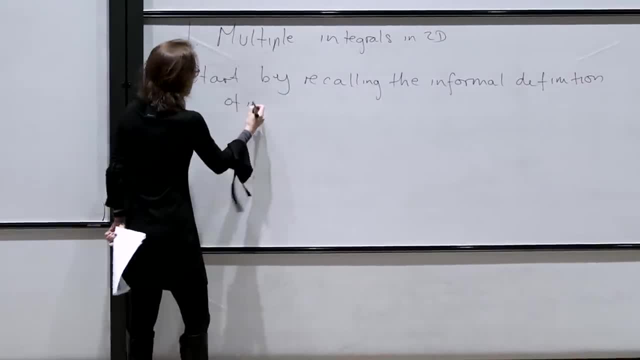 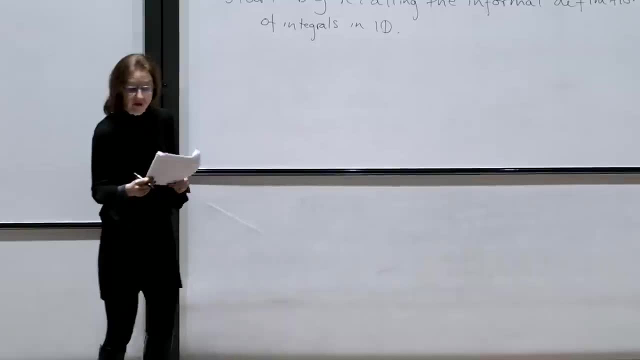 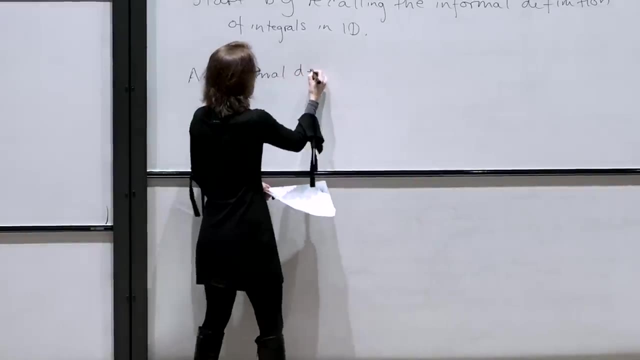 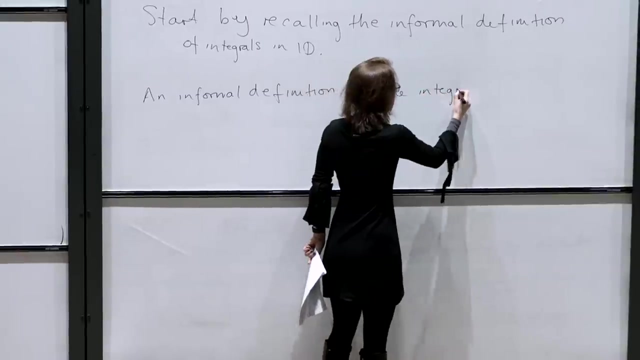 familiar to all of you, So of integrals in one dimension, Okay. so it will be very familiar to all of you. You've done plenty of examples. So an informal definition of the integral, So the integral, let's say, of some. 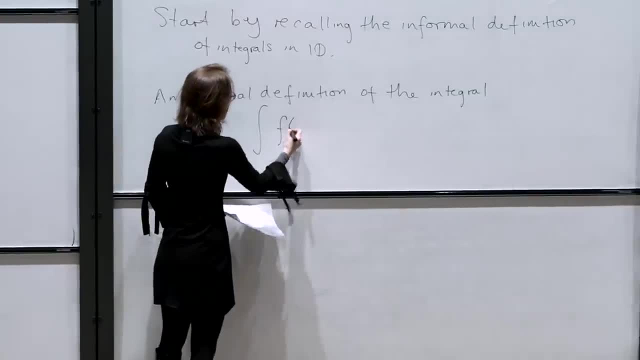 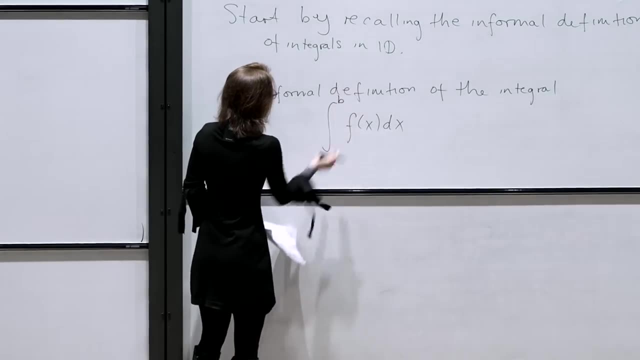 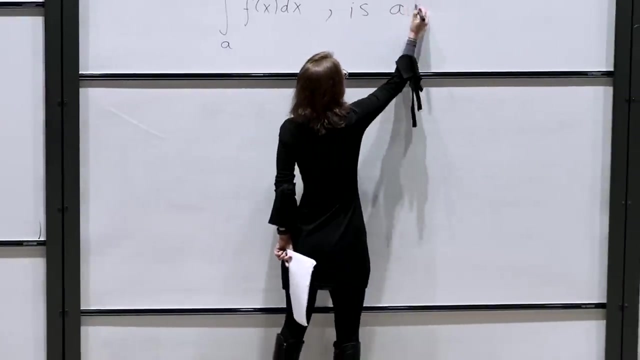 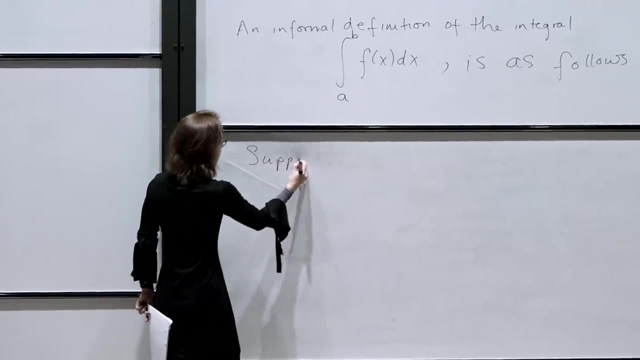 function f of x integrated with respect to x between some definite limits, So we might have x equals a and x equals b. So what do we really mean when we write that down? Well, we can think of that informally as follows: So let's suppose we have some function f which takes values on 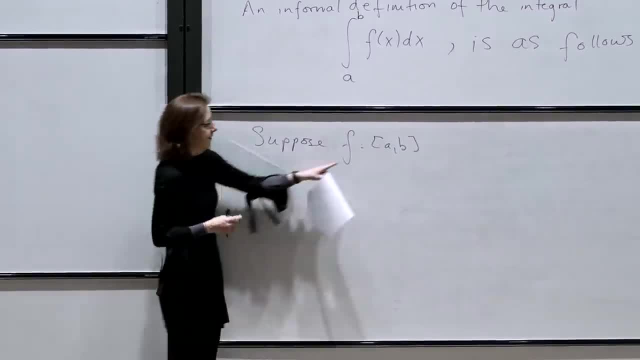 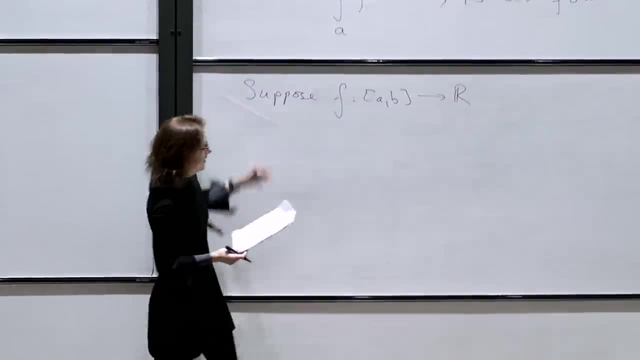 the interval a- b, So a- b. on the closed interval a- b, f takes these values and returns a real number, So a real valued function. Let's suppose that f is a function. Okay, so we can sketch f. 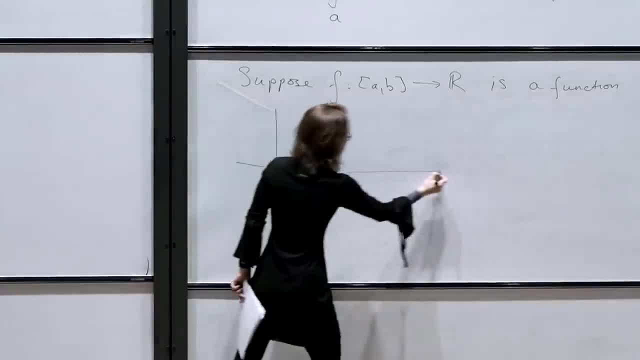 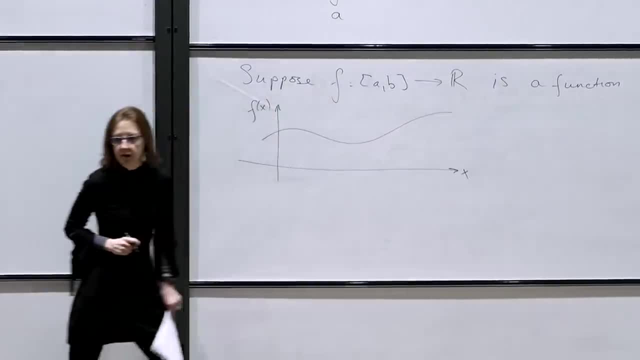 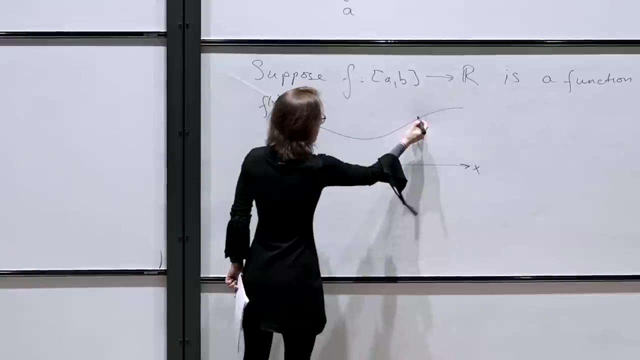 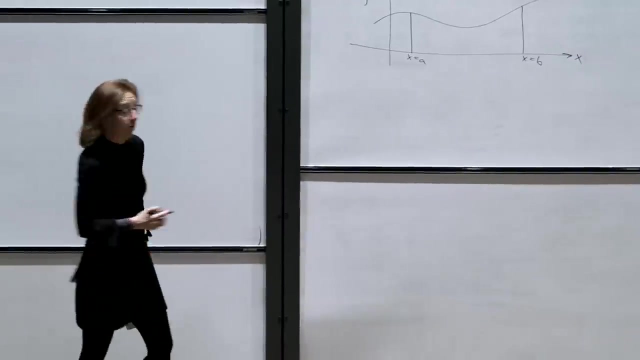 So anything you like. So we have x along here, f of x along here and we draw some function, Nice, continuous function, Okay. and then we can think about what happens when I integrate between x equals a and x equals b. So obviously, when you do that integral, what you're going to return? 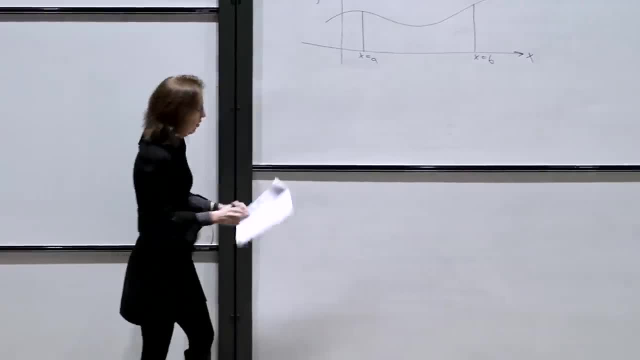 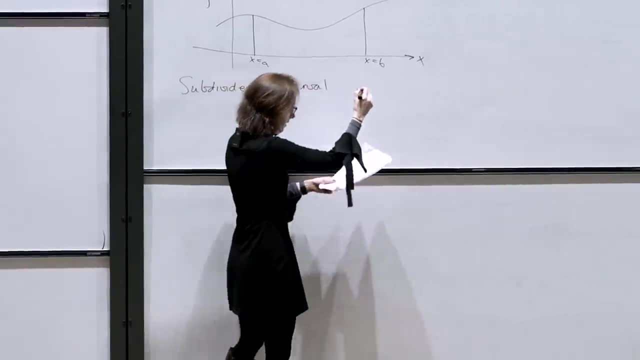 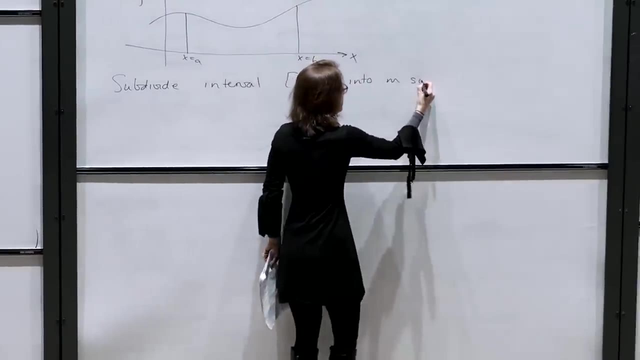 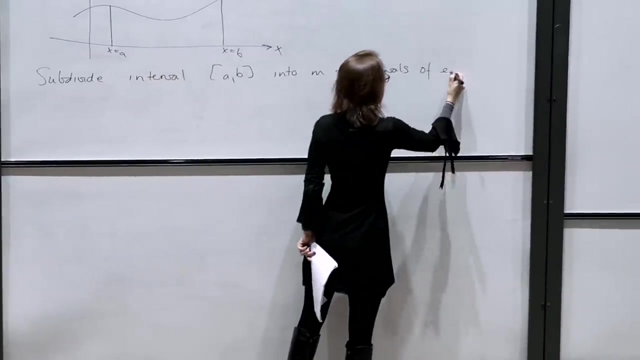 is the area under this curve. So what we do when we think about doing this is we subdivide the interval a- b into a number of subintervals, So let's say into m subintervals. We can make them equal lengths if you like. Doesn't have to be, but let's suppose we do. 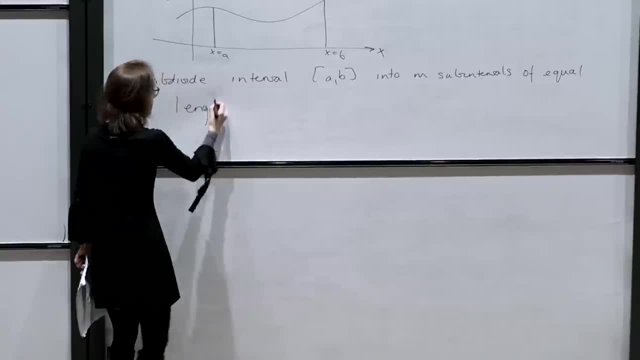 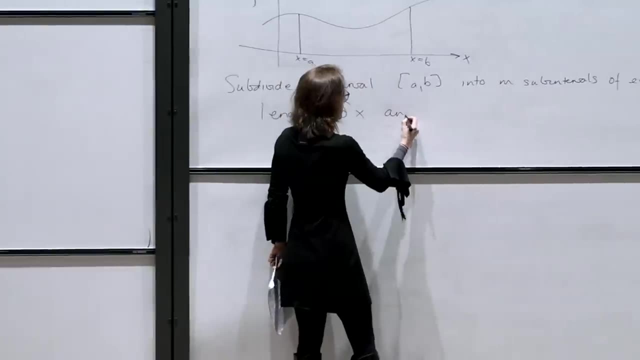 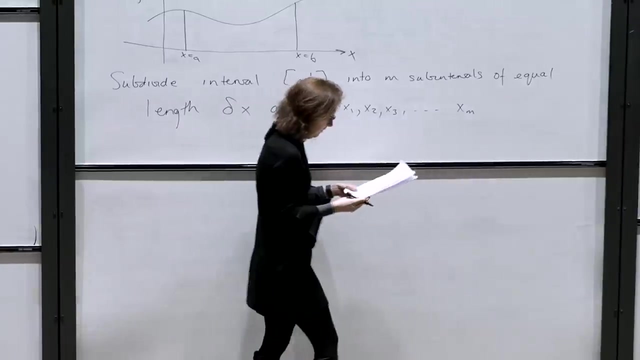 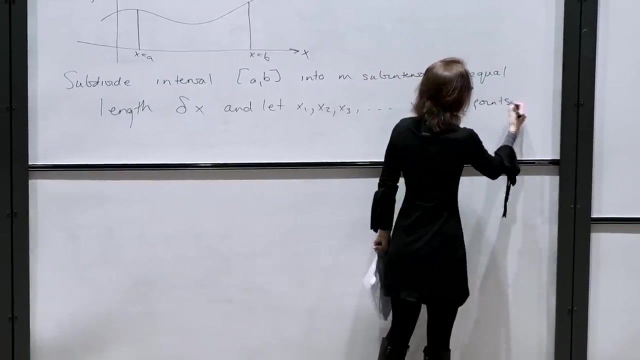 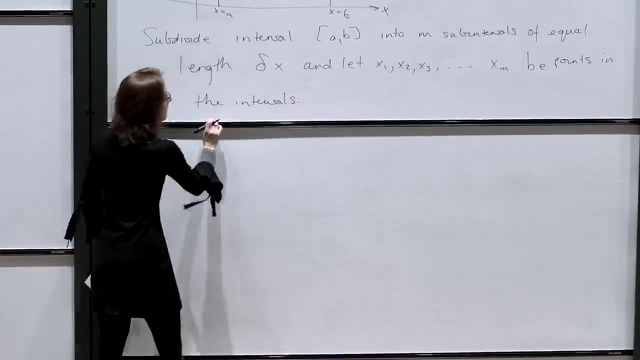 of equal length. Let's call that delta of x. So delta of x is just a small increment in x, And we let x, one, x, two, x, three, all the way up to x, m, b points in the interval. Okay, so what we do is we take our domain and we chop it up into intervals. Let's see: 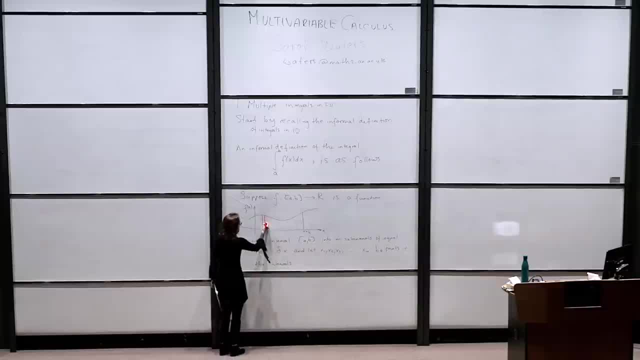 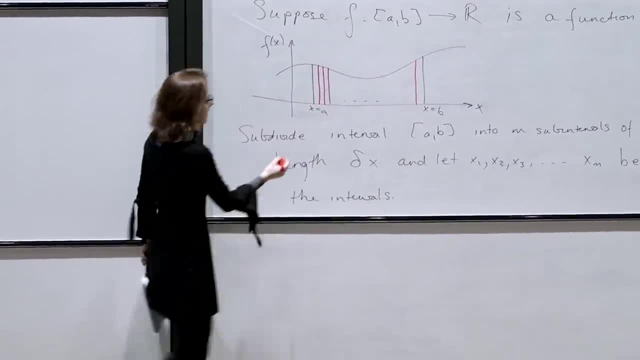 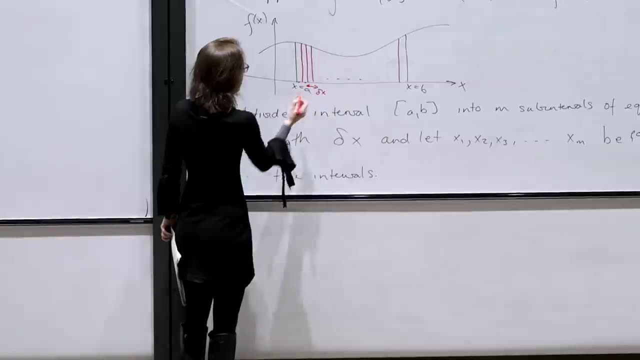 That's a nice integral, Awesome, Cool. Here we are, and so on. And we make those intervals be of some length- delta x- and within the interval we define some value of x. So in here we have x1,, in here we have x2,, etc. okay, 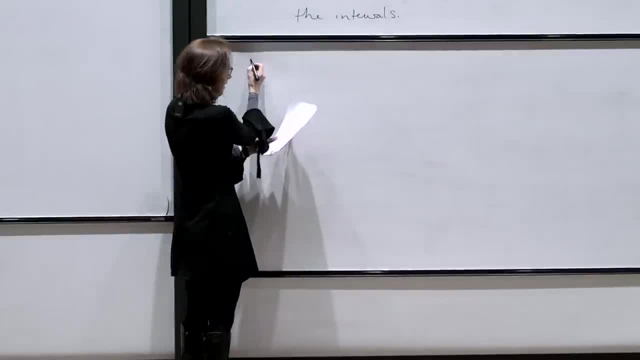 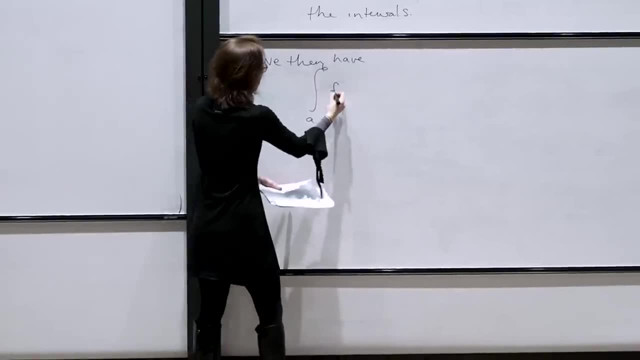 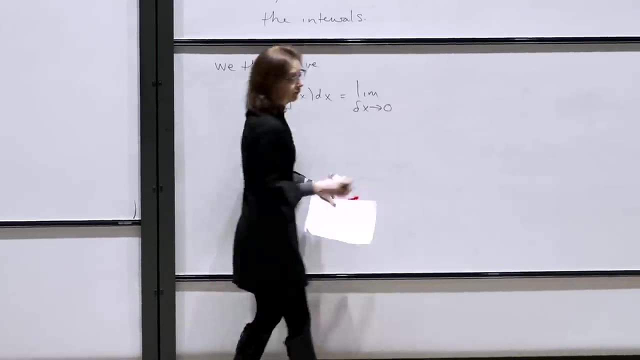 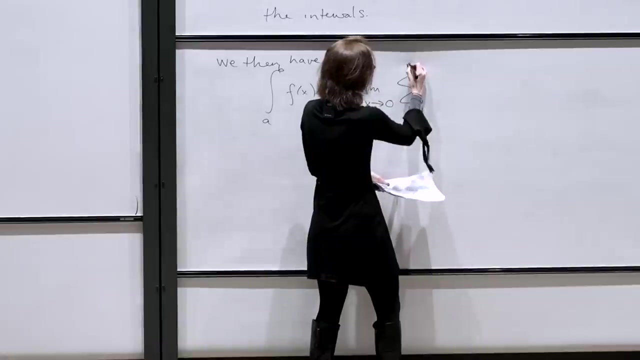 And then we can say so. we then have that the integral from a to b of f of x- dx is given by the limit, as that interval tends to zero. so it's delta x to zero of the sum of r equals 1 to m of f of xr. delta x. 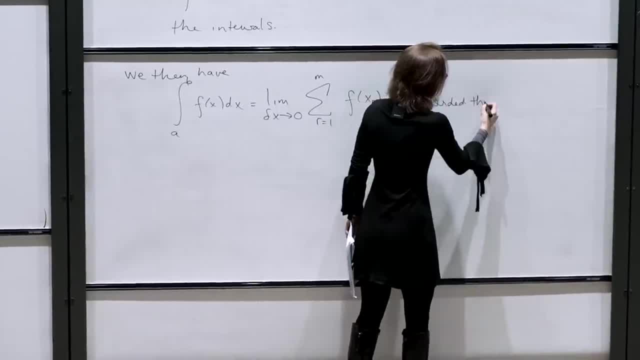 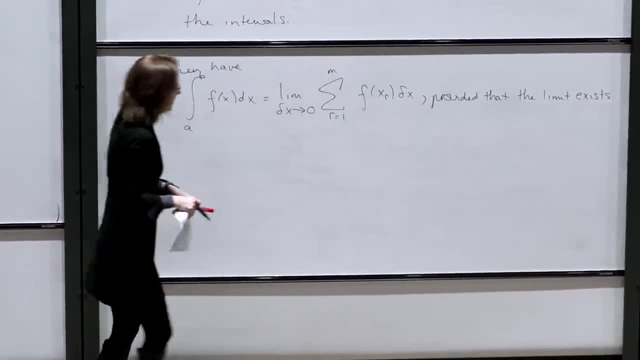 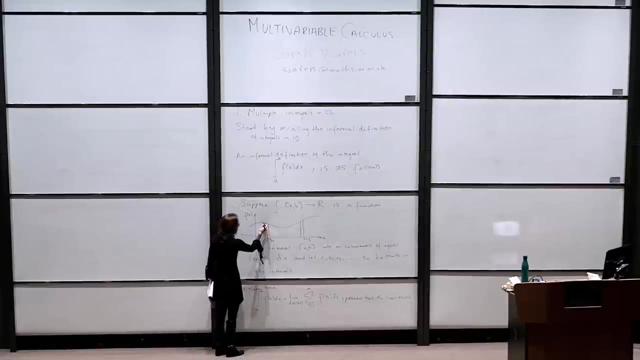 Divided, that the limit exists. So what you're really doing there is, you're saying, right, I'm going to take a whole bunch of rectangles. I'm going to do the height of the rectangle would just be the value of the function at that intermediate point in the interval which we're labeling x1,, x2,. 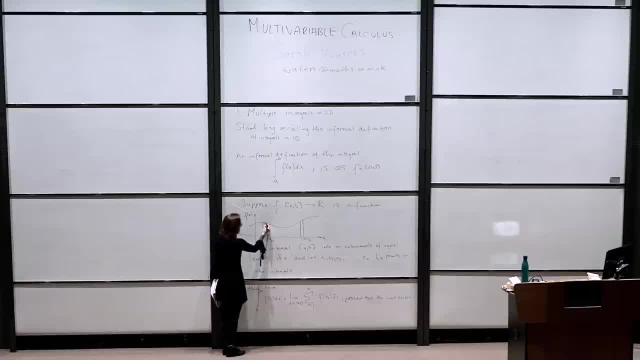 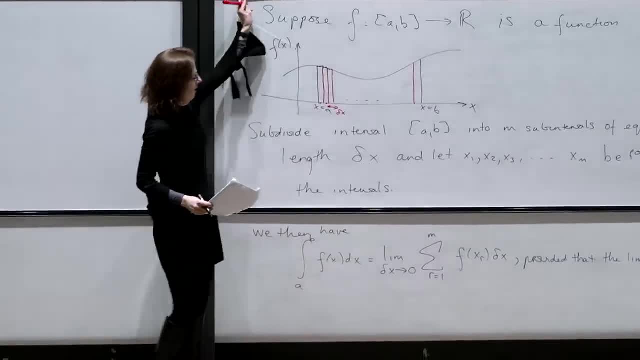 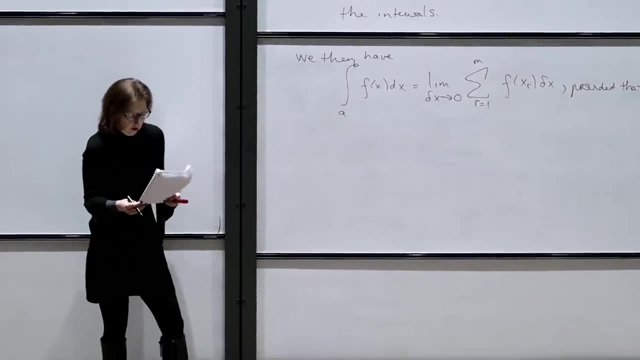 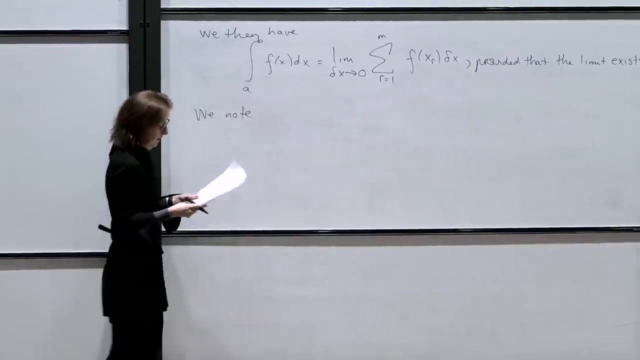 etc. and I draw those little rectangles and I sum up all those rectangles. Take the limit, as delta x tends to zero and that gives me the integral of the function between a and b, provided that that limit exists. So that will always be the case, that the limit will exist provided f is continuous. 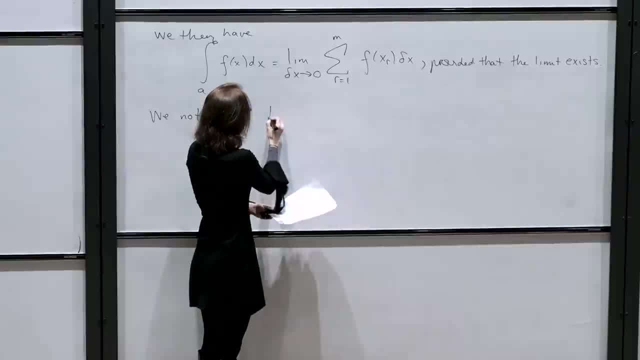 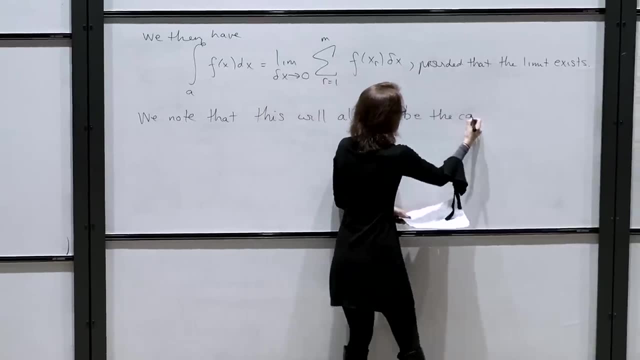 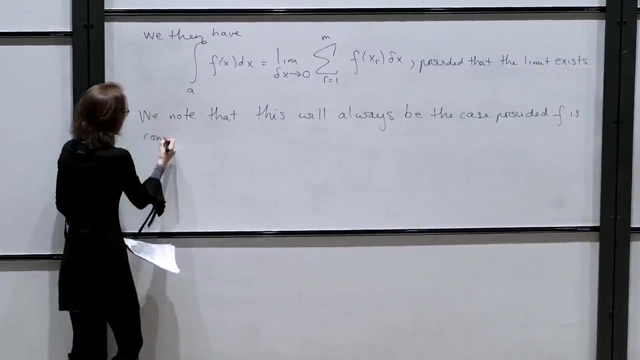 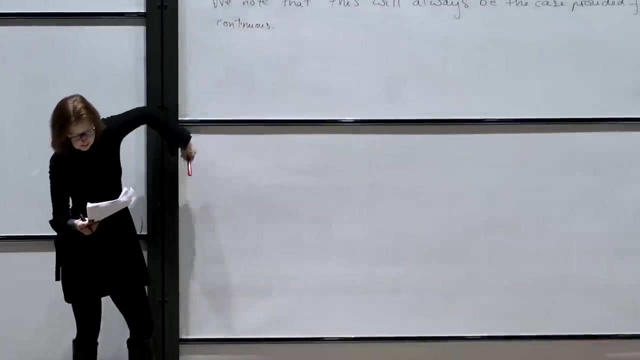 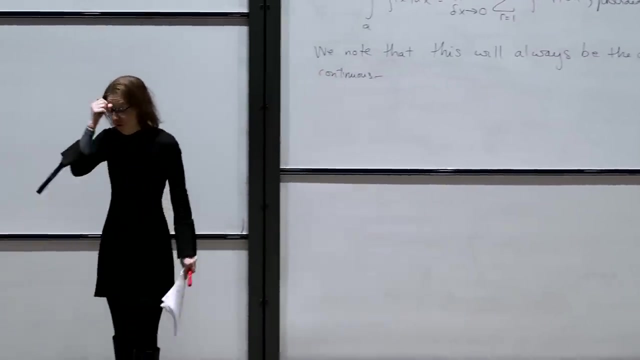 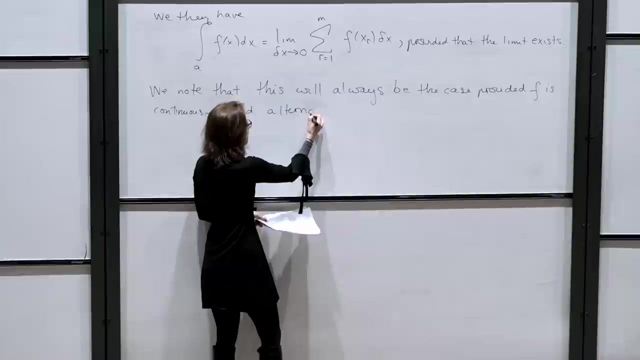 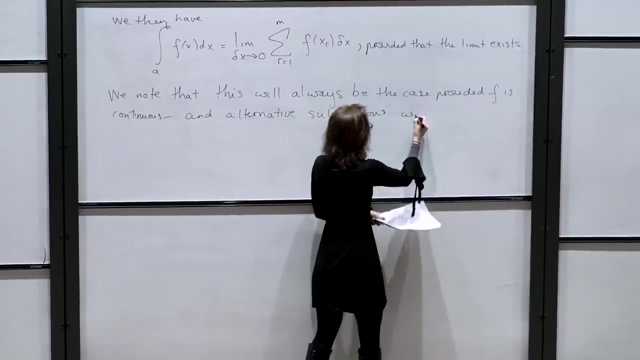 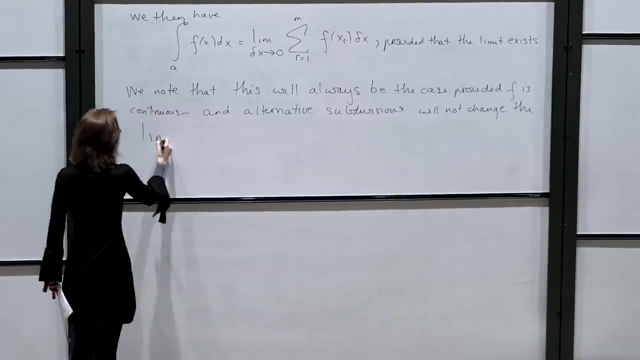 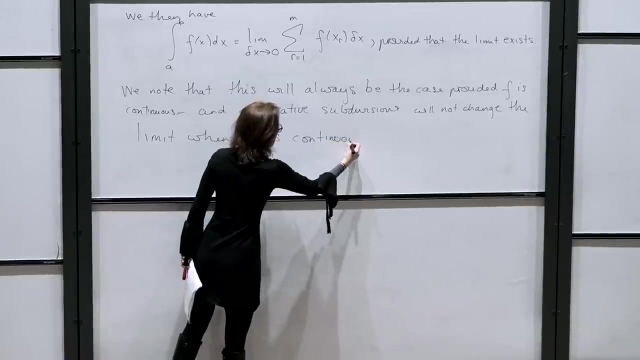 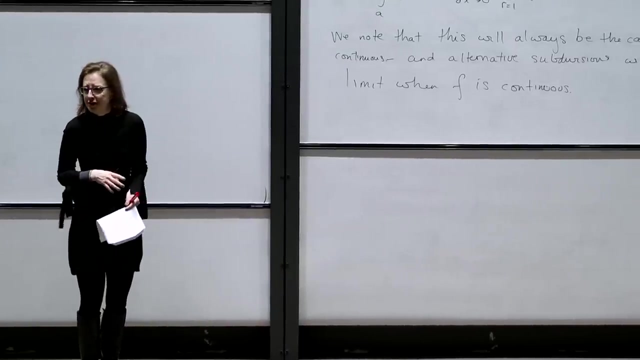 So this will always be the case, Okay, Okay, rodz, mw w w Fund Do f N, N, b h N, it 0, a, f, n, f, r, 1 mw will not change the limit when f is continuous. All right, so that's all very straightforward. You've all seen that, And the reason I wanted 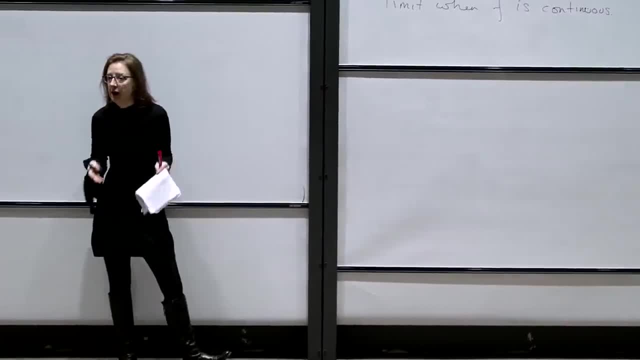 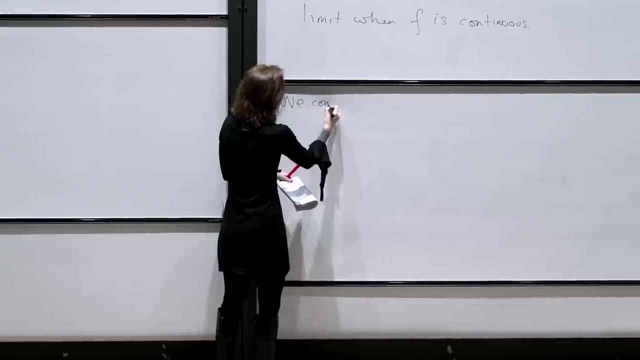 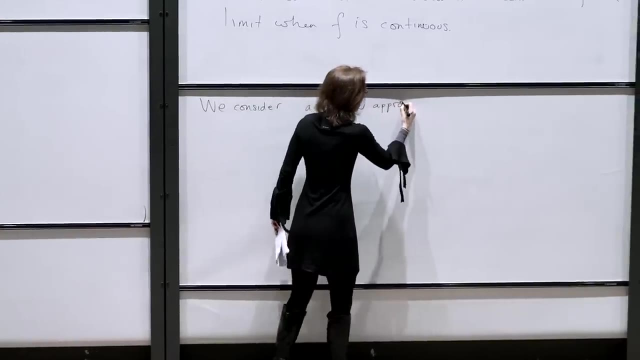 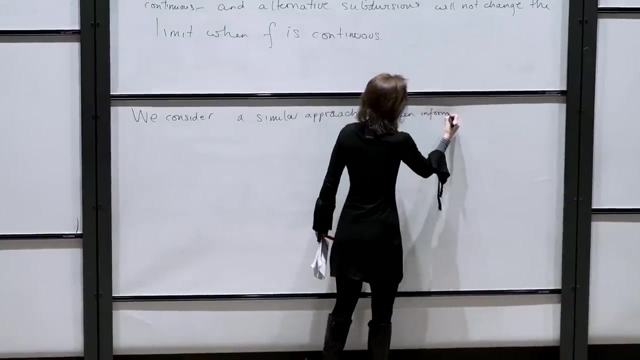 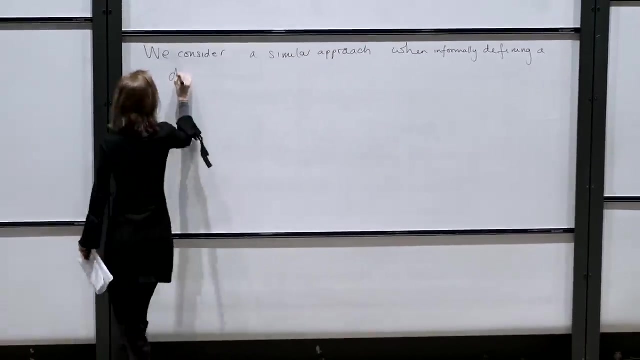 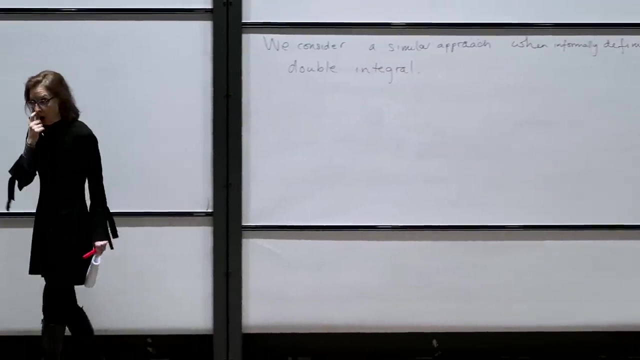 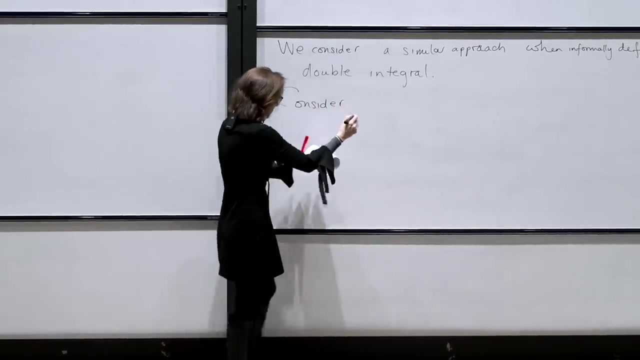 to just briefly go over. it is because we extend those ideas when we're thinking of integrals in higher dimensions. So now we're going to consider this in two dimensions, So we consider a similar approach when informally defining a double integral. Okay, so let's think about what we're doing now. So let's suppose we consider a region of the plane. 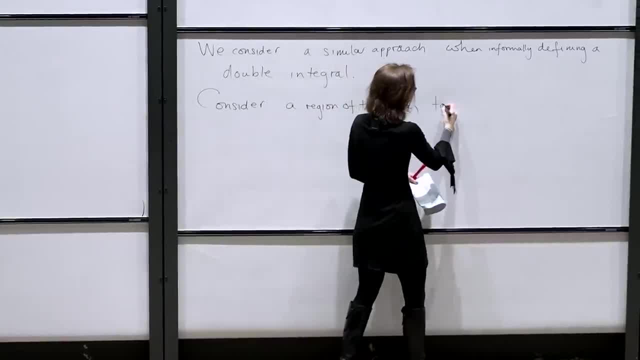 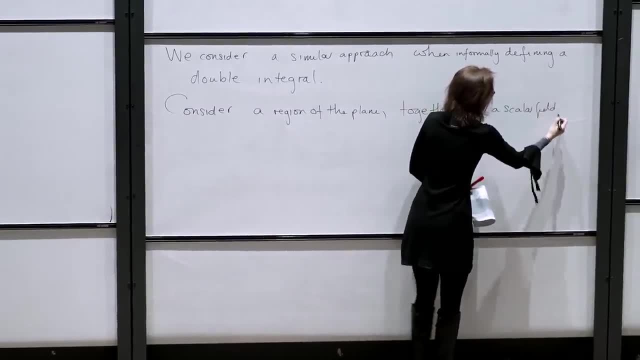 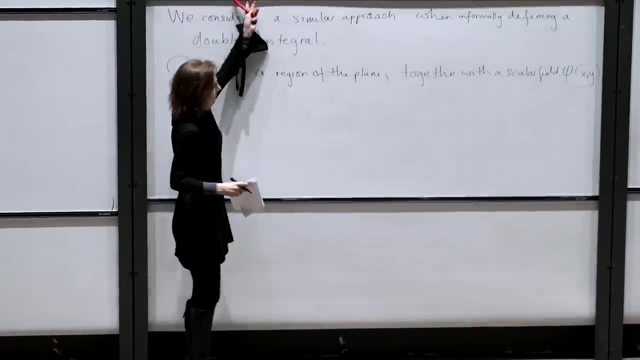 together with some function, So together with a scalar field now, which we're going to call psi, which will be a function of the coordinates in the plane: x, y. Okay, so we're going to have the plane: Here's x, here's y. 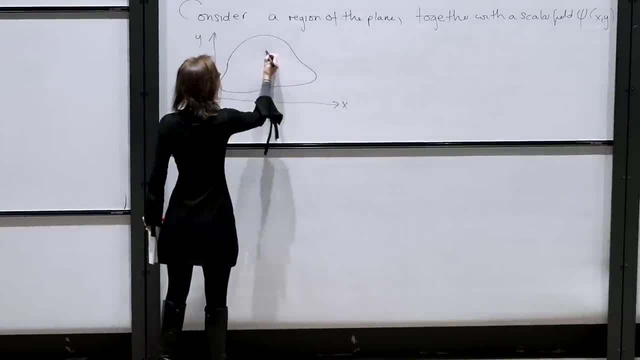 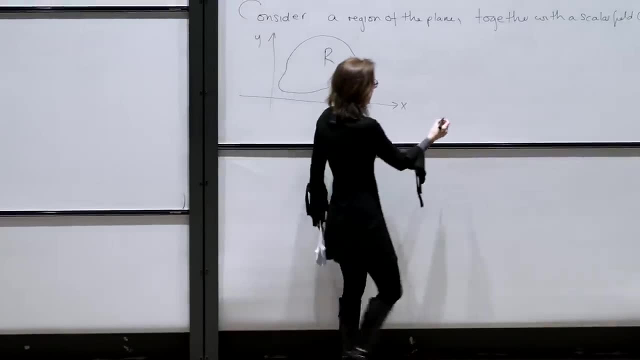 And we're going to integrate over some region in the plane which we're going to call R, our region of interest, R. So if I'm thinking of this in terms of its sort of physical interpretation, so if I have x and y now, 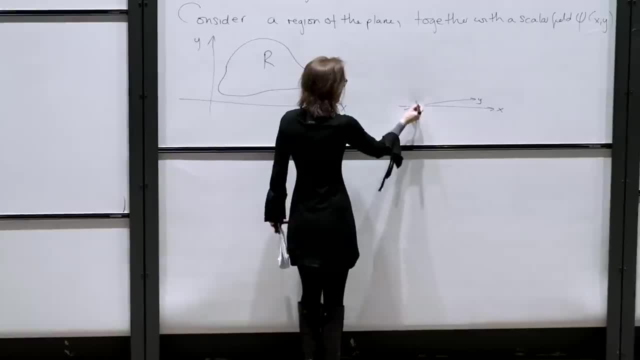 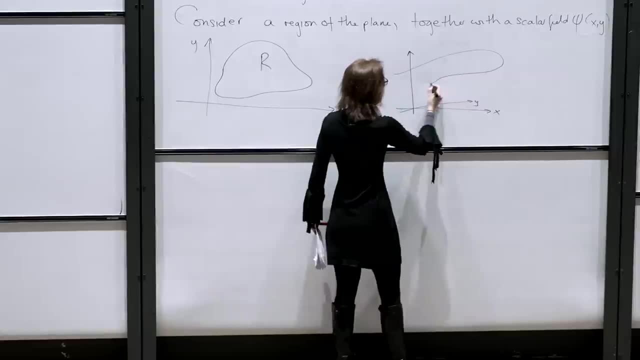 in the plane and I have my third dimension coming up here. then psi is some scalar field, it's a surface. So here's where I challenge my ability to draw but something like that. Let's suppose that's psi And what I want to do is integrate that function. 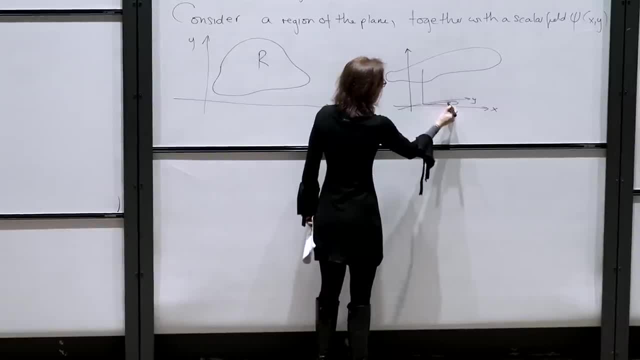 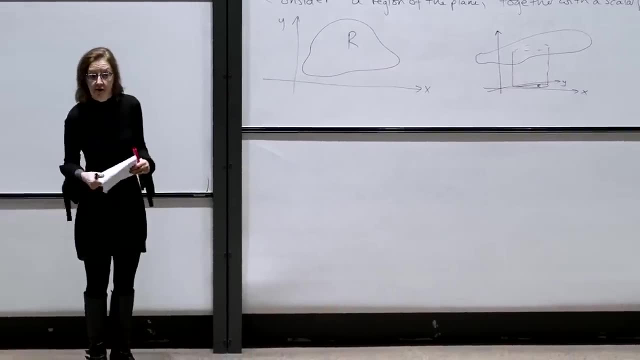 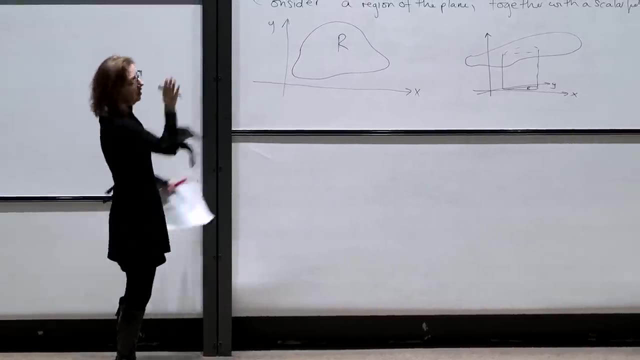 over some region in the plane. So here's my R, and I want to integrate that function over that region. So what I'm doing now is computing the volume underneath that surface. Okay, So we do exactly the same thing. So this time, instead of partitioning- 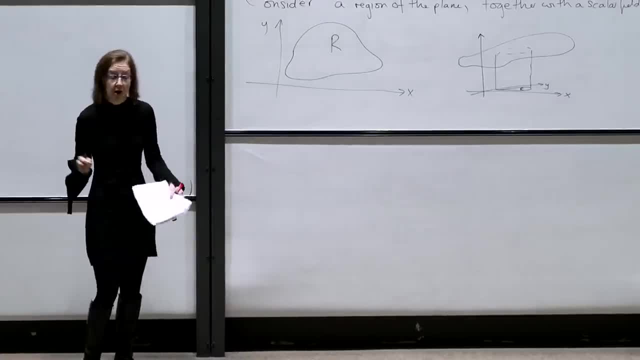 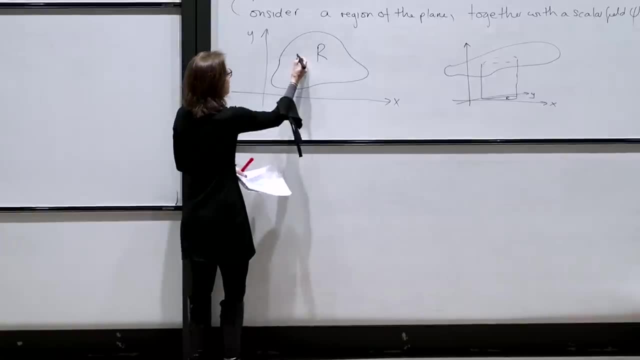 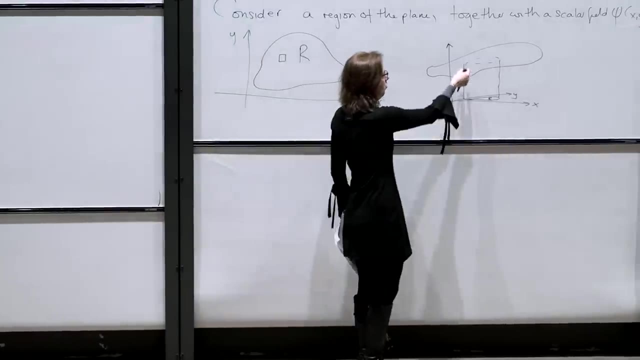 the line into small intervals of width. delta x. we partition the plane into small elements of a given area. So we can think about dividing this up into regions and then summing, playing the same trick: summing all the volumes that are given between the surface. 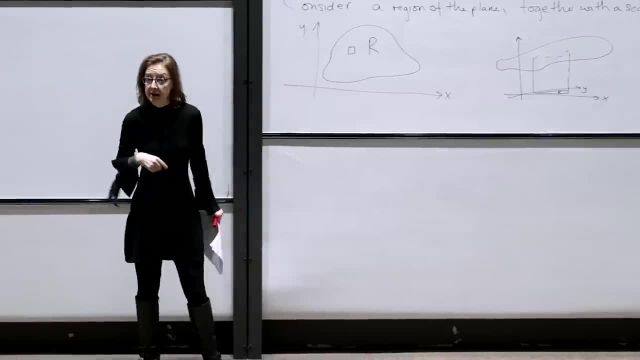 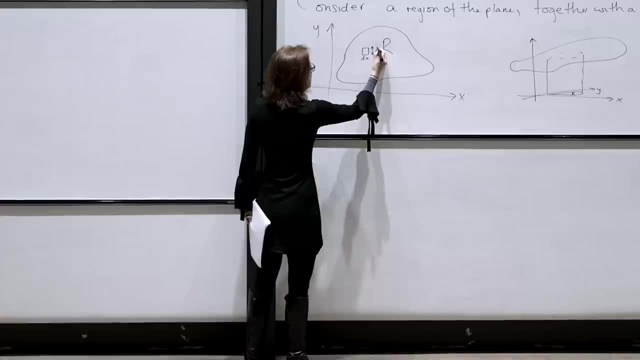 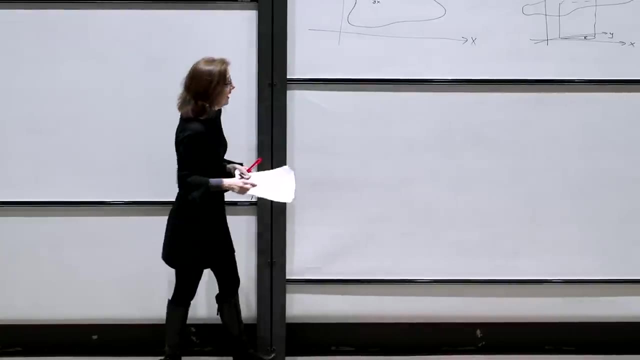 over that small element in the plane. sum them all up, take the limit and that will give me the double integral in this case. So we might suppose this has width delta x and height delta y, And we can say again: we need to define some value of the scalar field. So let's suppose 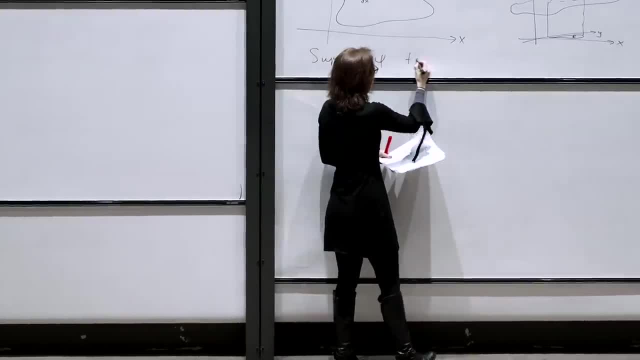 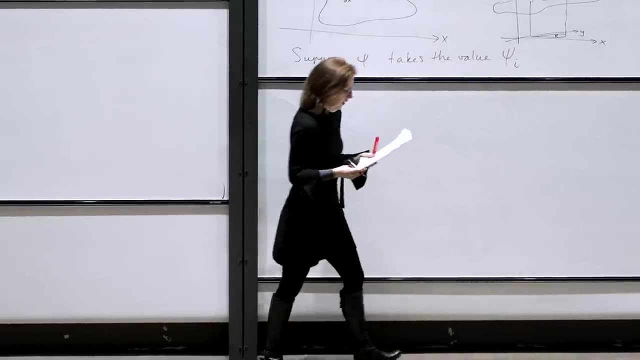 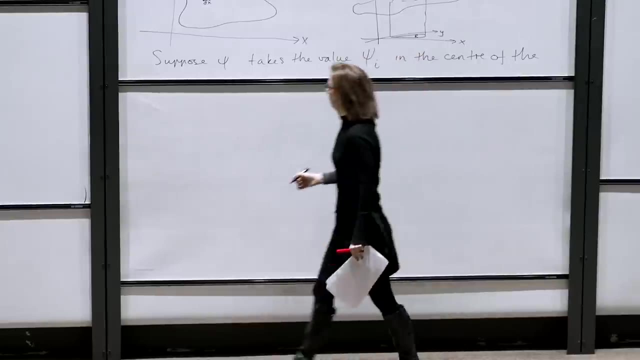 the scalar field, psi takes the value and we're going to call it psi with a subscript i in the centre. So I'm going to say psi with a subscript i. So I'm going to say psi with a subscript i in the centre. 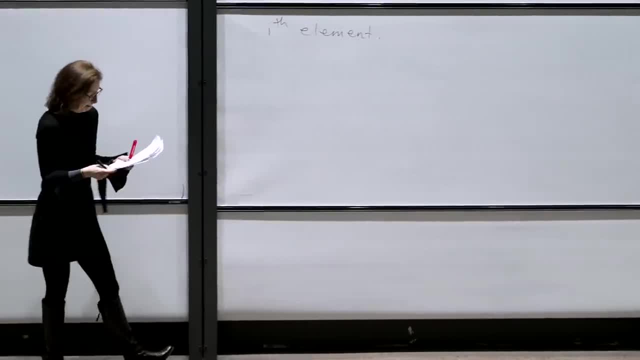 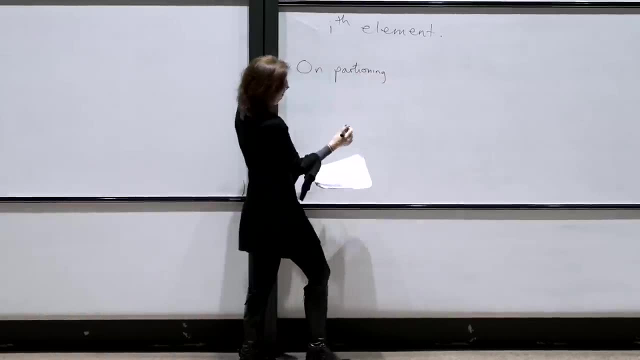 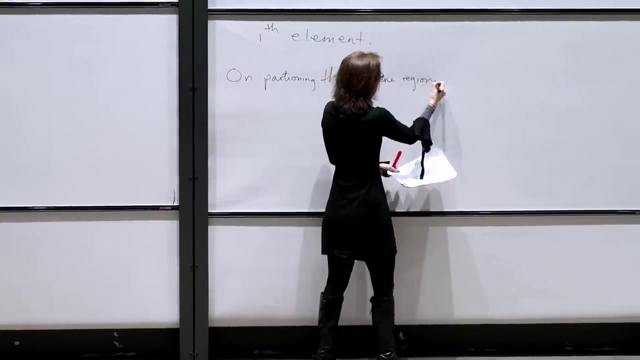 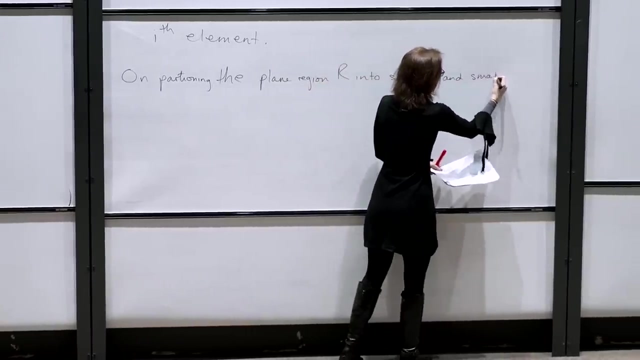 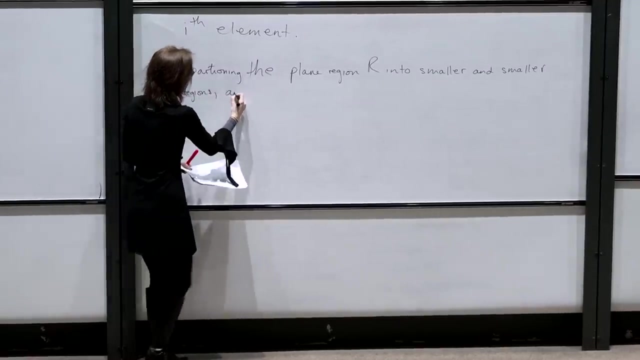 So I'm going to say psi with a subscript i And this is going to be the value of the element. So we can take a small element of the ice element, Plane region R, into smaller and smaller subregions And then taking the limit, this time as the region, the area of that region tends to zero. 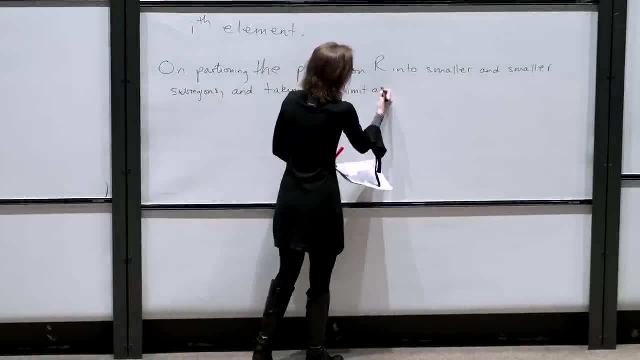 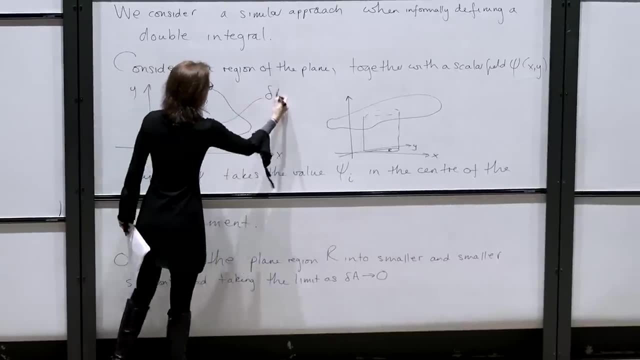 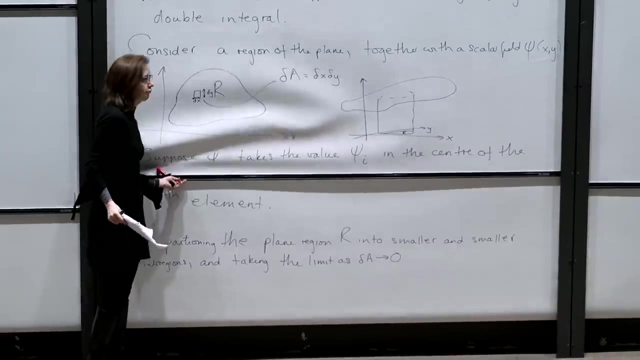 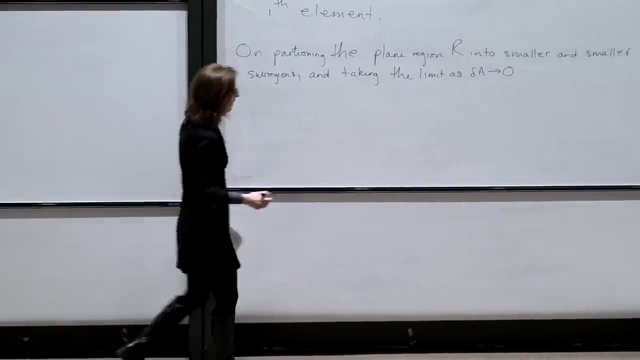 so taking the limit as delta A tends to zero, so I should have said it up here, but I'm going to define delta A to be delta X, delta Y. It's just the area of that little region of width- delta X, and height, delta Y. 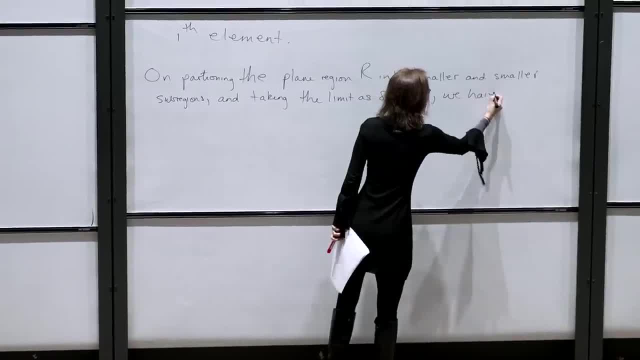 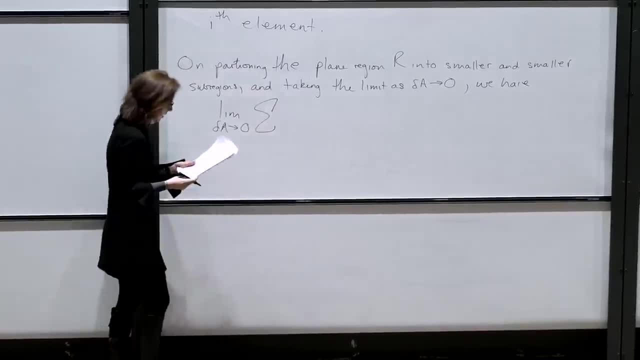 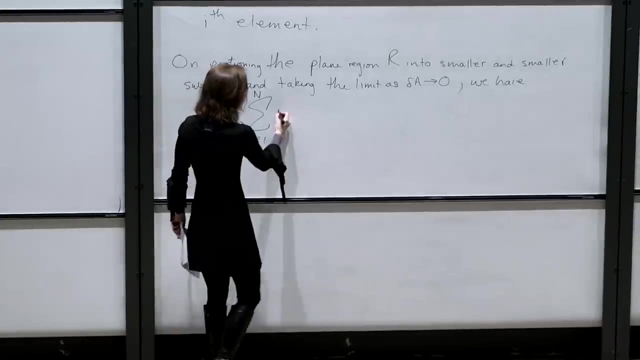 So then we can define the double integral. So we have that the limit As delta A tends to zero of the sum. So now I sum over. let's suppose there are N subregions, So I sum from: I equals one to N the value of this scalar field at the centre of the. 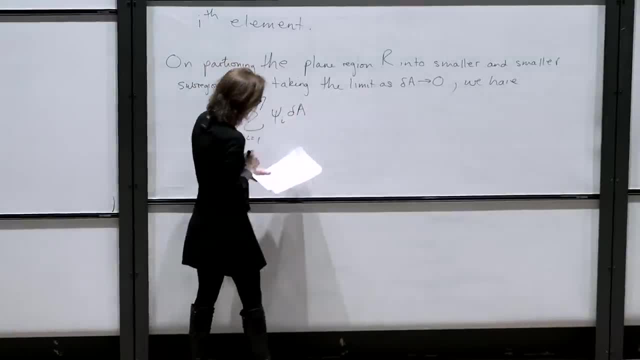 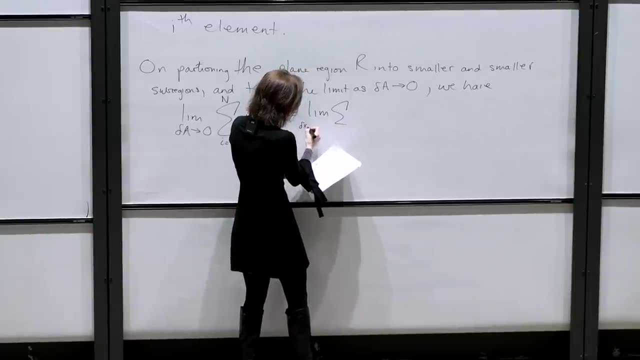 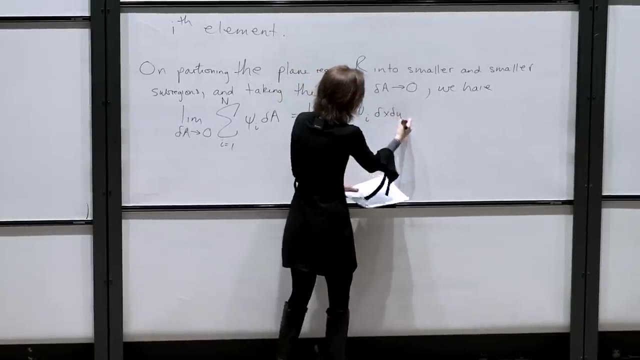 subregion times. delta A, which is the same as saying the limit, as delta X, delta Y tends to zero. I equals one to N, So I add up the sum of the sum, I get a negative. I can't get this. I just can't. 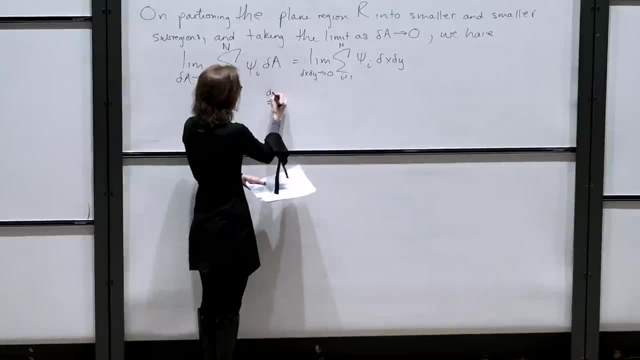 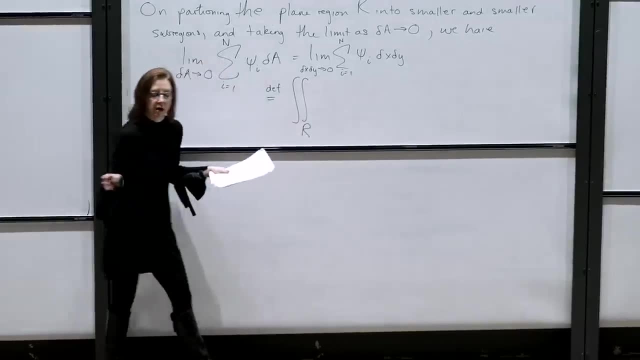 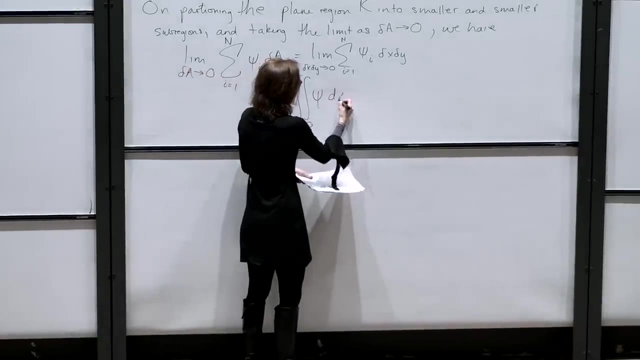 So this is the integral of the region of psi I, delta X, delta Y, And we define that to be So. this is definition, The integral over the region R. And to denote the fact we're integrating over an area, not over a single line or single variable, we use a double integral of psi, dx, dy. 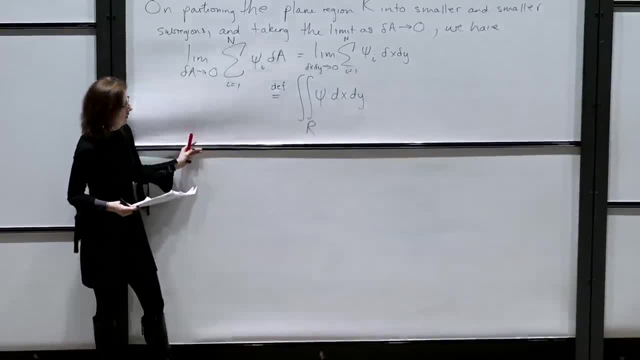 And in the last course- you did last time- you did a double integral of psi dx dy. And in the last course- you did last time- you did a double integral of psi dy- dx dy, last term in introductory calculus. you've computed a lot of these double. 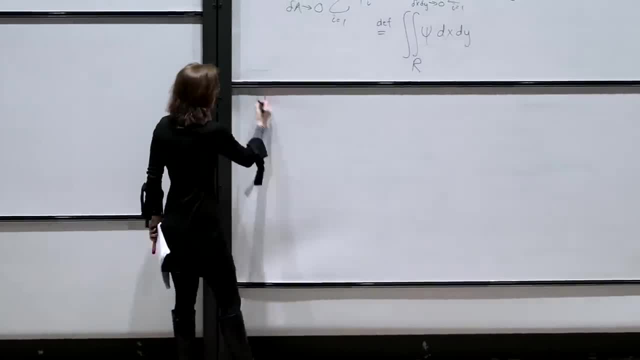 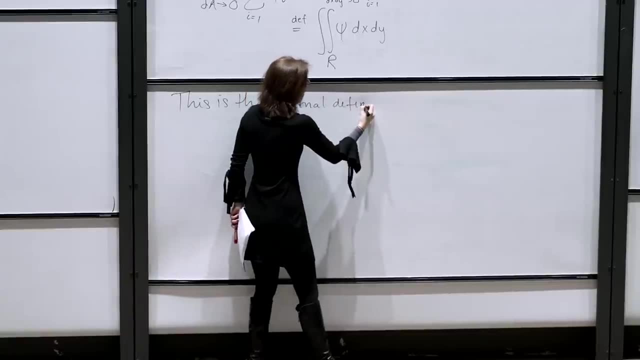 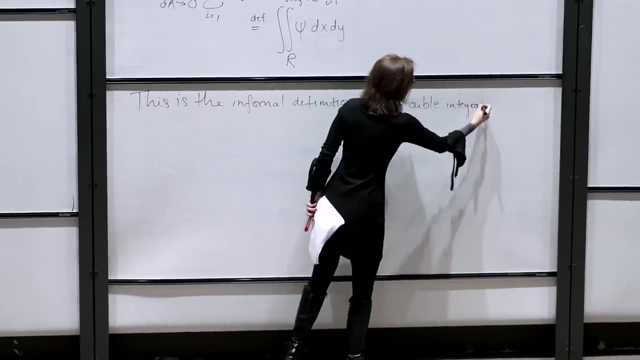 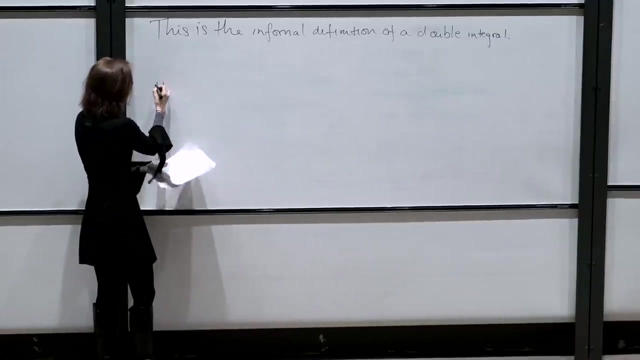 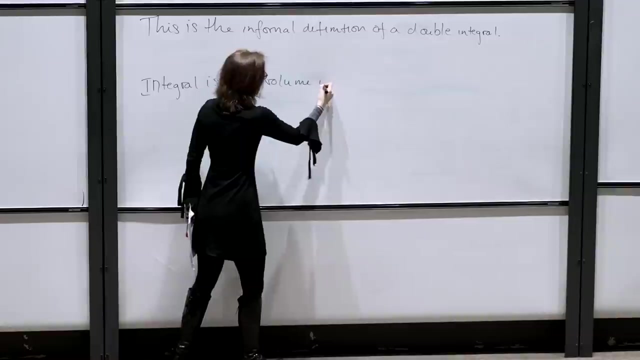 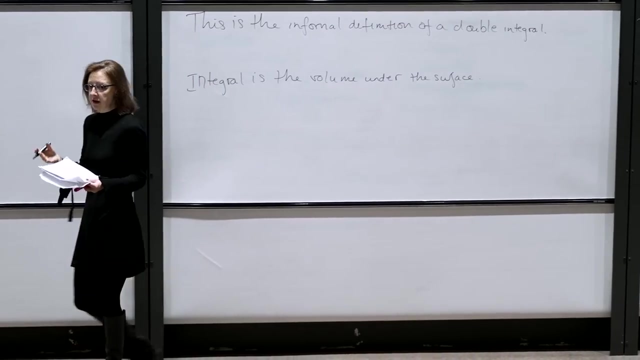 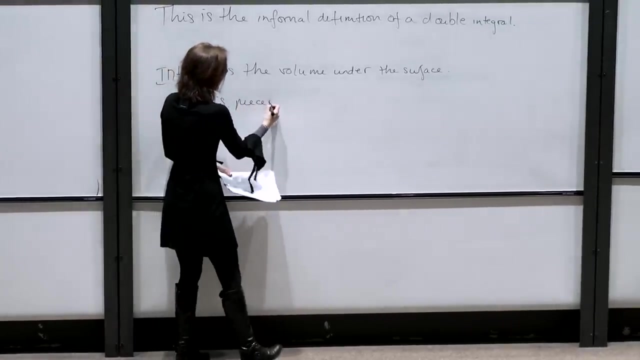 integrals. So this is the informal definition of a double integral, and it represents the volume and the integral is the volume under the surface. So again we have all the usual things: we want to make sure that the limit exists, and it turns out that if psi is piecewise continuous, 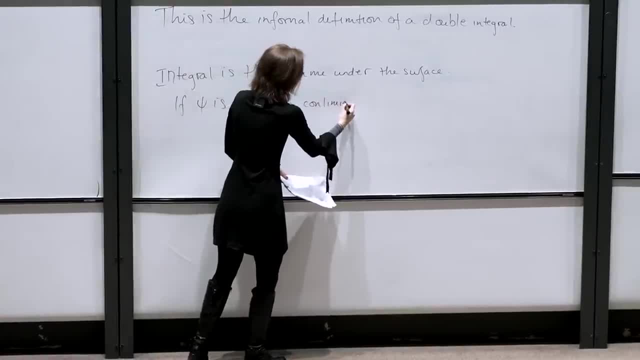 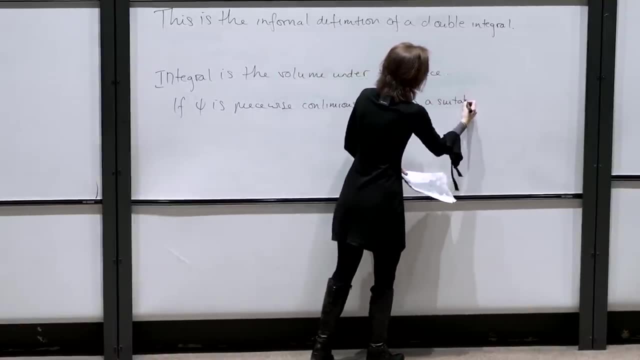 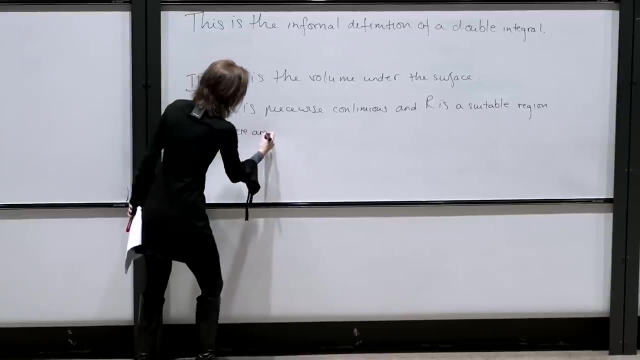 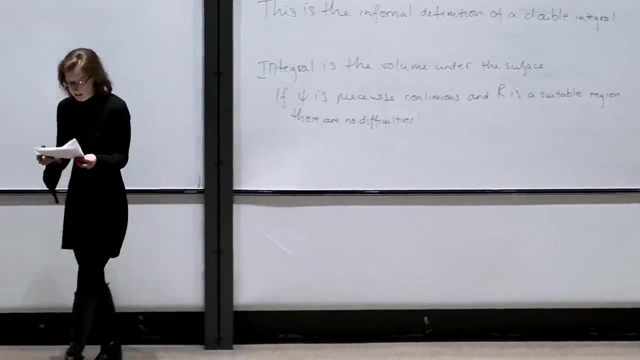 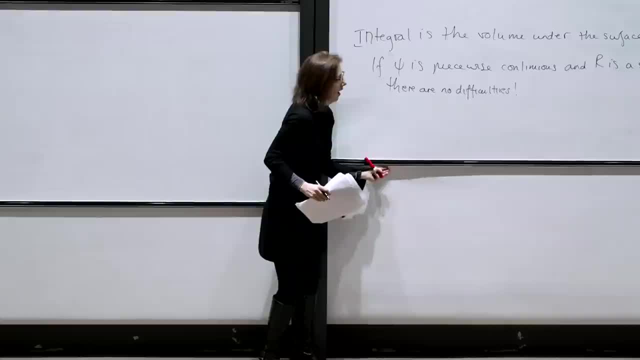 how to calculate a double integral. So that's a whistle stop through how we think about double integrals and how they connect single integrals, and it's going to be the focus of our lectures in the coming weeks. So these double integrals have a number of properties. 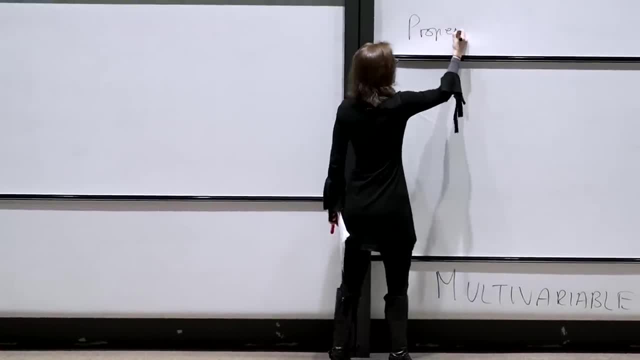 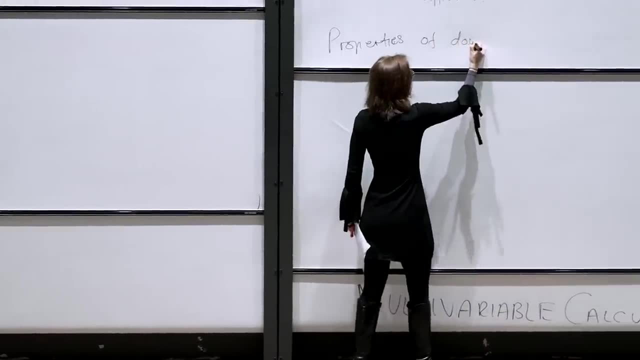 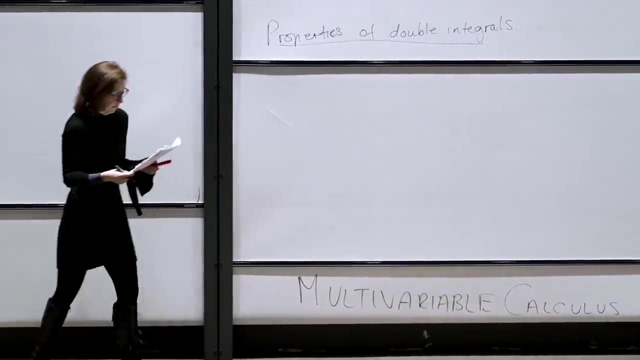 which are useful to note and exploit, and there's even more in the online lecture notes that you want to take a look at. So the following two articles are the text of the lecture you've just a look at and the text of the lecture you'll need to take a look at. 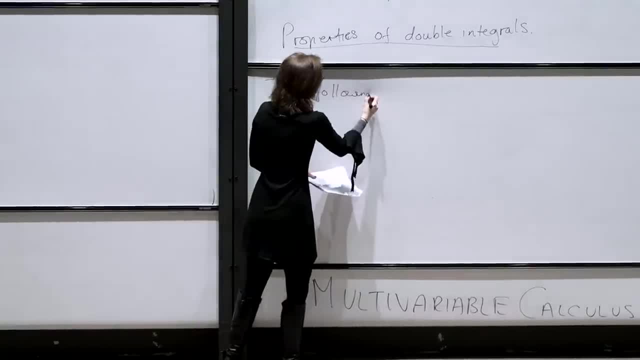 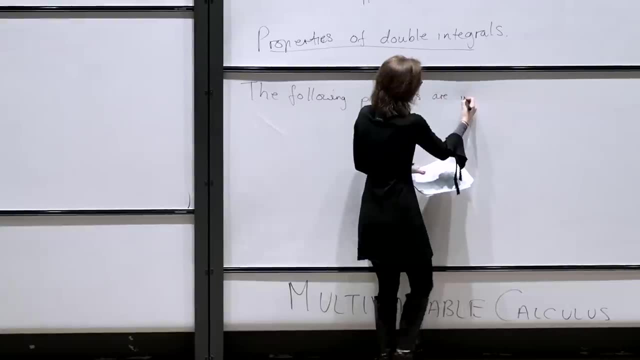 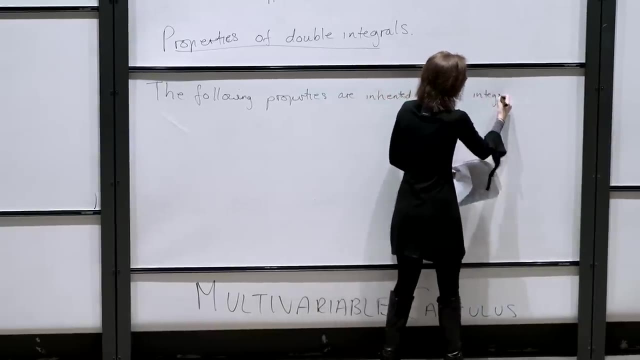 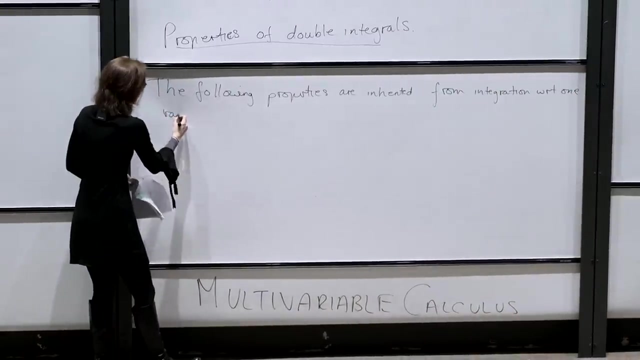 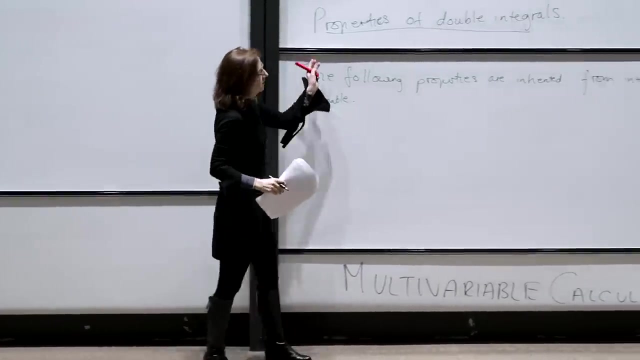 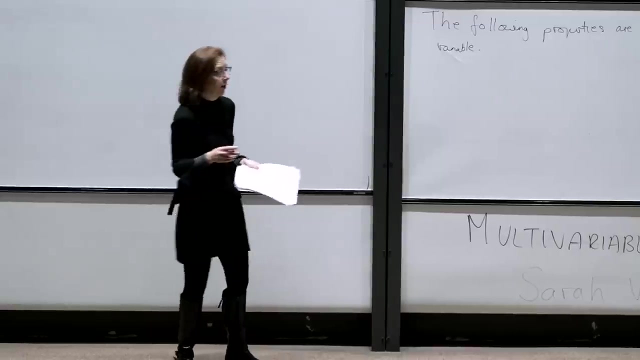 properties are inherited from integration with respect to one variable. So the properties I'm going to write down are often useful when you're trying to think about careful and more straightforward ways to compute double integrals. So we're going to see examples where it doesn't matter which way I integrate, whether I integrate 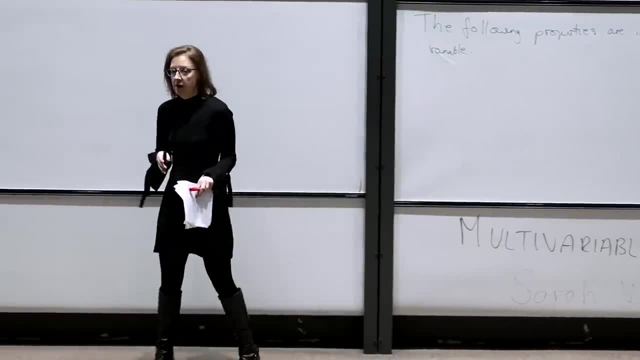 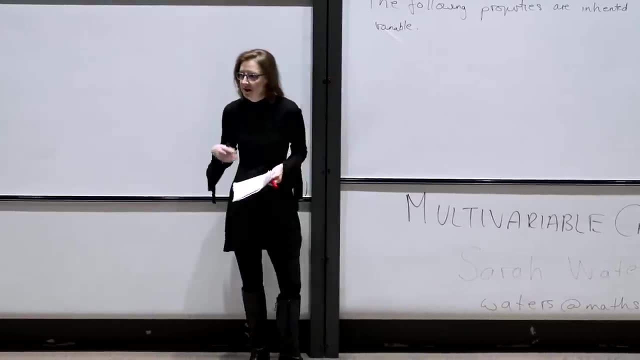 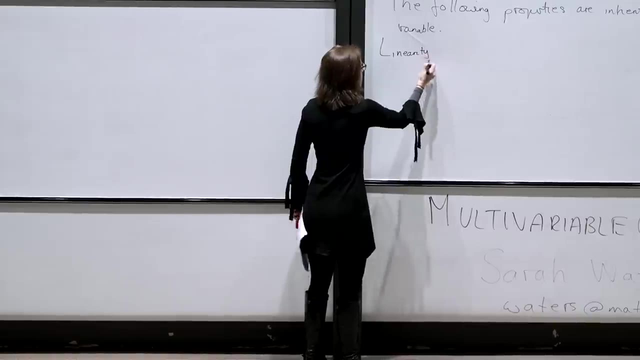 first with respect to x, or then with respect to y, or vice versa. but some methods are more advantageous and mean you have to do less work, And these properties can also be exploited to allow you to essentially do less work. So we're going to think about sensible ways to compute these integrals, exploiting various 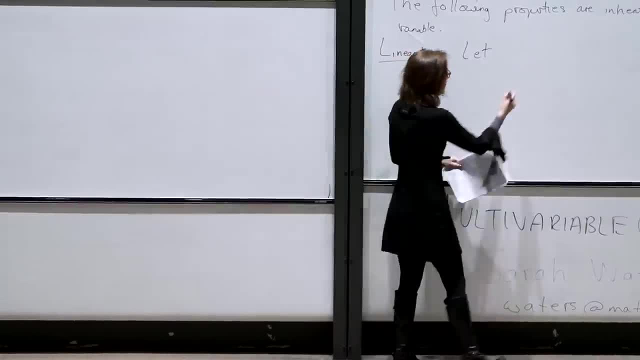 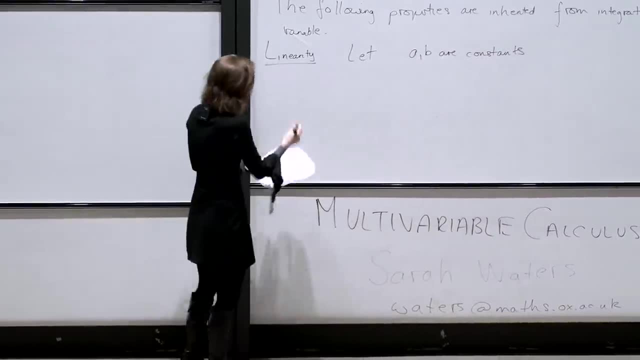 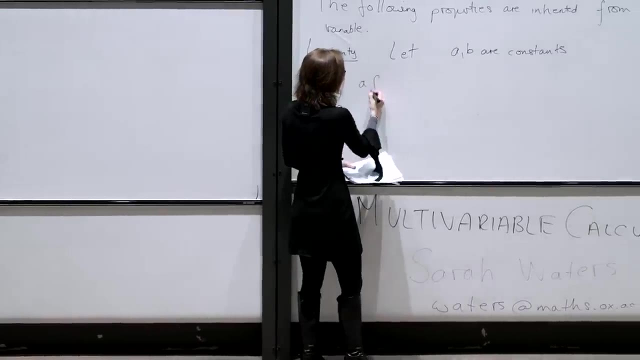 properties. So let's start with the property of linearity. So let's Suppose a and b are just constants, so then we have that, the integral over r, so some suitable domain in the plane of a times some function of f, of x and y, plus b times a function. 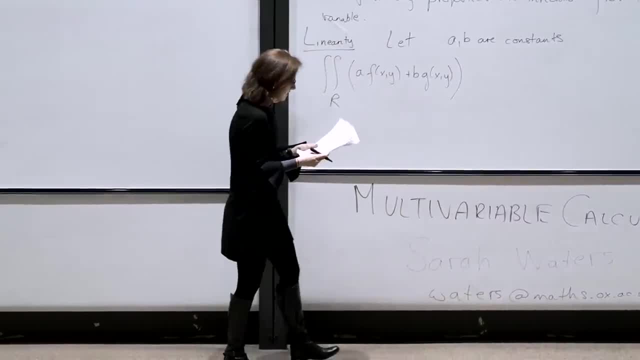 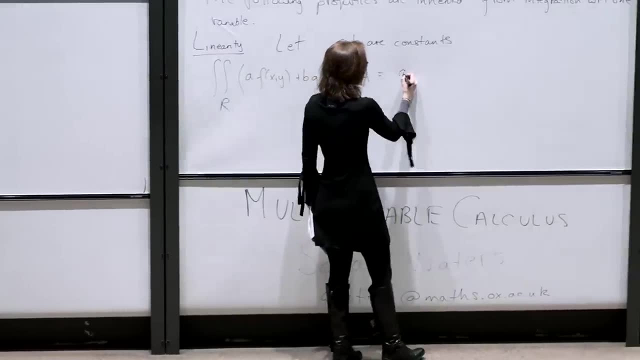 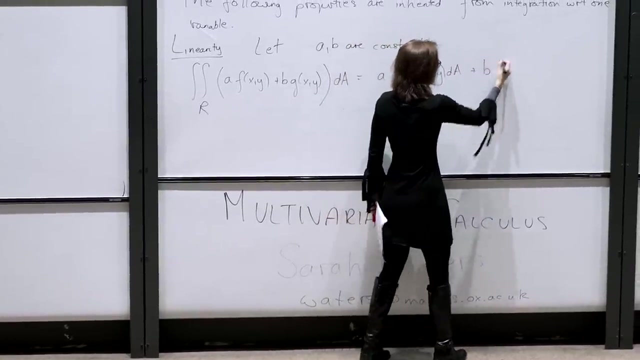 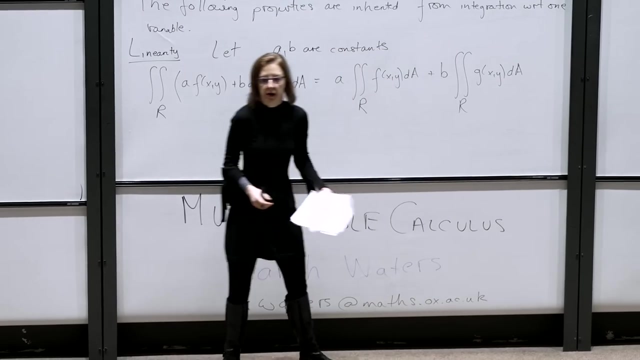 g of x and y all integrated over the plane dA over the region of interest. well, that's just the same as. So we have a times integral of f over the region plus b times the integral of g over the region, exactly as you would have seen in integration of one variable. 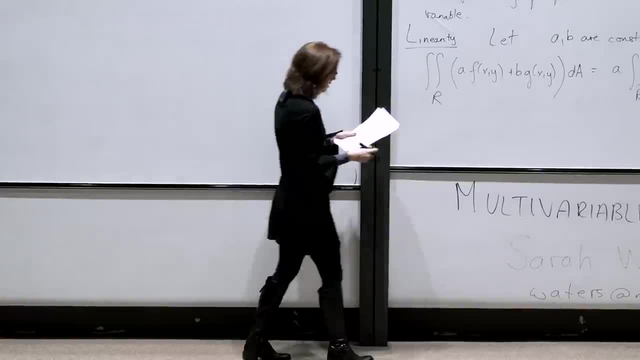 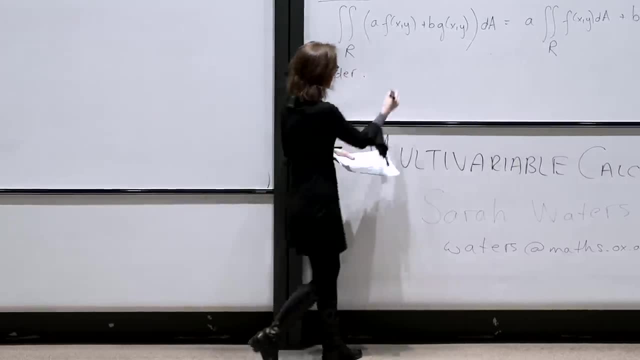 So then we have the property of order. So if we have that a function f of x and y is alreadyustomer, we can simply write this and we will have to integrate it. So if we have that a function f of x and y is alreadyestimated, then we can use the. 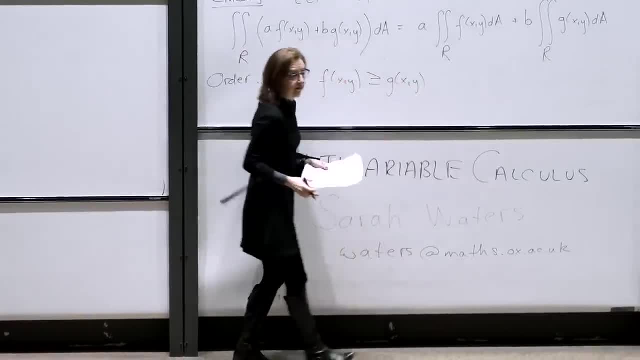 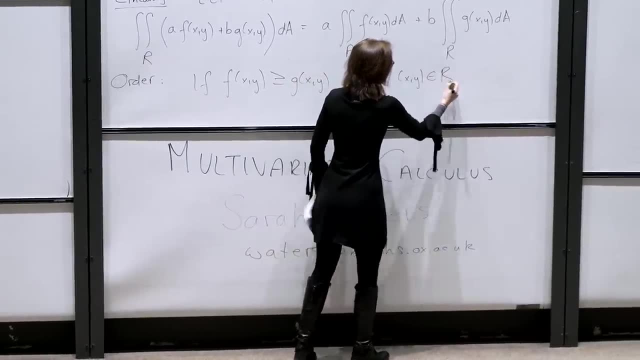 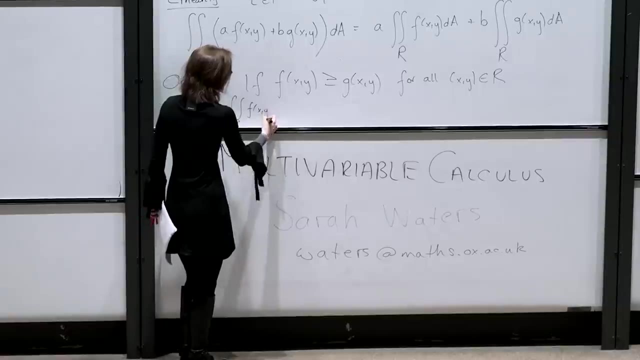 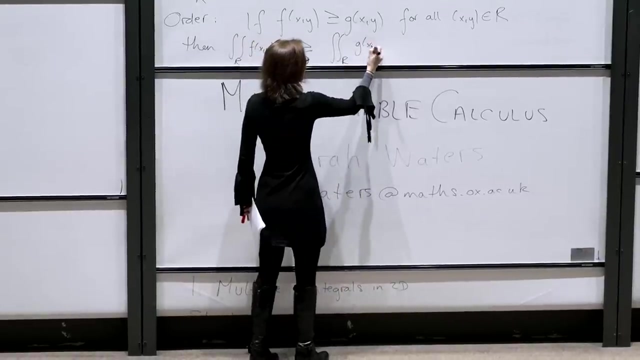 always greater than or equal to a function g of x and y on the region of interest. so for all x and y in R, then we will have that the integral over the region of f of x, y, dA will always be greater than or equal to the integral over R of g of x and y dA. 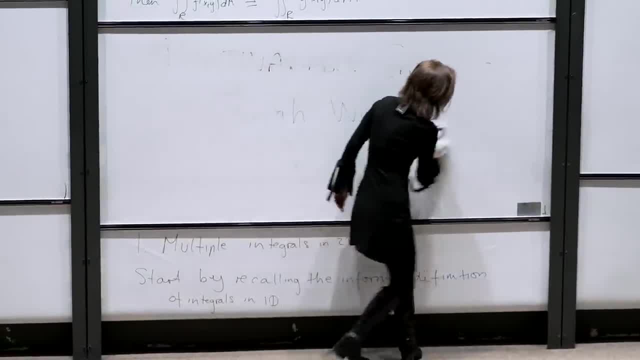 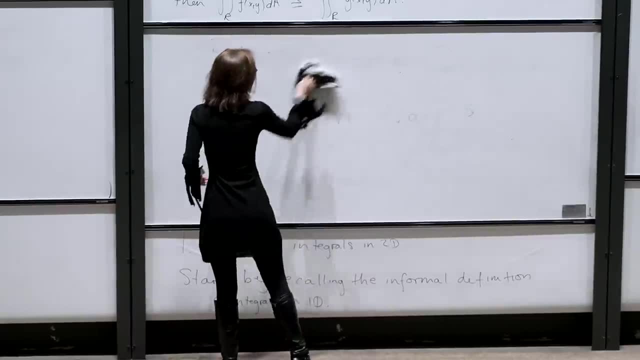 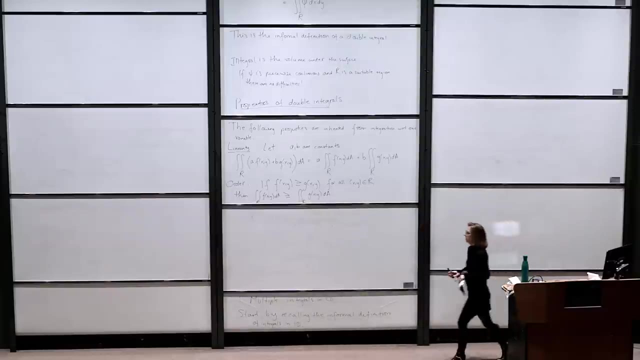 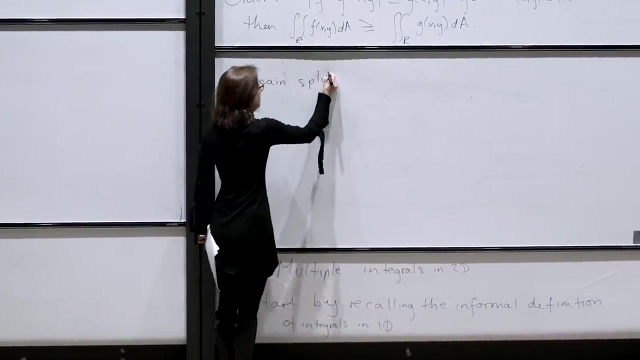 All right, and the last one I'm going to write down is the property of domain splitting, which is that sometimes you can exploit the fact it's sensible to split the domain up to make your life easier. So let's suppose that the region of interest is greater than or equal to the integral over R of x, y, dA. 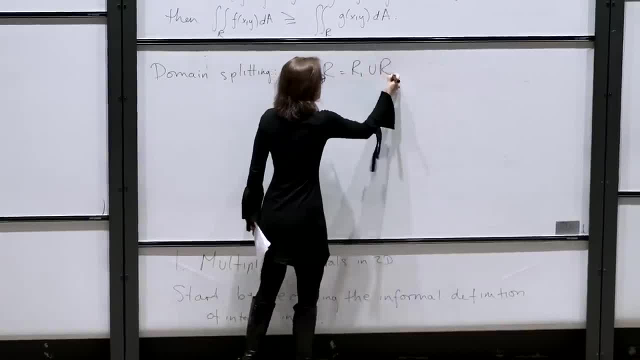 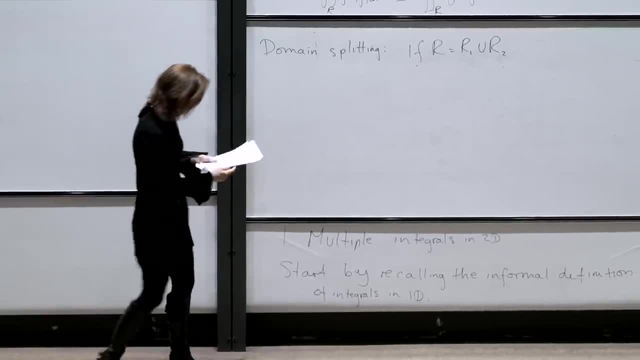 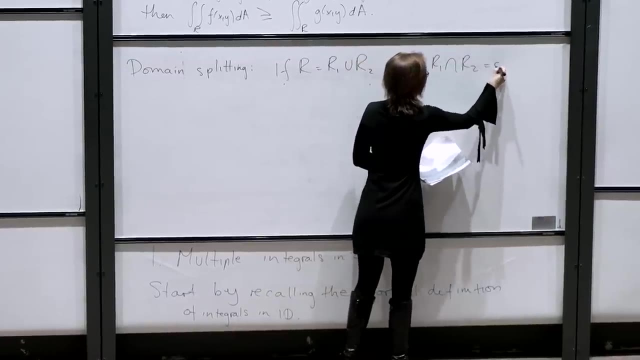 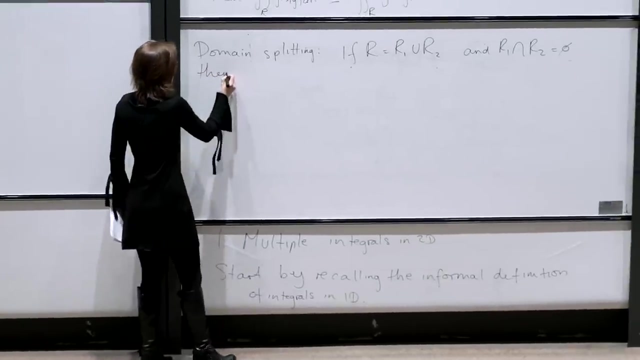 and that the function g of x is greater than or equal to the integral of n over x, y, dA, and then when we divide that into four, we'll get the function and the gradient of E to the head, which is called the gradient of E over a function g of x. So that could be 1.. Using this simple formula, we're going to get the gradient of x, y, dA, and if we can get equal to these functions, what do u by undestand 1 over x, y, dA? Canceling all values is a simple function. 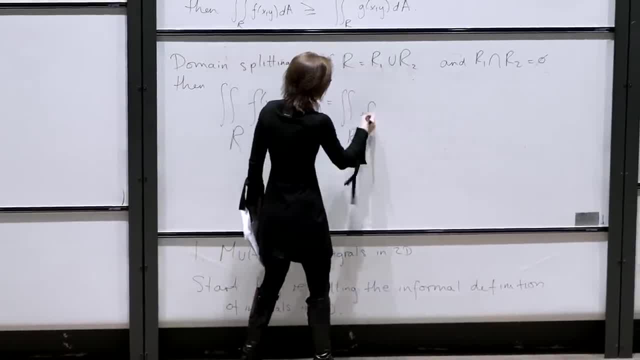 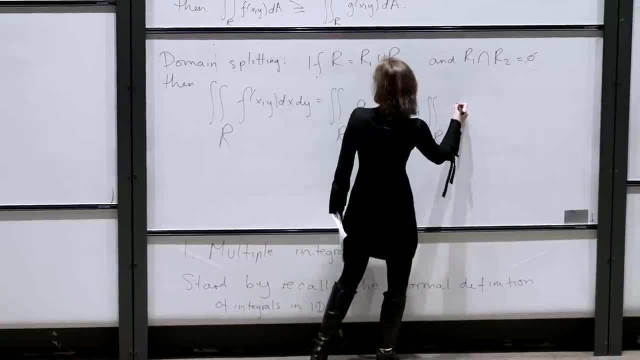 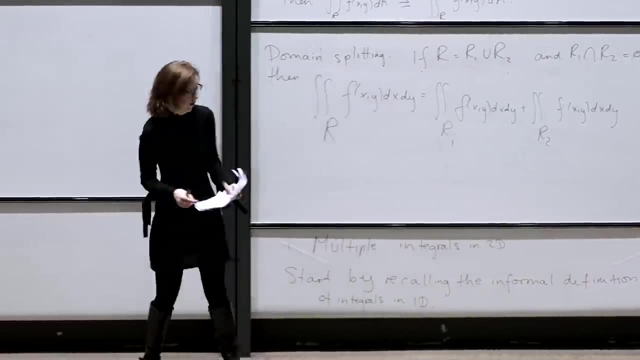 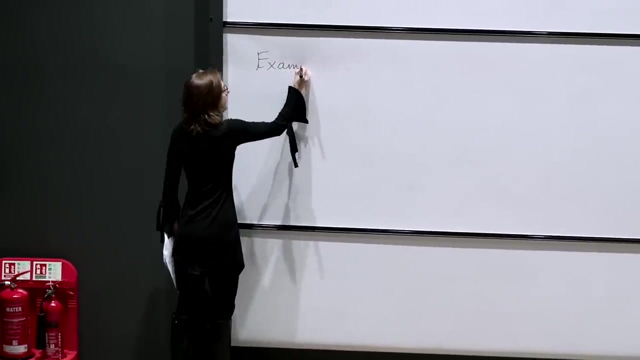 y equals the integral over r1 of f of x, y, dx, dy plus the integral over r2 f of x, y, dx, dy, And we'll certainly exploit that Right. so it's very helpful to see examples, And so we're going to start with a nice straightforward example, which is how we integrate some function. 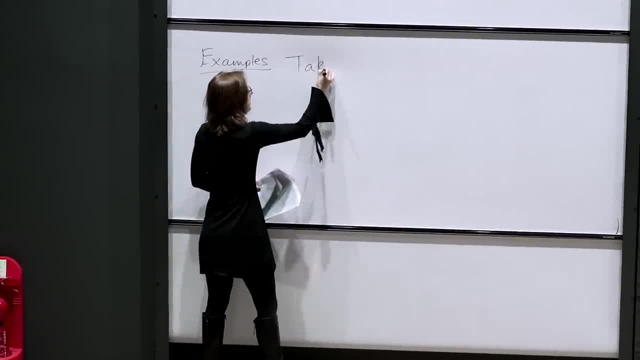 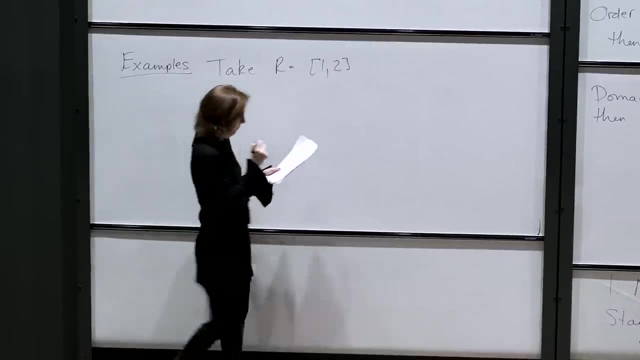 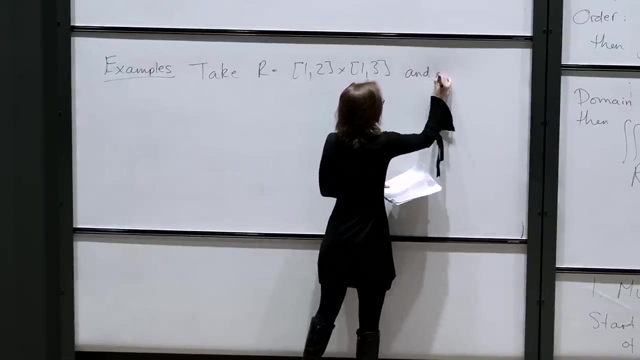 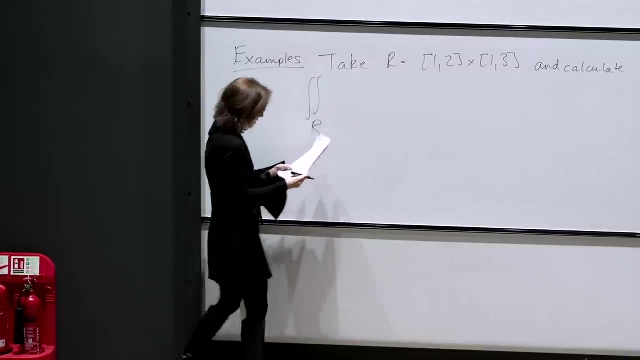 over a square or rectangular domain. So let's consider r to be the domain spanned by 1, 2 in the x direction and 1, 3 in the y, And we're going to calculate the integral over that region of r, x squared y, cubed, dx, dy. 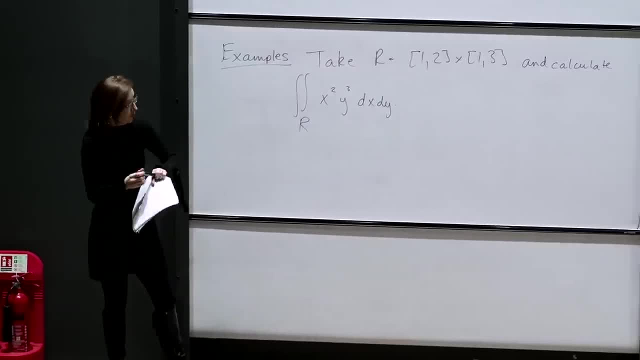 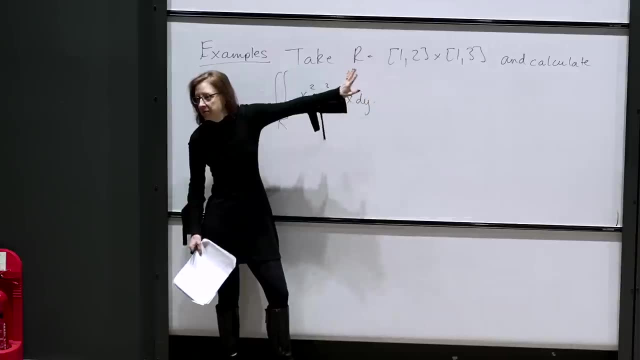 So this is much more simple than probably a lot of the problems you thought about in introductory calculus, mainly because the domain is very straightforward: It's just a rectangle, And when domains are rectangles you don't have to worry so much about being careful about your limits. So I would encourage you, when you're doing these problems, always: 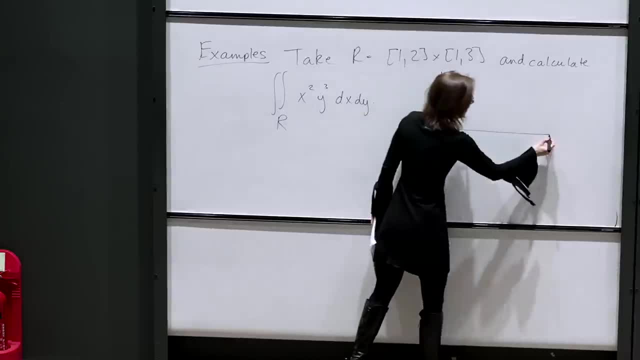 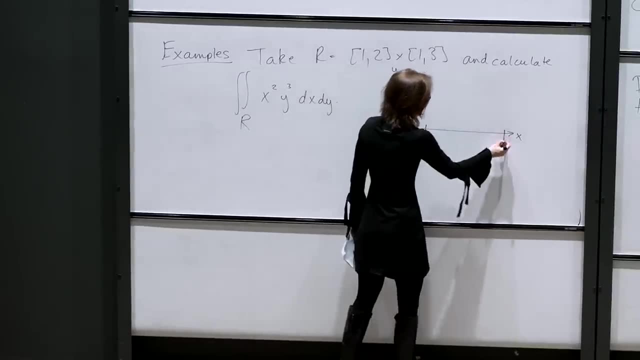 draw a diagram so it's clear what domain you're thinking about. So we have x along here and y along here. Then in the x direction, I'm going between 1 and 2.. And in the y direction, between 1 and 3.. And then in the y direction, I'm going between 1 and 2.. And then in the 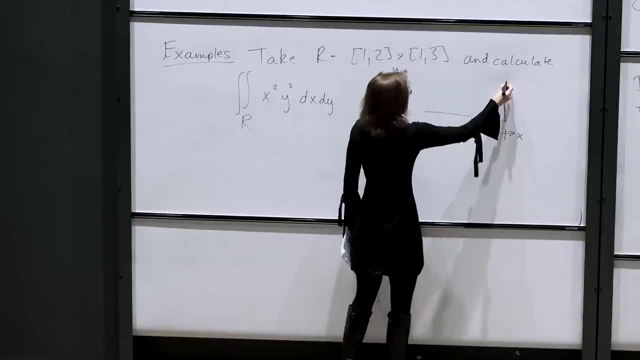 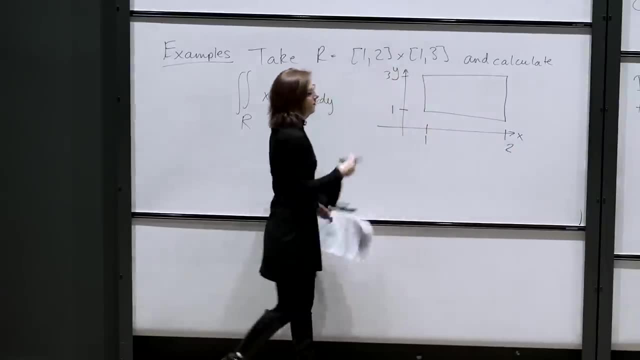 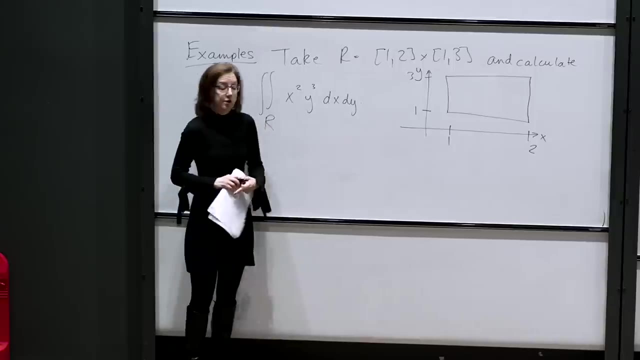 y direction. I'm going between 1 and 3.. So I'm integrating over some domain that looks something like that: So 1, 2, 1, 3.. So a nice, straightforward rectangular domain. So when you do these integrations you've got two choices. You can integrate first with 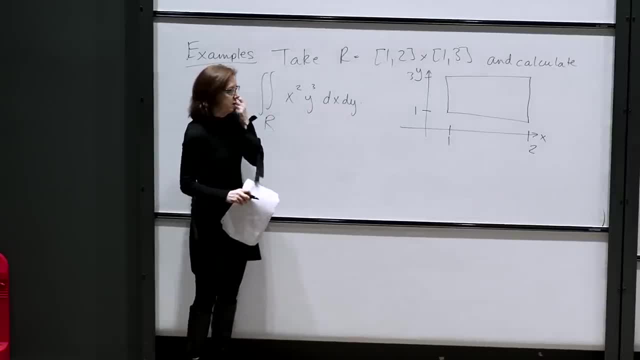 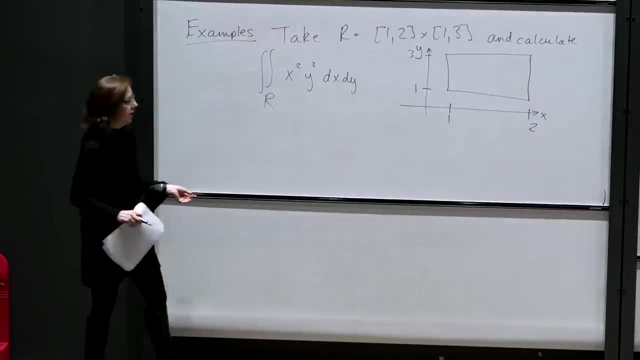 respect to x and then with respect to y, or vice versa, And it makes no difference. But we will see that sometimes it's better to do x first and then y, And sometimes it's better to do y first and x. So you're going to have a little bit of a problem there. 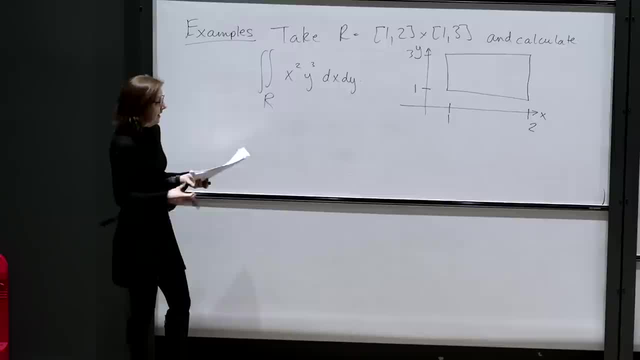 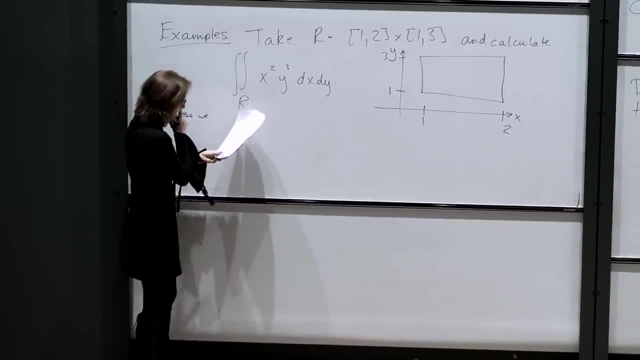 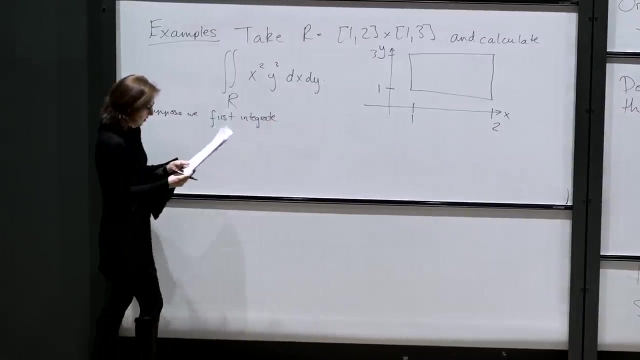 So let's have a look at a little bit of a problem. So we always work from the outside in. So let's suppose first we integrate. Sorry, We always work from the inside out. Suppose first we integrate with respect to x keeping 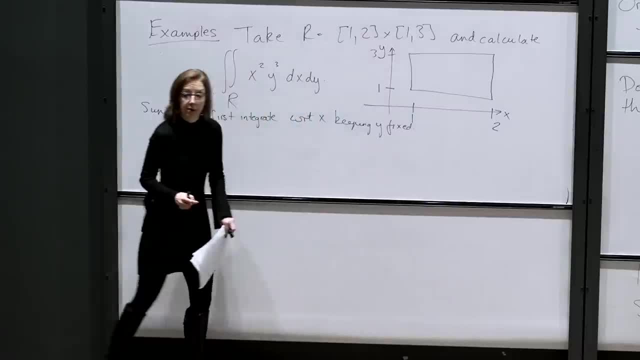 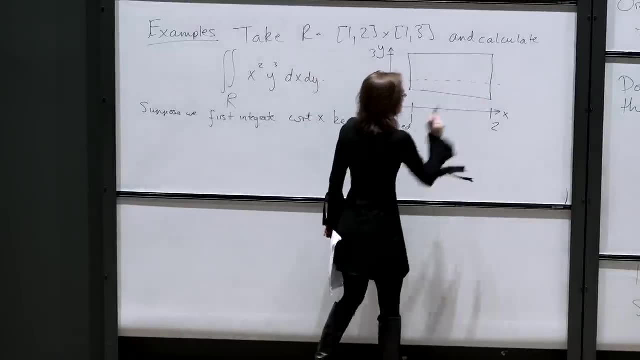 y fixed. So if we're doing that, then what we mean we're doing is we're going to fix y, so we're going to just consider some value of y- let's suppose this one- and we're going to integrate with respect to x. so what we're doing in this, when we do it in this, 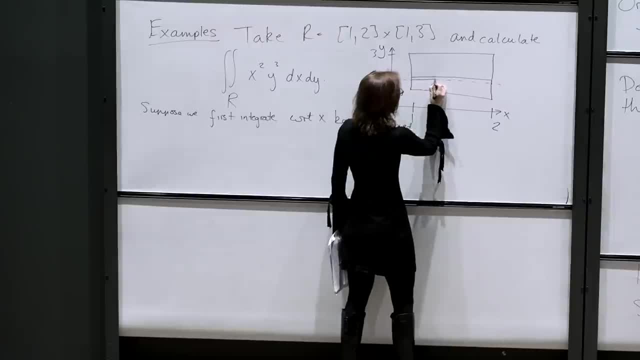 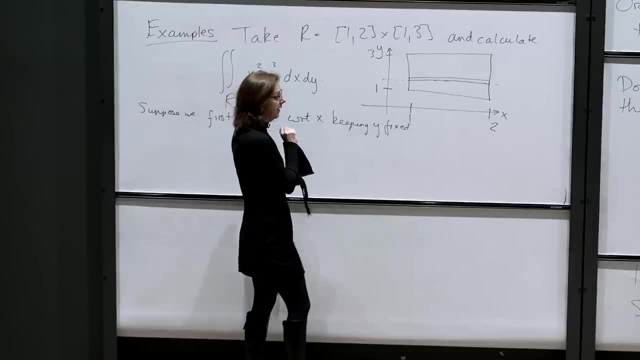 sense is we split our domain up into lots of slivers that are horizontal and then we sum them all up equally. we could have integrated first with respect to y, keeping x fixed, and when we do that we split the domain up into slivers that are vertical. but it makes no. 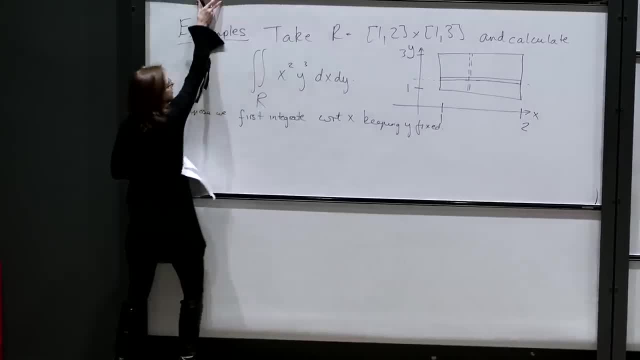 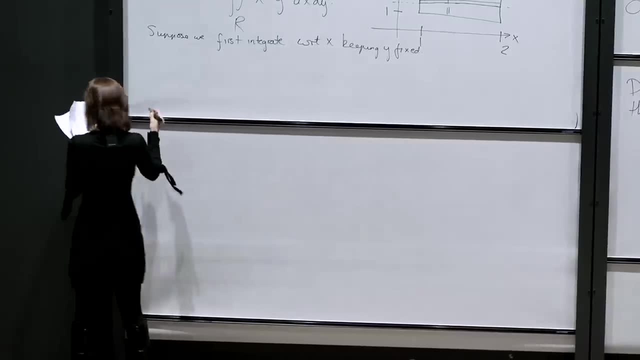 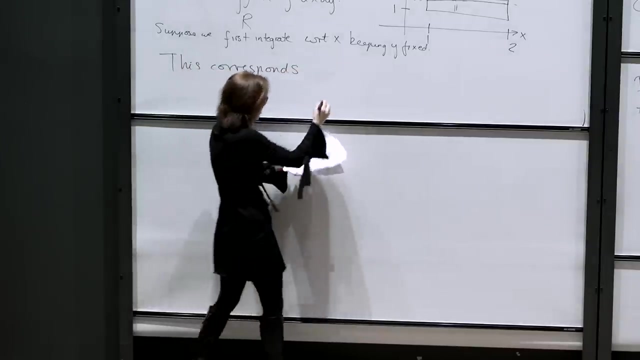 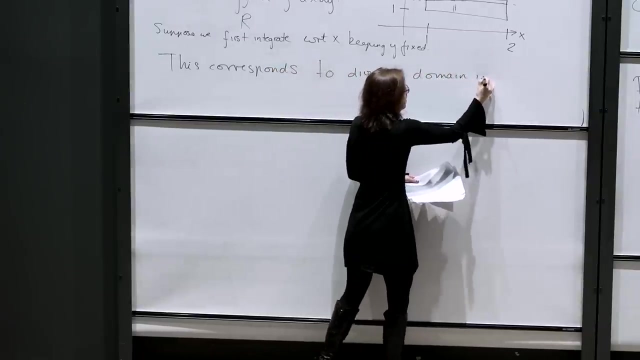 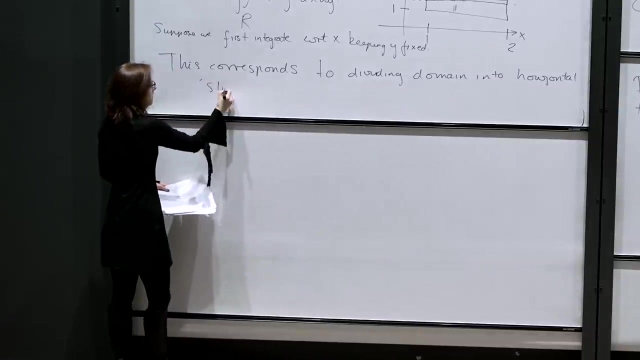 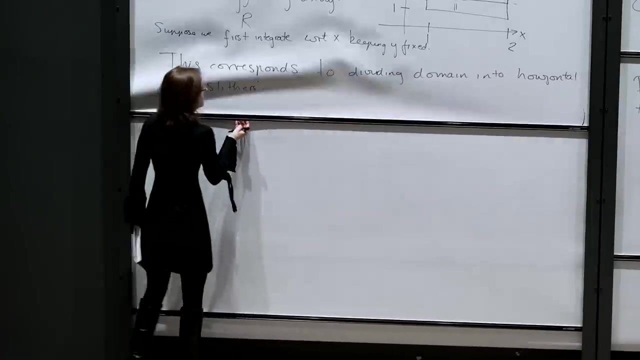 difference. okay, so if we integrate first with respect to x, keeping y fixed. oh so this corresponds to splitting our domain up into horizontal slivers. dividing domain into horizontal slivers? all right, so let's do that. so we're going to integrate first with respect to x. 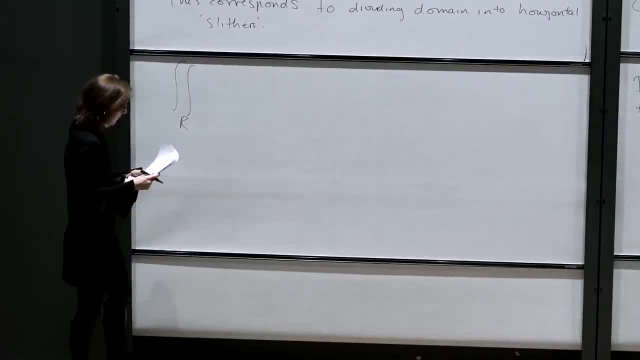 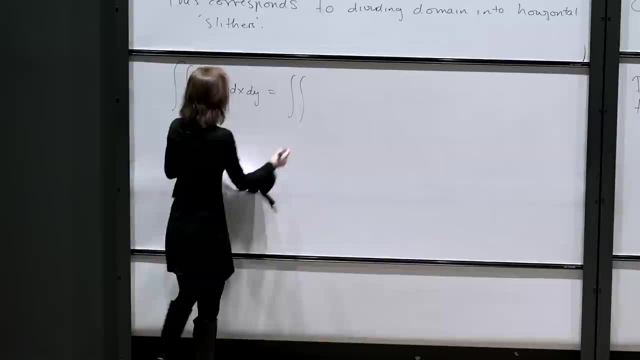 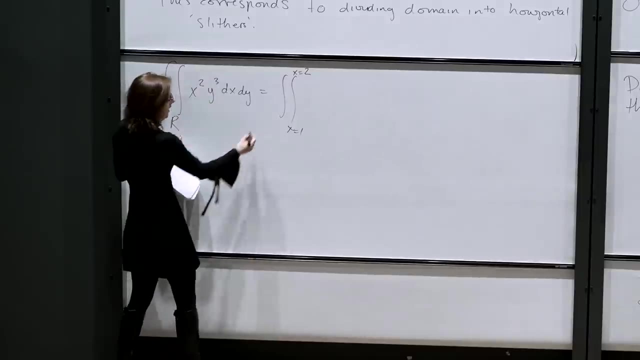 so that means that the integral over my region of x squared y, cubed dx, dy is just the integral, so integrating. with respect to x, my limits go between x equals 1 and x equals 2. my y is between y equals 1 and y equals 3. 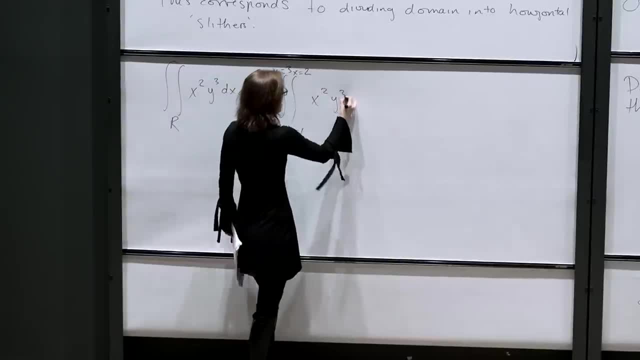 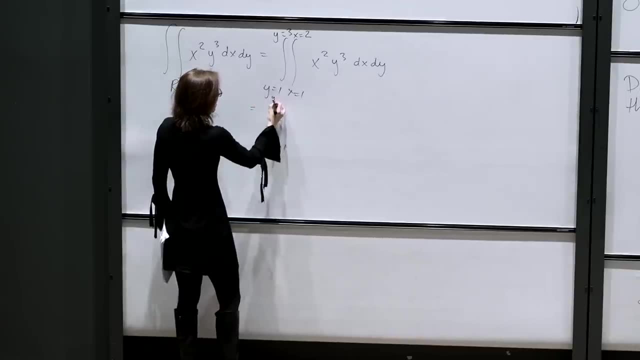 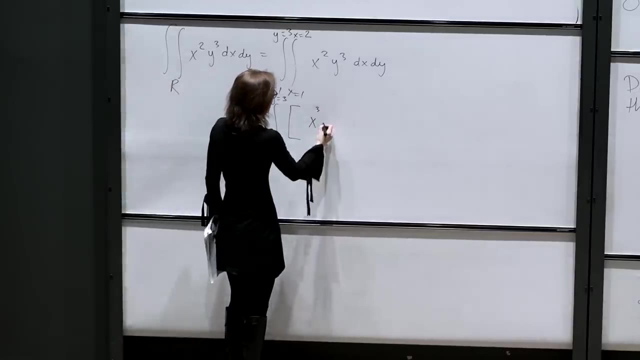 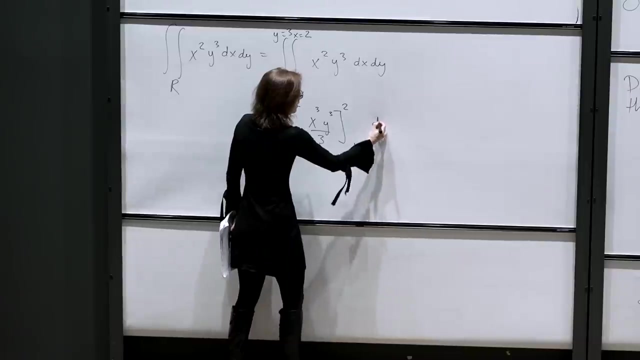 x squared y cubed, dx dy. so keeping the outside integral in play and integrating x squared y cubed with respect to x gives me x cubed, y cubed over three. now i put in my limits between one and two d y. so i'm going to integrate x squared y cubed with respect to x gives me x cubed, y cubed over three. now i put in my limits between one and two dy. 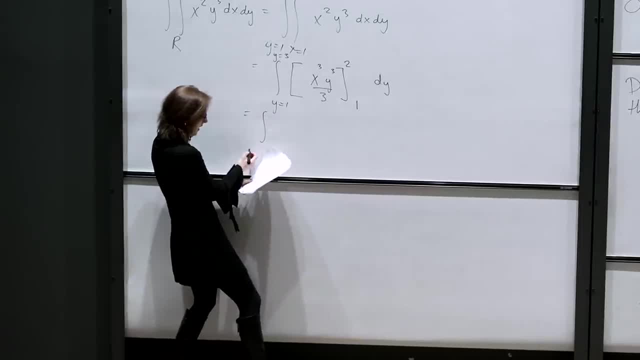 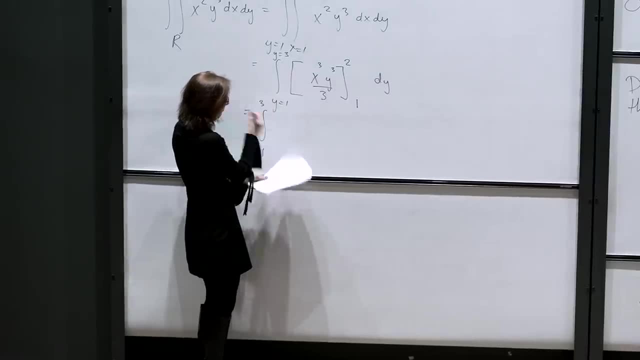 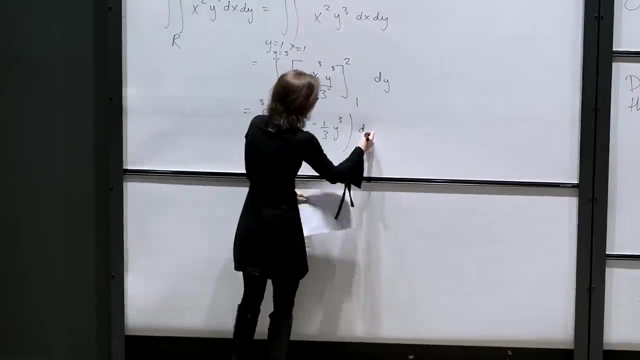 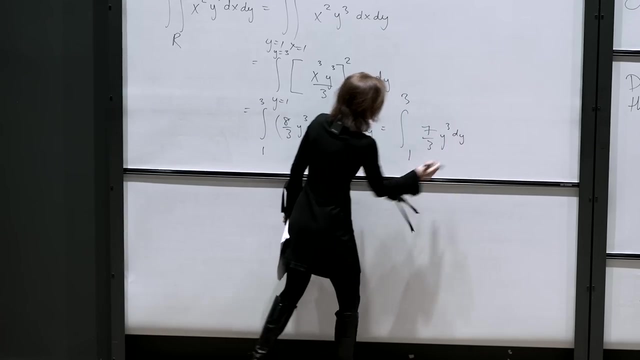 which, if i don't mess up my algebra, i think is the integral from one to three of eight thirds y cubed minus one third y cubed dy, which is the integral from one to three of seven thirds y cubed dy. now i've got a very easy integral to do, just a single integral. as i said, by now i have excellent idea of whichlanguage is exactly the same thing. but this idea where i make the Lorentz equation and applied these three ancient vectors- here i already know what they do, but is say they include one and two, two third, us 카� was one and one over ten divided by three. 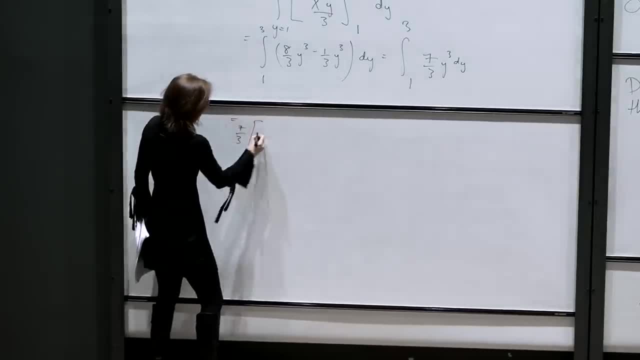 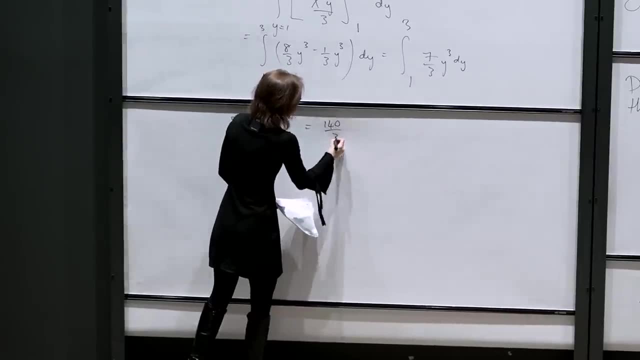 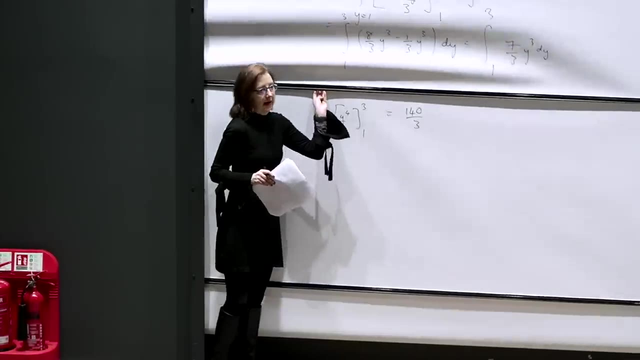 so that just becomes 7 thirds y to the 4 over 4, between 1 and 3, which is 140 over 3. and the reason this integral was so straightforward to do is because the domain is so simple. the x and the y, if you like, are independent because you're integrating over in a rectangular domain. so 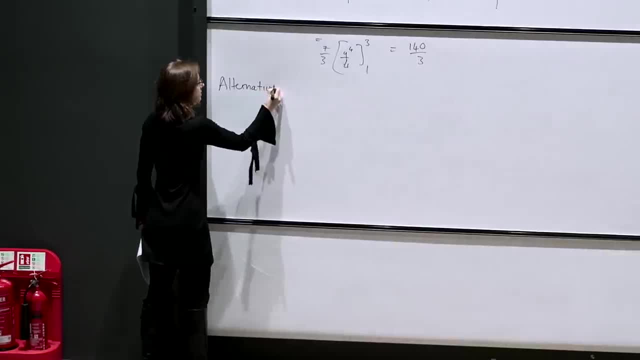 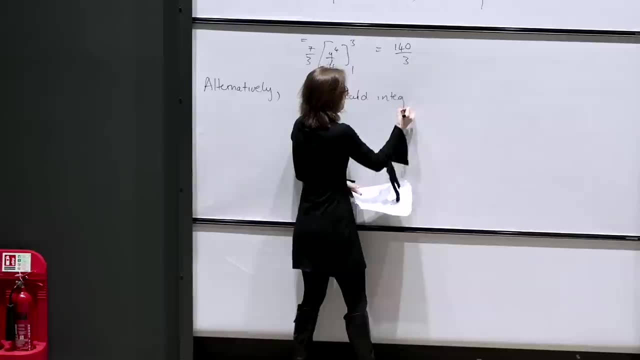 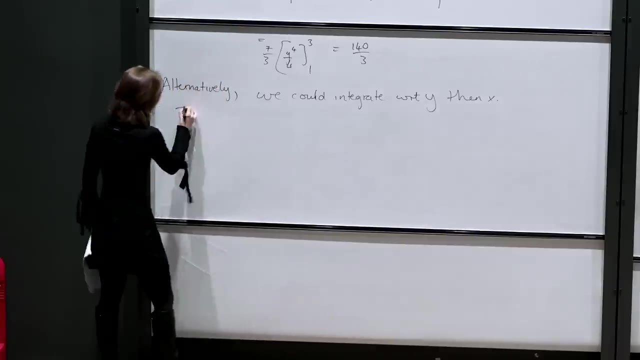 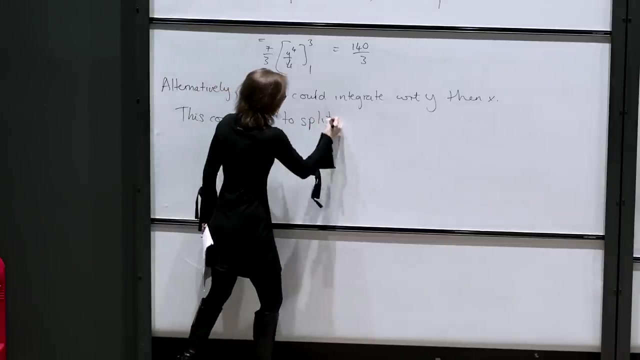 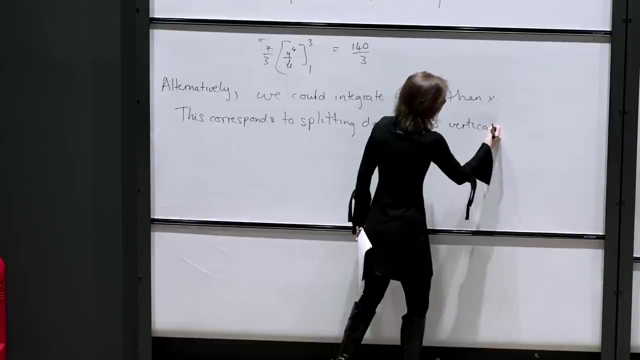 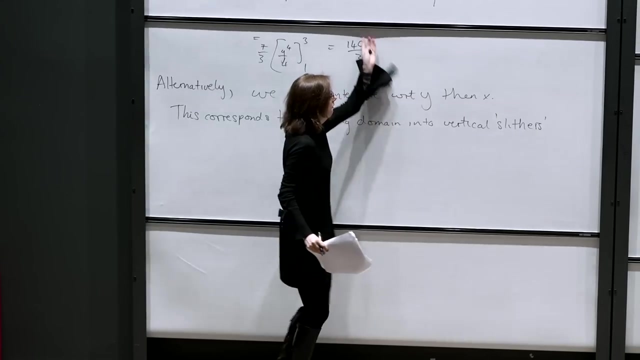 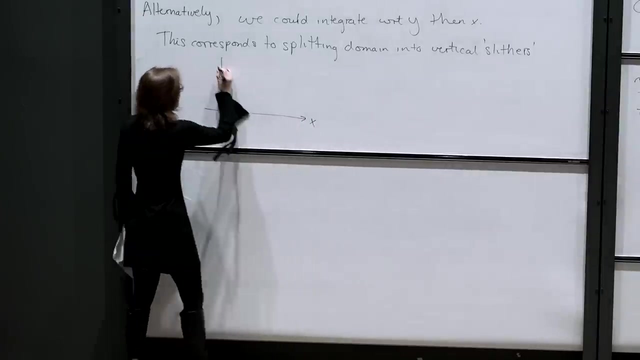 alternatively, you could integrate with respect to y and then with respect to x, so with respect to y, then X. so this corresponds to splitting the domain into vertical slivers. okay, so if we're thinking about what we're doing, so the domain is here somewhere and what we're? 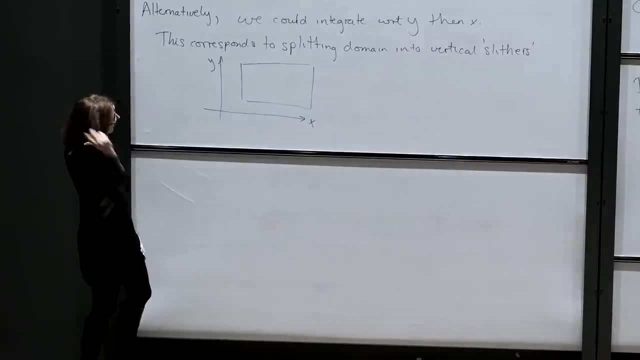 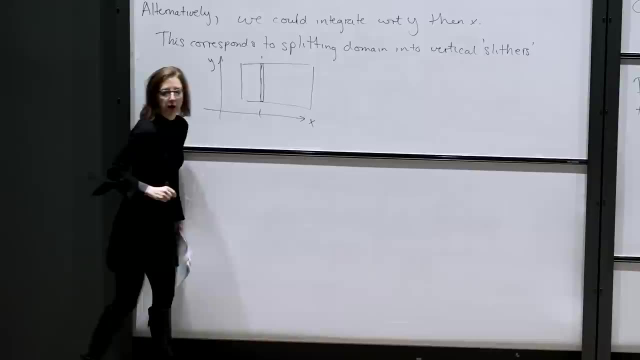 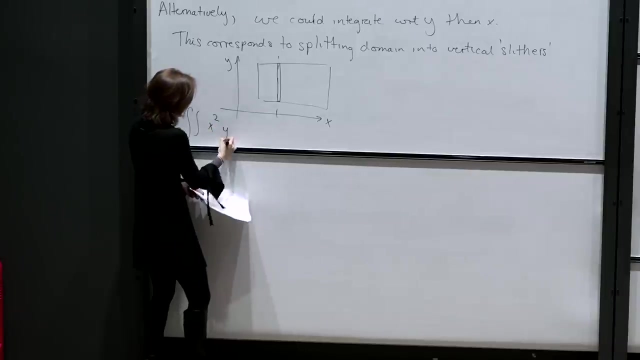 doing now is saying: right, going to fix X, that, and then I'm going to split my domain into these vertical slivers and then sum them all up to get my area. so now the integral over R of x squared, y cubed. but now with respect to y first, 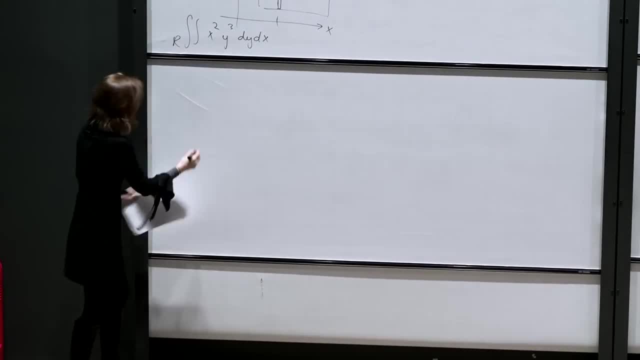 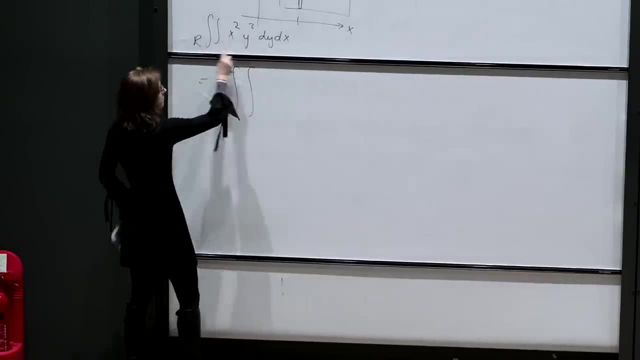 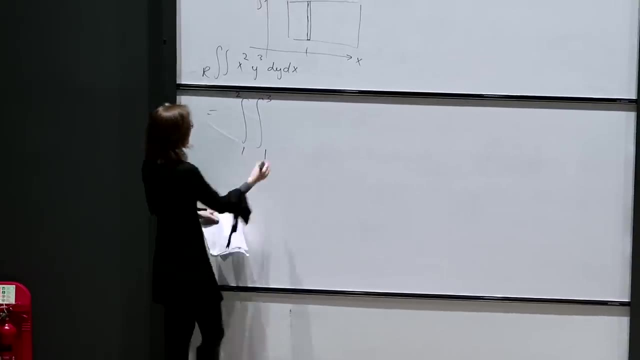 so dy dx. so we change the limits because we switch the order of integration. so now the x is the outer integral that's appearing here, so that goes between 1 and 2. the y is the inner, so that's between 1 and 3. now we get x squared, y cubed. 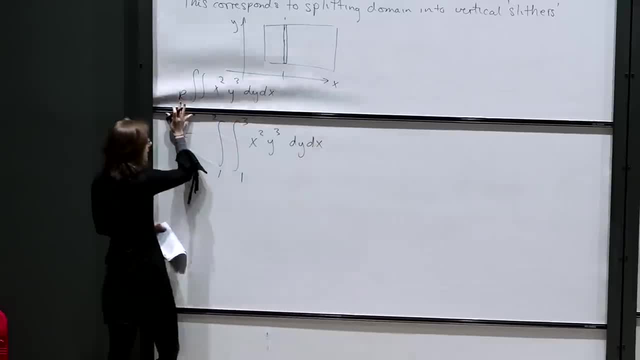 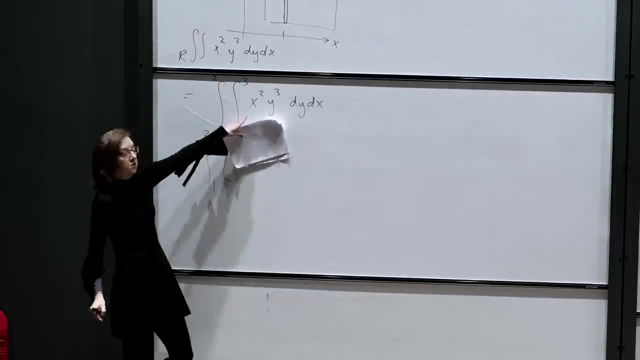 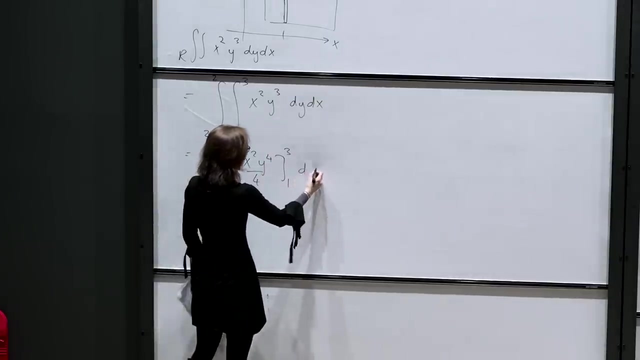 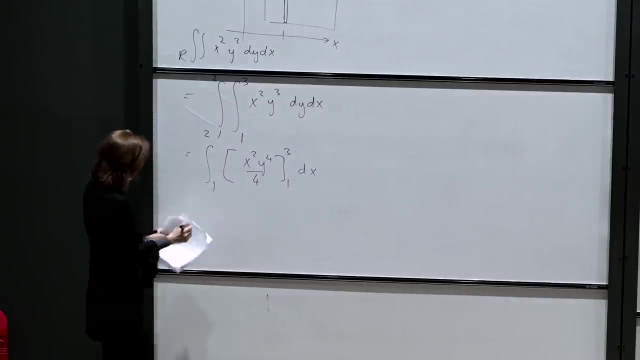 dy dx and we do the same as before. so we work on the inside out and we get integrating. this integrand with respect to y gives us x squared y, 4 over 4 between 1 and 3 dx, which is cut. a longer story short, 20. 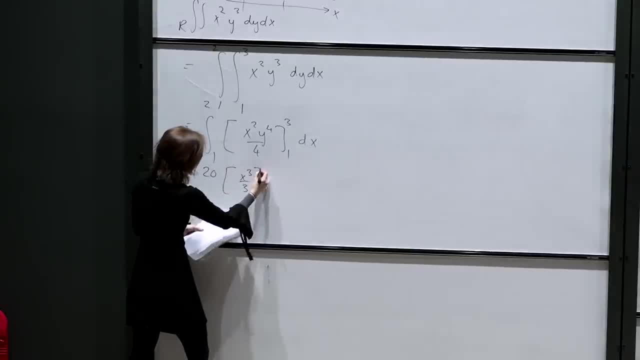 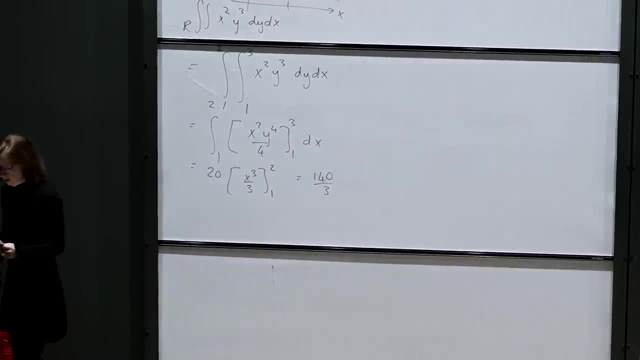 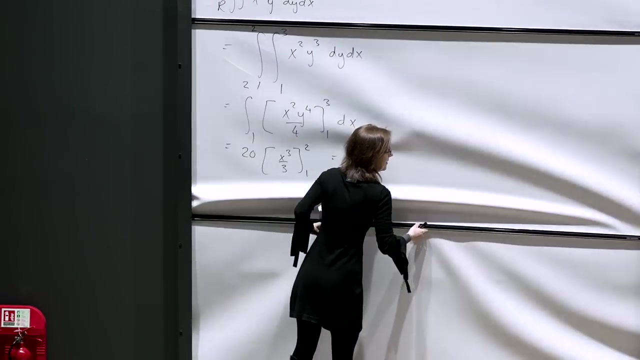 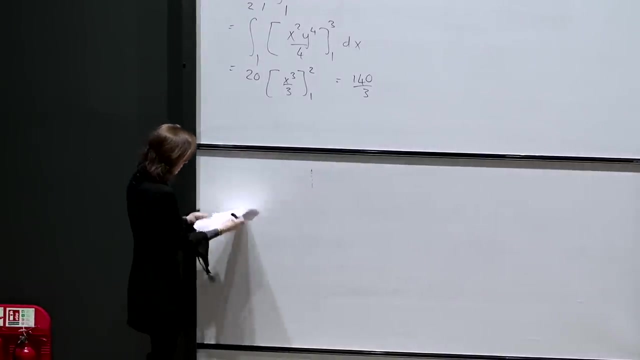 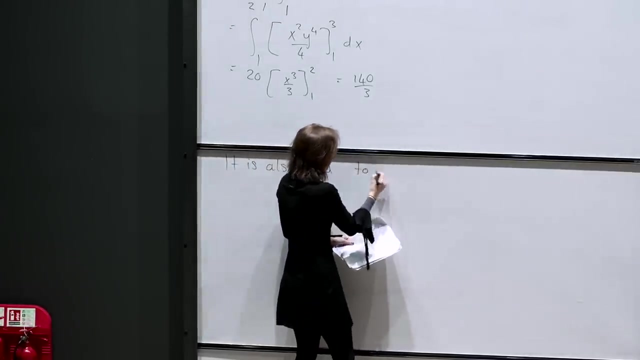 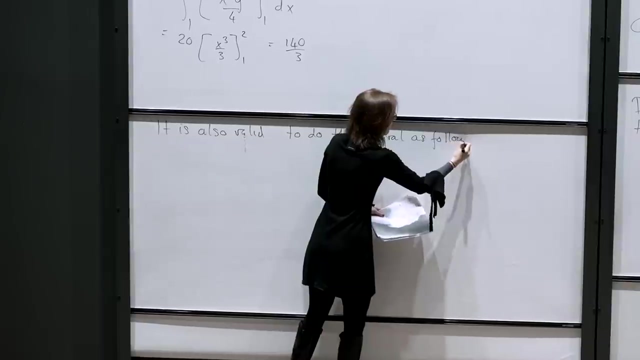 x cubed, cubed over 3, between 1 and 2, which is 140 over 3, as expected. so it doesn't matter what order we do things in, we get the same answer as you expect. okay, you could also do in this case to do the integral as follows: so what we could do is acknowledge the fact we're integrating on. 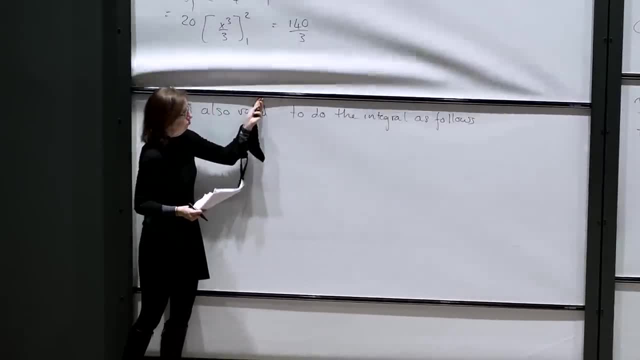 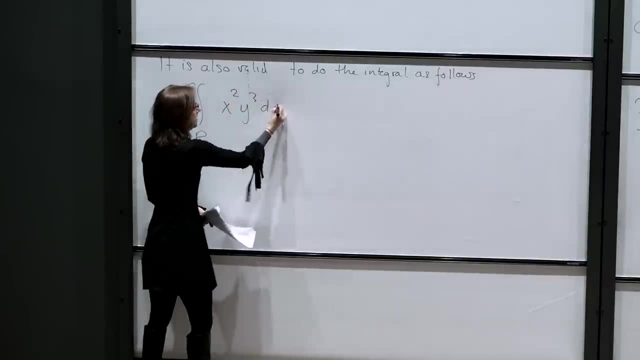 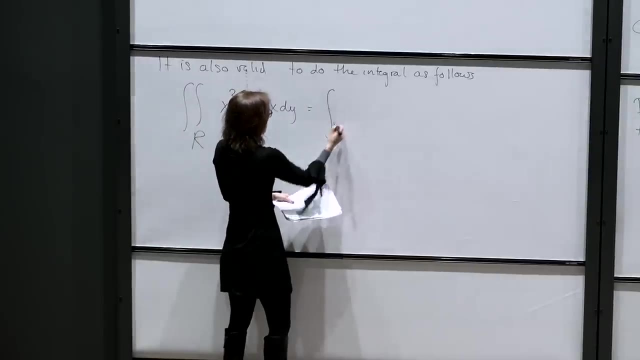 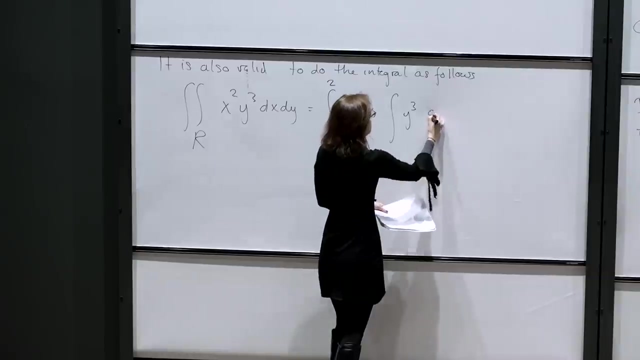 a rectangle and then we have the integral over r of the integrand x squared y cube dx dy and we can actually split the integrals up and we can do the x squared dx. so we can do the x squared dx between one and two times the y cubed dy between one and three. and if i do that of 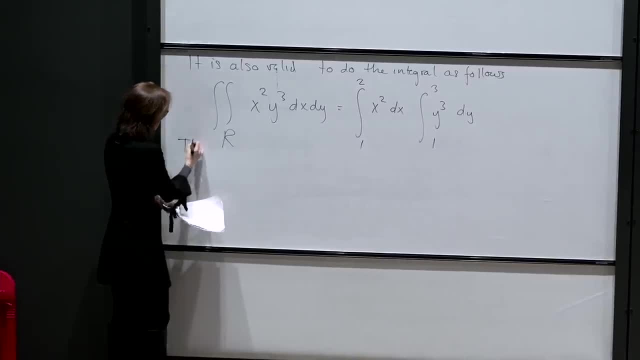 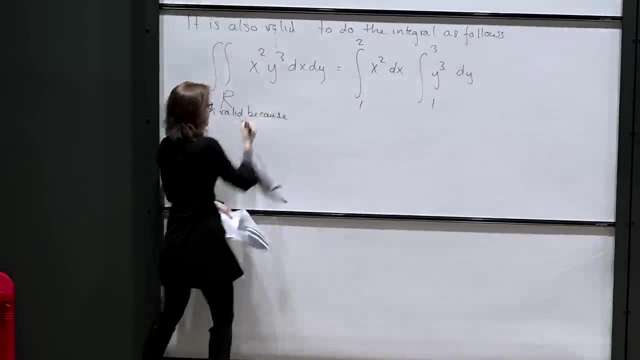 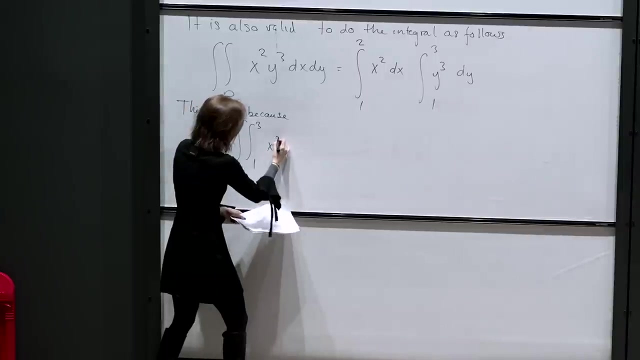 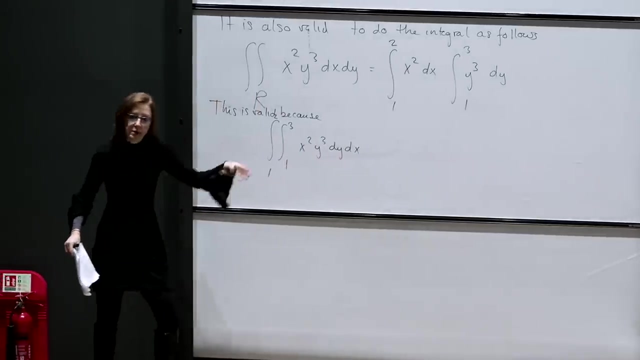 course we'll get the same answer. and this is valid because when i'm doing the integrals, so when i integrate one, two, one, three of x, squared y, cube, dy, dx, so when i do the integral here with respect to y, i'm holding x fixed. so as far as i'm concerned, 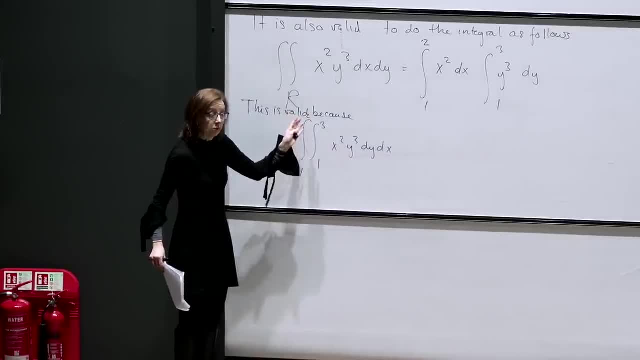 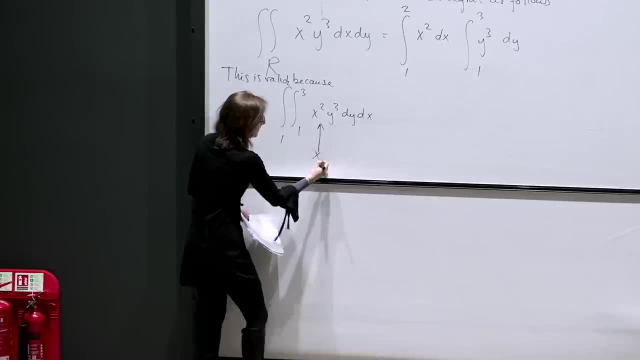 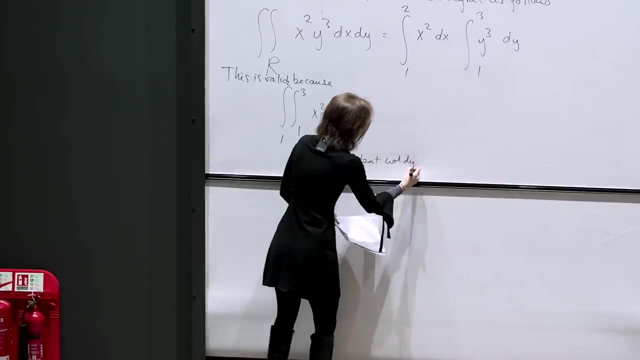 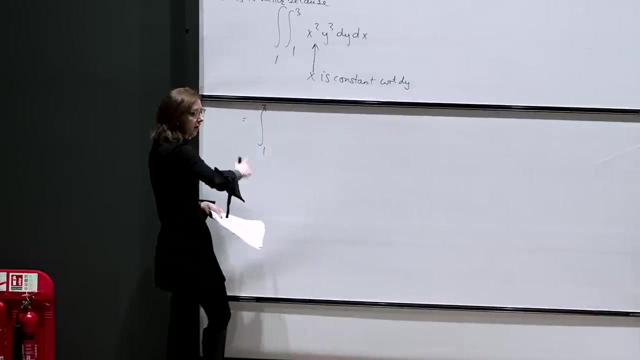 with this x is just some constant and then i can use linearity to pull it out. so this: when i'm doing the y integral, this x is constant or held constant with respect to dy, and so i can just write this as one. two: i can pull the x squared out of the y integral. x squared, the integral from one to three of y cubed. 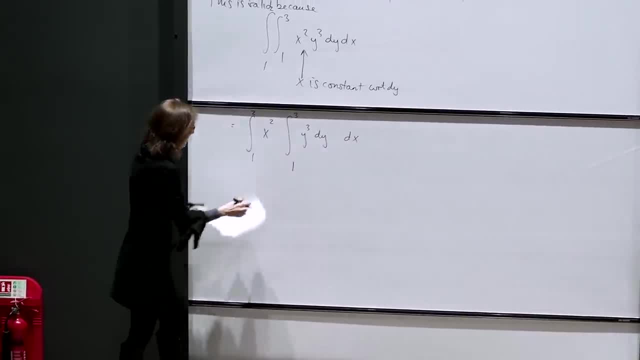 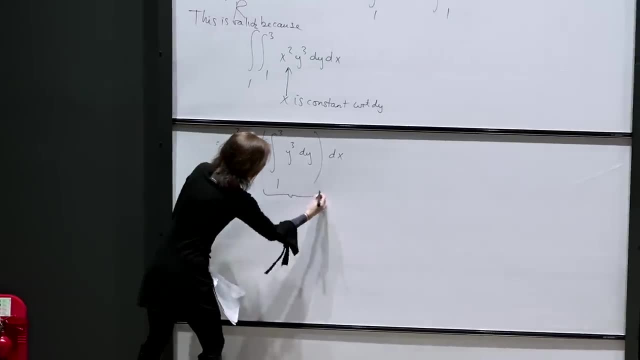 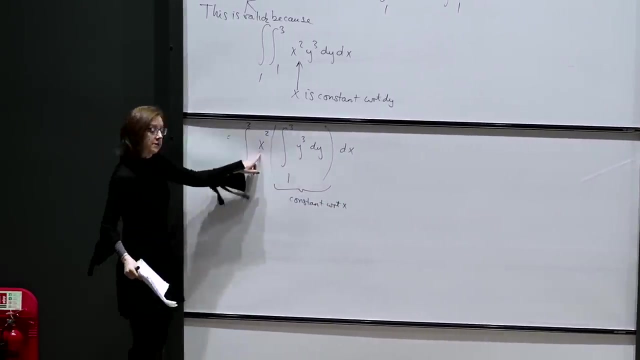 dy, dx. and then this is just a constant with respect to x. so i play the same game and pull it out. so this is constant. so when i'm doing my x integration, i'm integrating the x squared, but this has just become a number so i can pull it out. 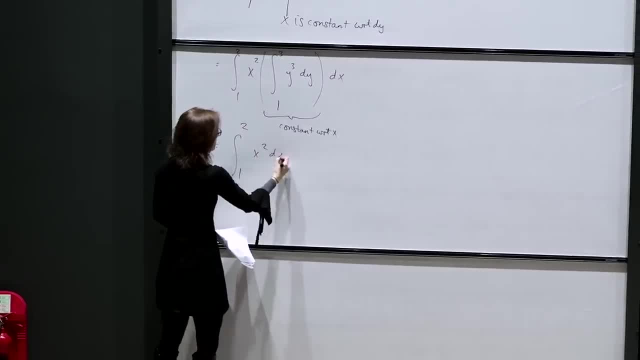 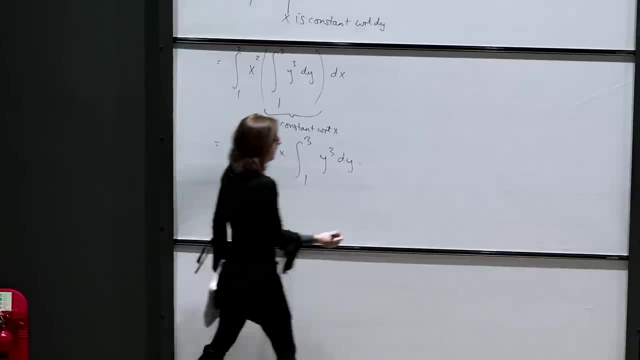 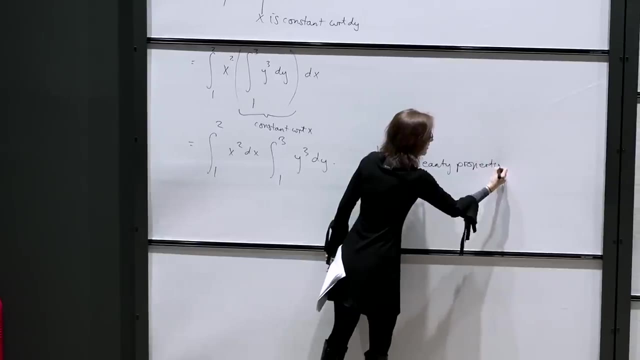 and so i get the integral from 1 to 2, x squared dx, the integral from 1 to 3, y cubed dy, bilinearity. so those properties that um we covered can be exploited when you're making decisions about how to do your integration. and in fact, if you look at the lecture notes as a whole, 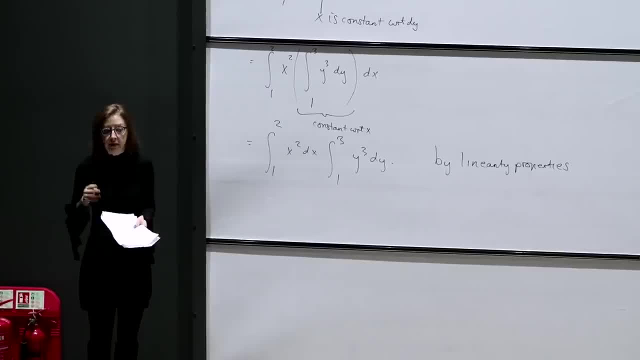 i think on page four of the online lecture notes there's some further properties that you would expect to see when you do the lecture notes, like this: if you have a question like kind a, these double intervals which you can exploit, but it can also be used as sanity checks. 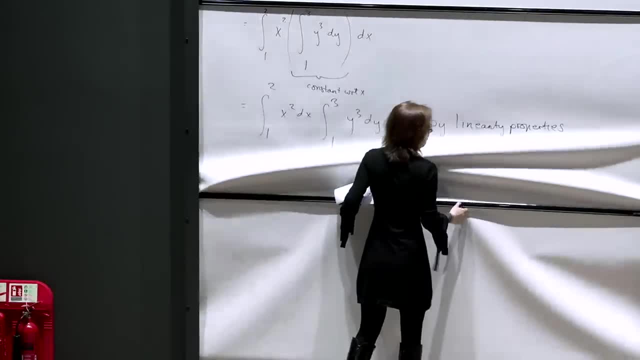 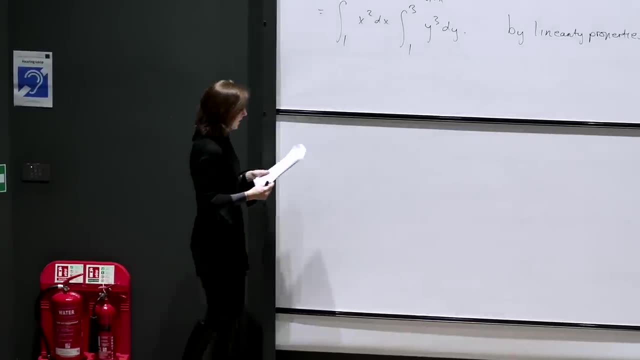 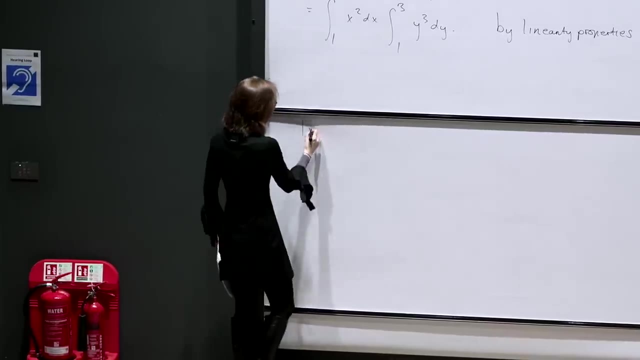 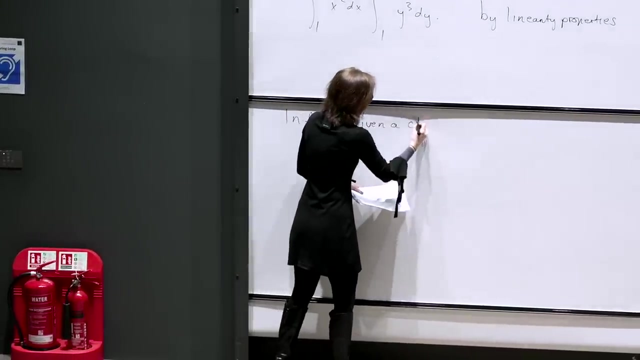 So I would encourage you to look at that, because I'm not going to write them down here. It's all in the lecture notes, Right, Okay? So it doesn't matter which way we integrate- with respect to x or with respect to y- And in fact we can write that as follows: So, given a continuous bounded, 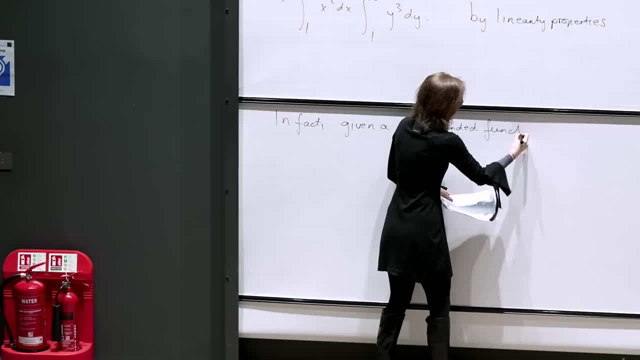 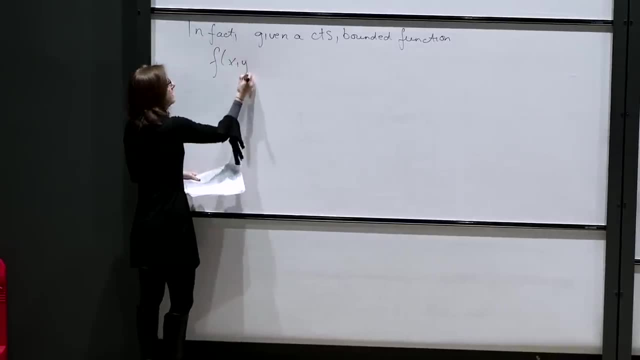 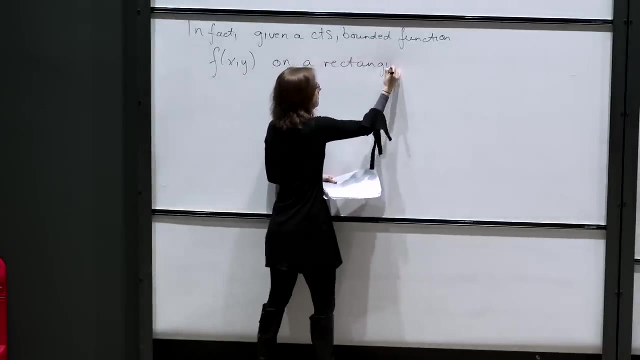 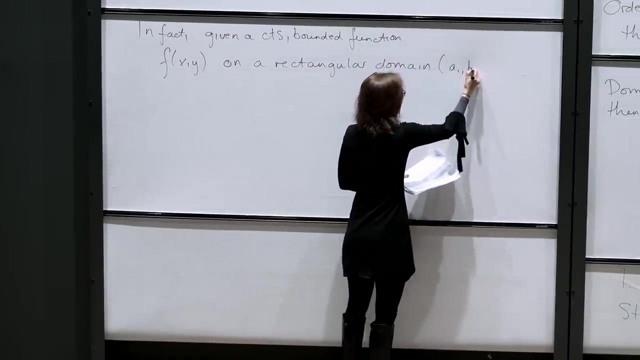 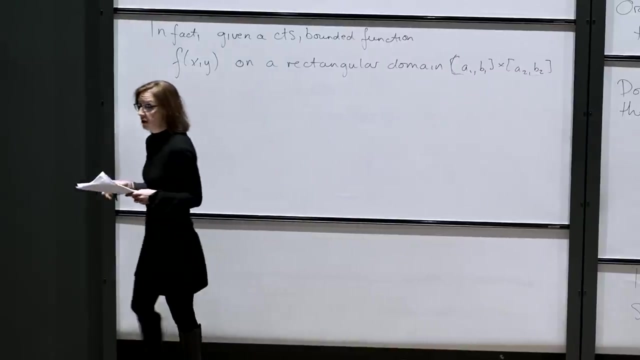 function, so f, which is a function of x, y, given that on a rectangular domain. so we're going to write that as a1, b1, cross with a2, b2. So we're just thinking about functions that are continuous and bounded on a rectangular domain. Then it is the case. 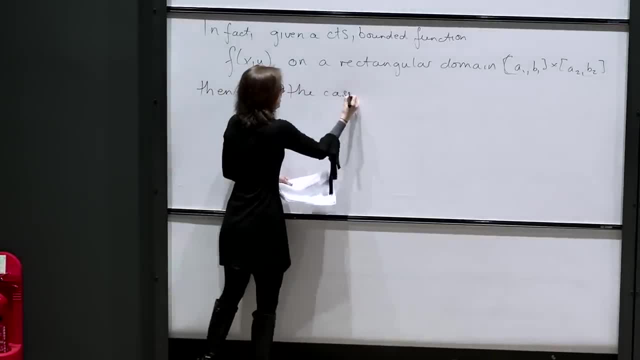 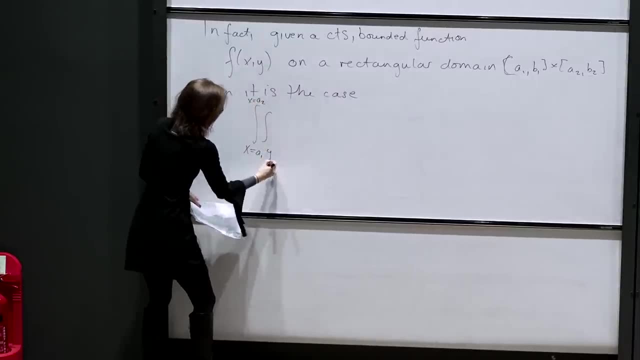 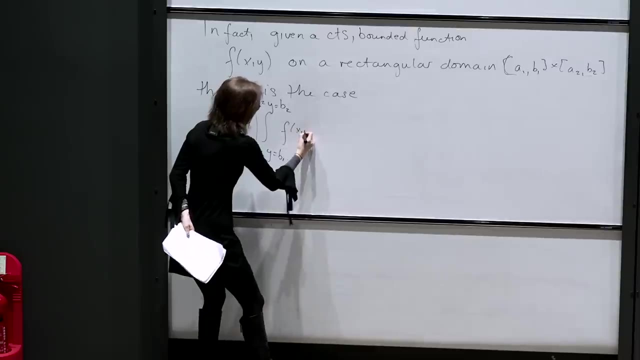 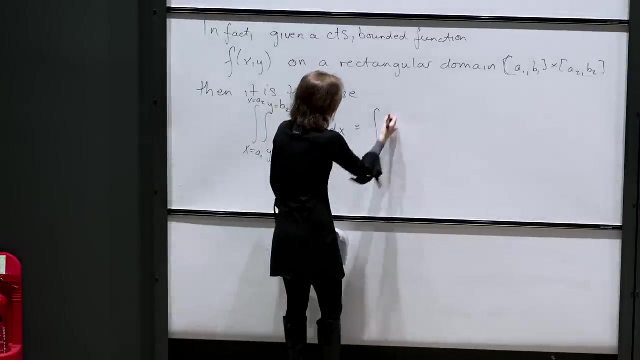 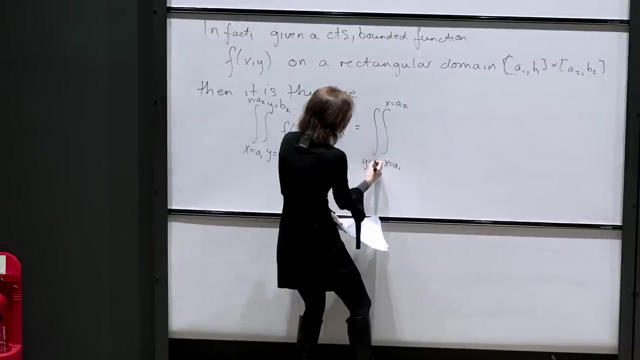 that the integral from x equals a1,, x equals a2, y equals b1, y equals b2, of my function, f of x, y, integrated with respect to y and then respect to x is equal to the integral from x equals a1,, x equals a2, y equals b1, y equals b2. of f of x, y. 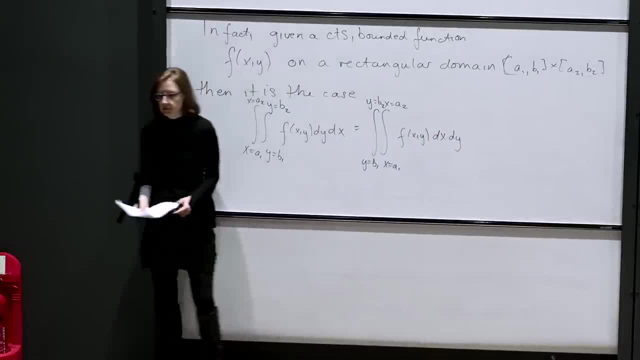 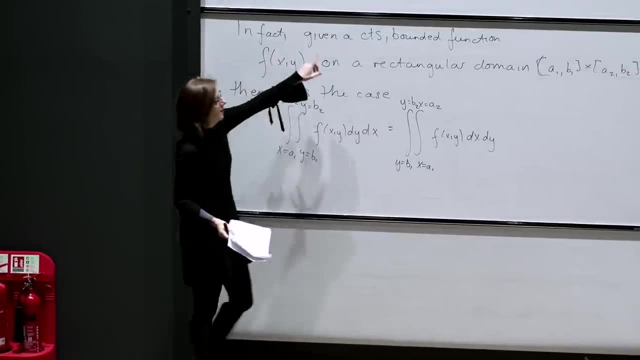 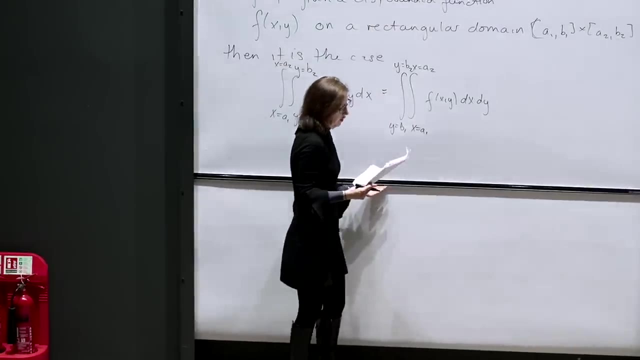 Now doing the x integral first and then the y integral, But this isn't true for all functions f. This is true when f is continuous and bounded. And one of the questions on the example sheet- example sheet one looks at a case where the function, the integrand that you're integrating is continuous. 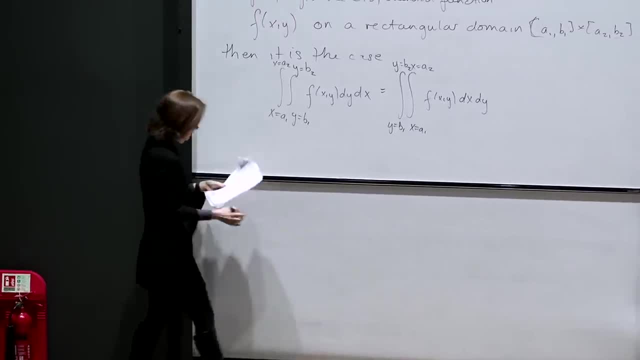 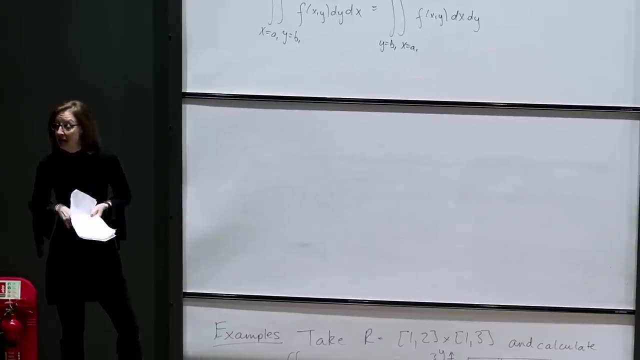 but it's unbounded, And then you'll see that this doesn't hold. That's okay. So rectangles are nice and straightforward. As long as we're bounded and continuous, everything's going to behave itself. But of course we want to do more. 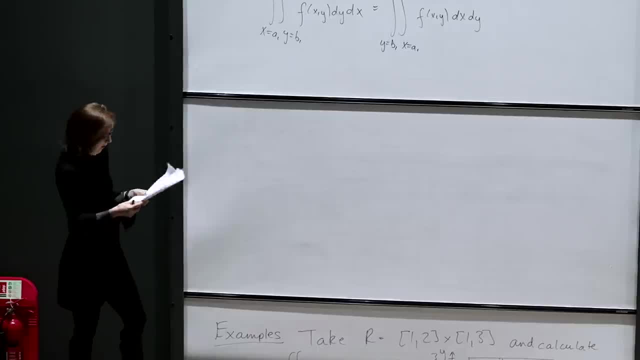 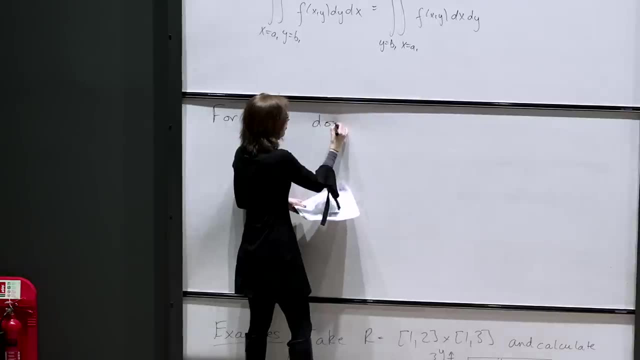 interesting integrations, So we're going to do more interesting integrations. So we often encounter them in problems we consider, And so for general domains, this is not so straightforward. It's the general domains that are not simply rectangles. 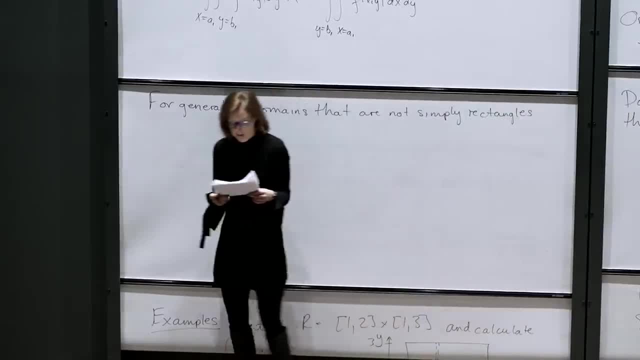 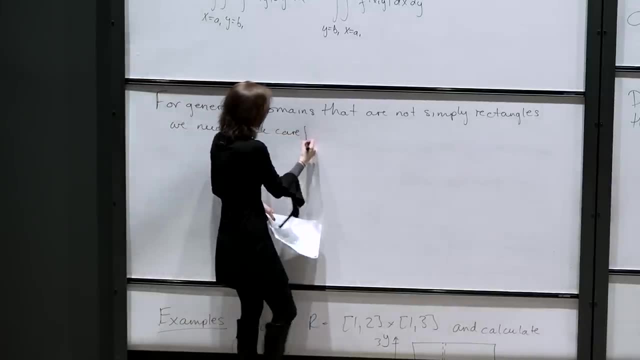 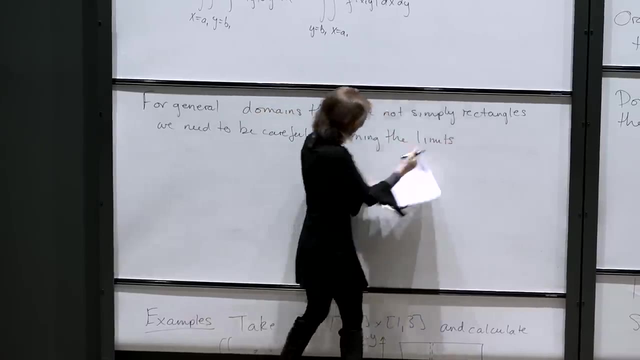 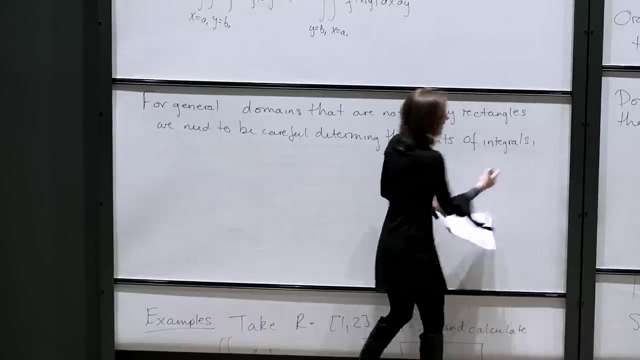 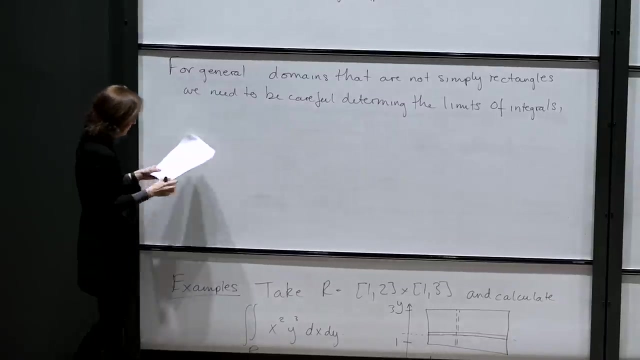 Then we have to be much more careful, especially with the limits. So we need to be careful determining the limits of integrals, And it might well be the case- and often is, that it's better to do it one way first and then the other way than the other order of integration. And it may well be. 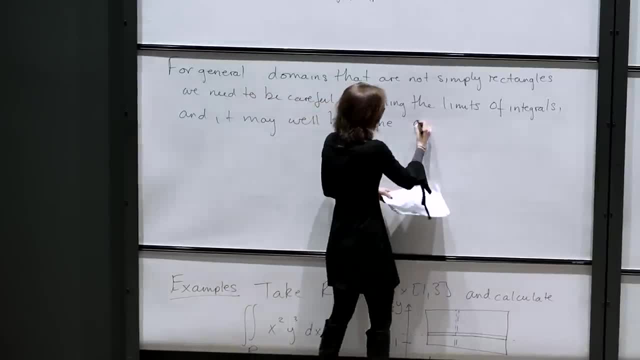 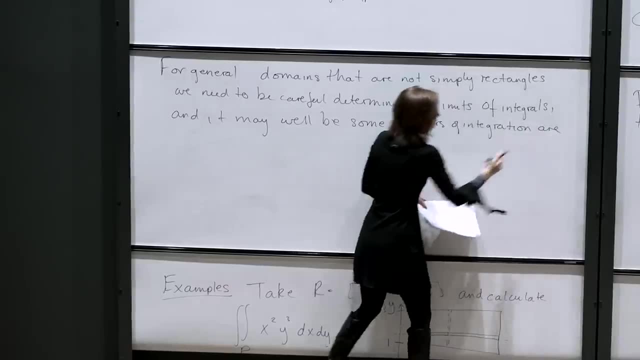 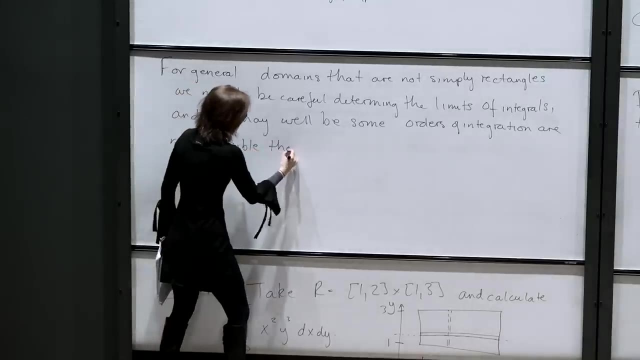 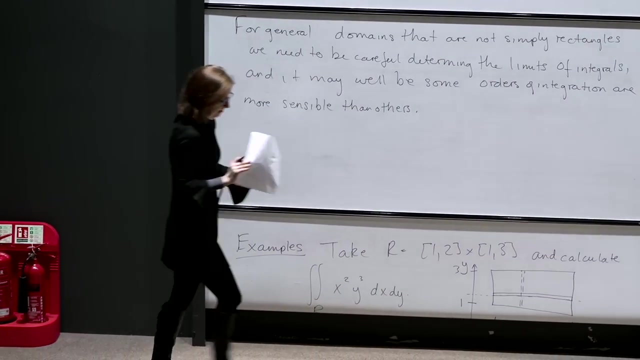 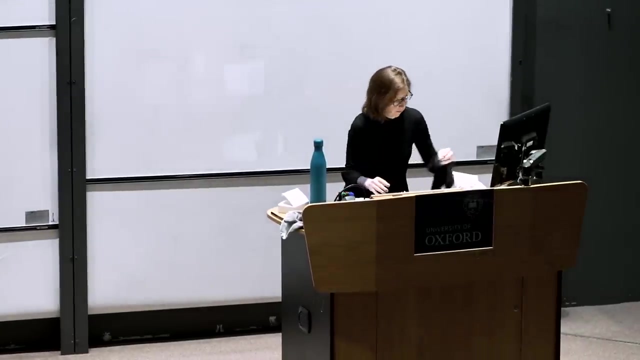 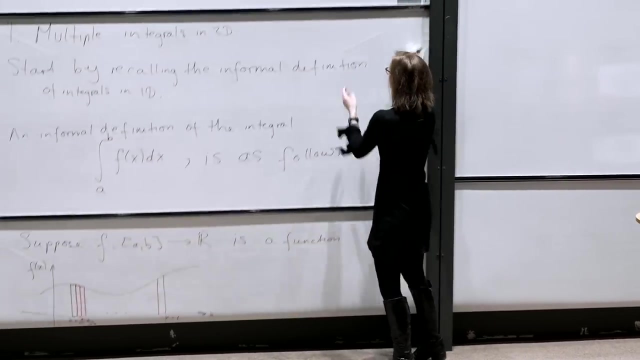 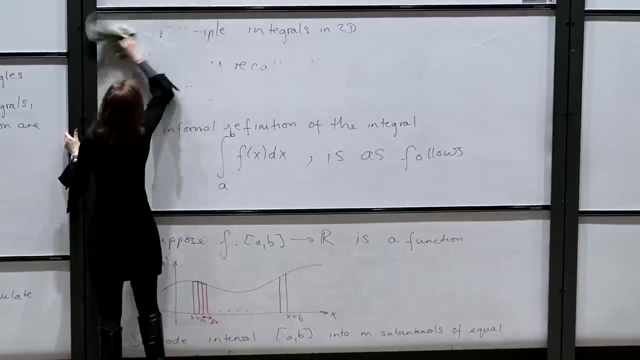 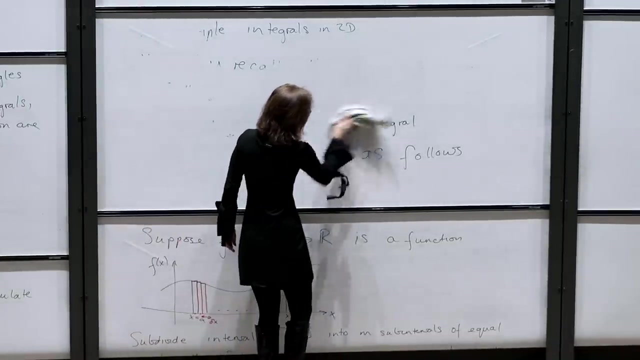 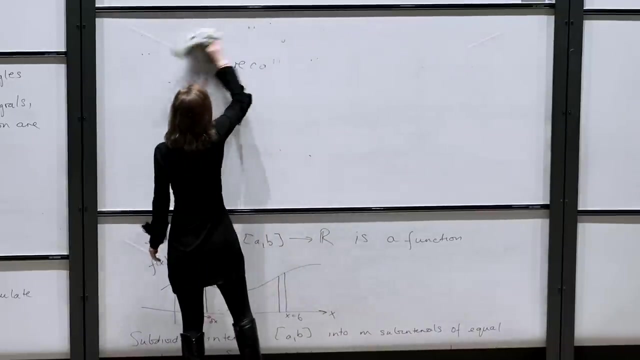 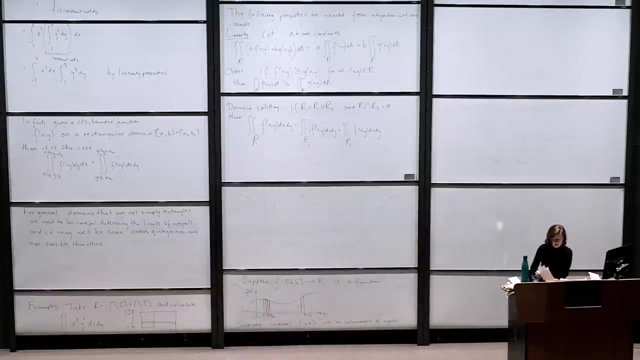 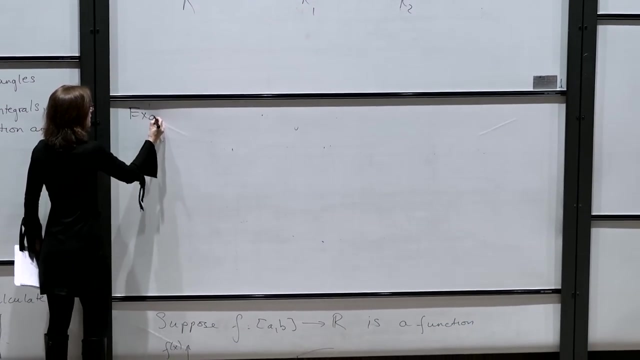 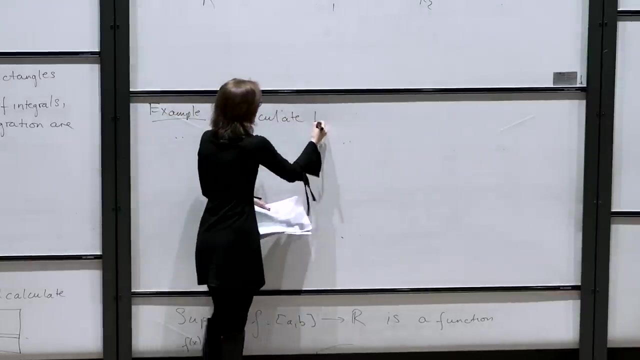 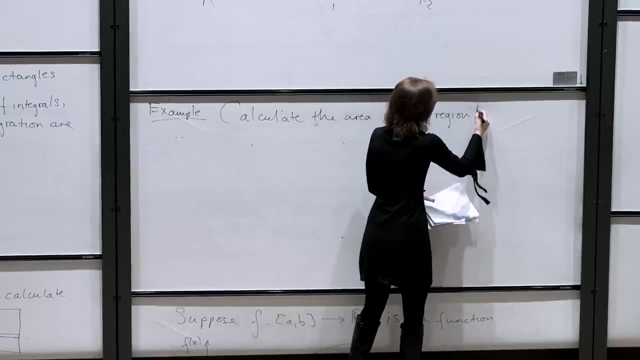 the case that some orders of integration are more sensible than others. Okay, Thank you. All right, so let's think about something a bit more complicated. So now let's consider. so another example. Let's calculate the area of the region R. 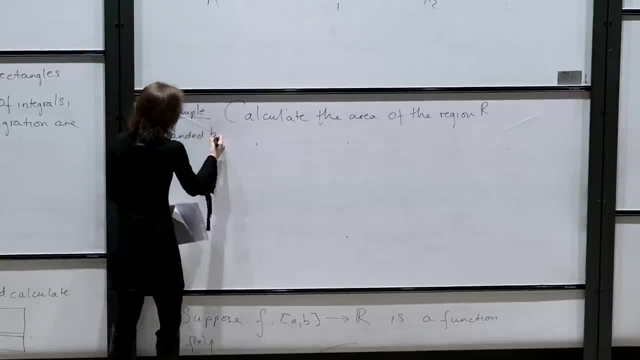 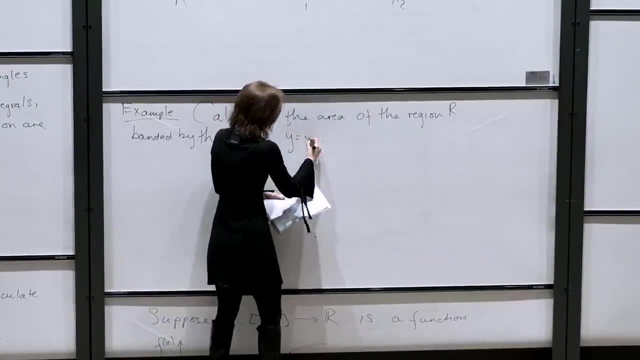 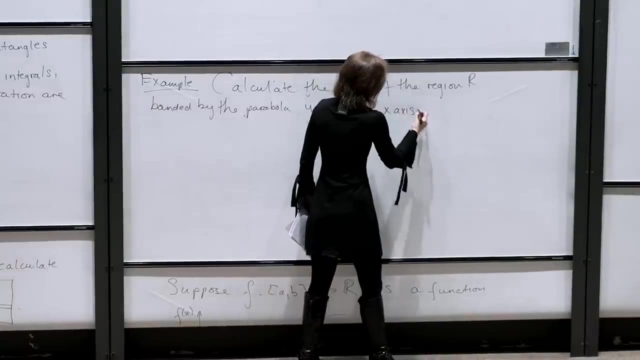 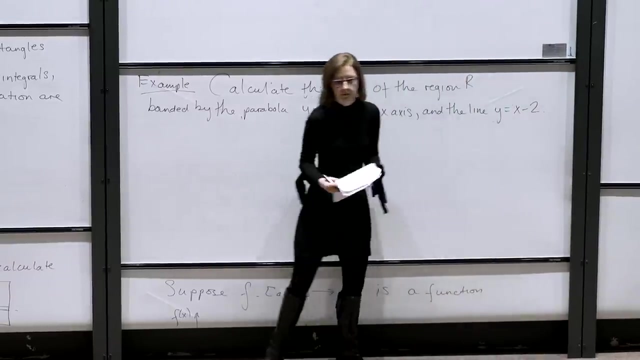 bounded by the parabola y equals root x, the x-axis, and the line y equals x minus 2.. Right? So when you're trying to calculate the area of the region, R bounded by the parabola y equals root x, the x-axis and the line y equals x minus 2. Right? so when you're trying to 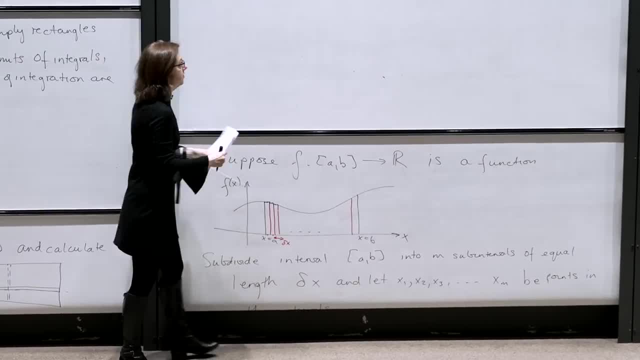 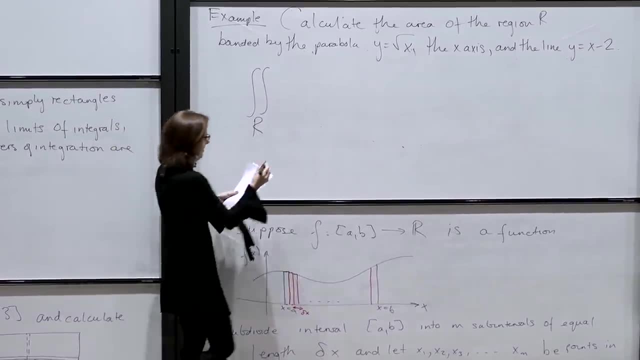 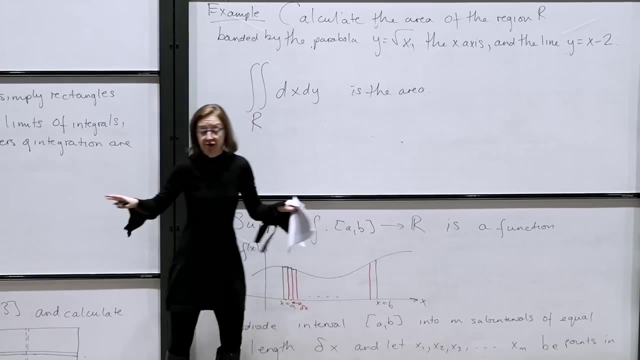 calculate the area. all you're doing is you integrate over the domain of interest which we're going to draw in a minute. so we'll just call that R, dx, dy. So that is the area. So you just divide the region of interest R into little. 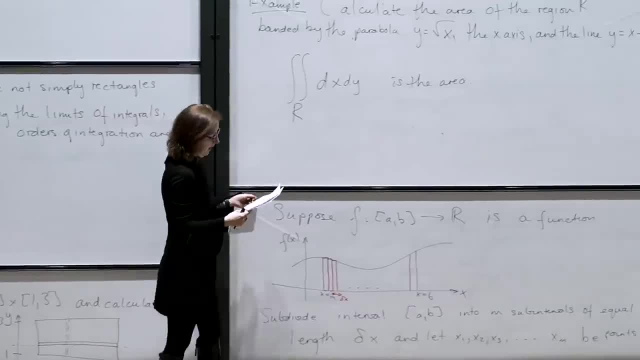 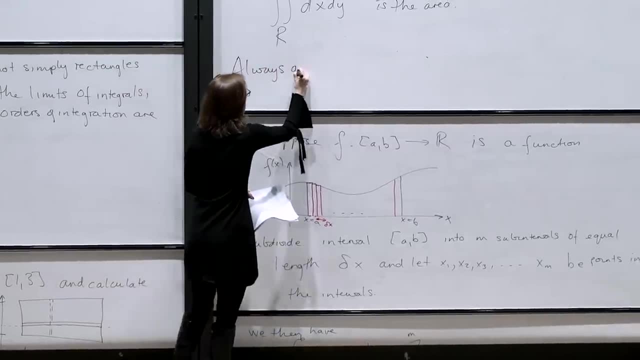 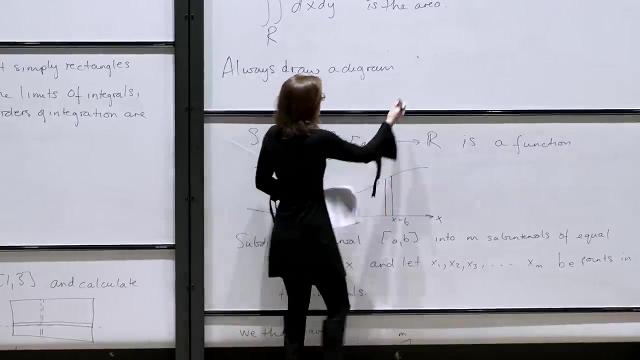 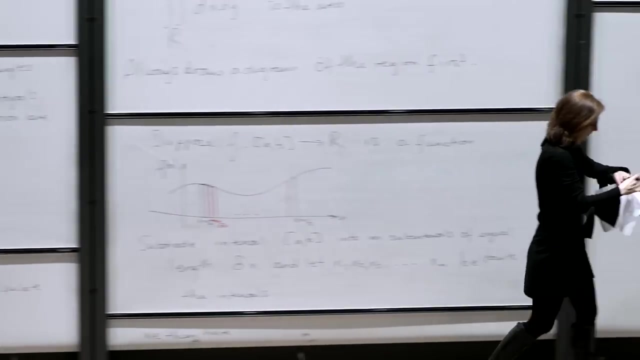 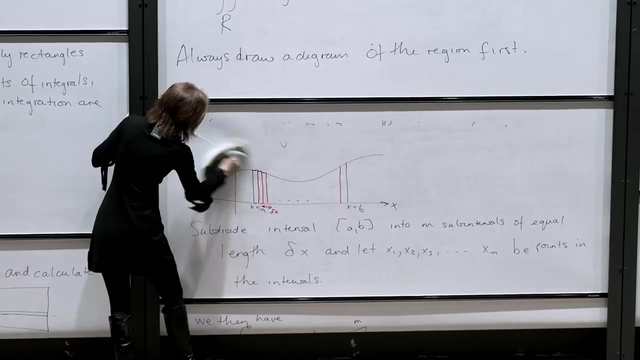 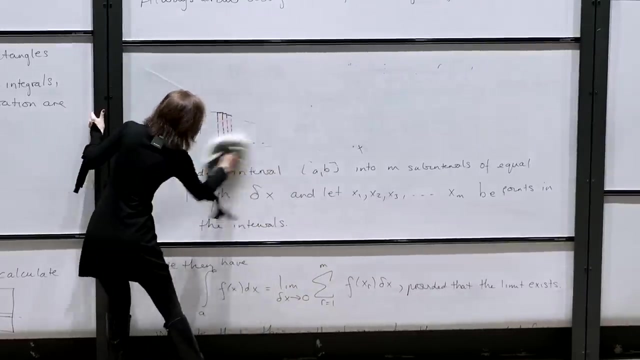 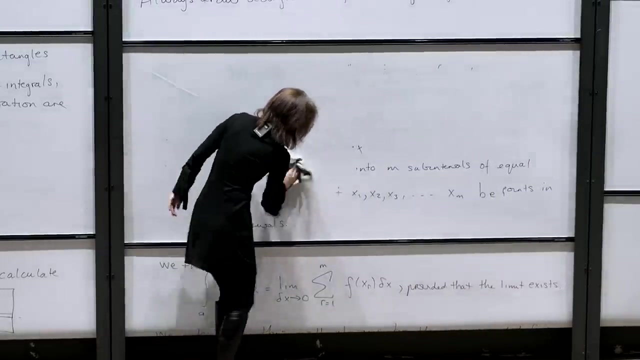 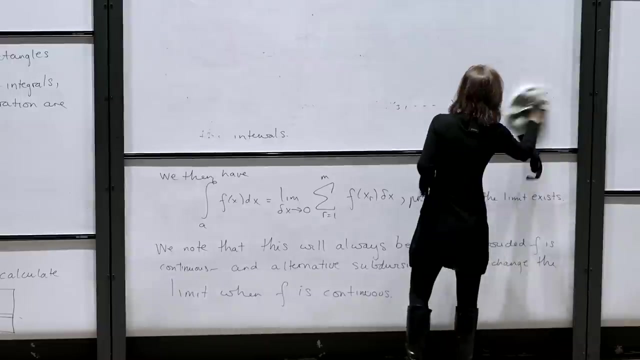 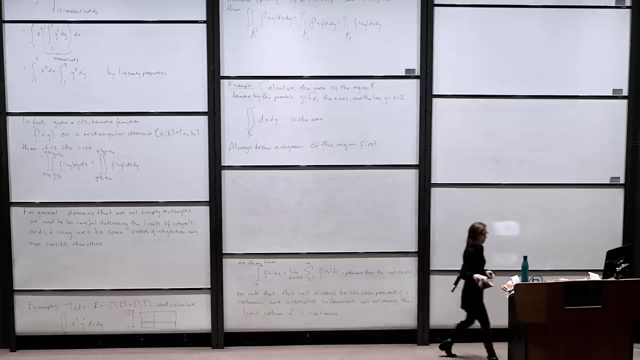 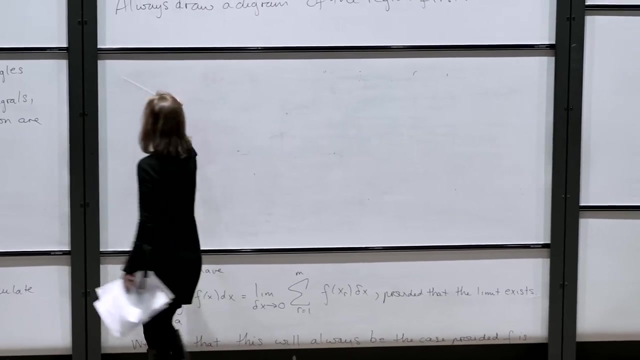 area elements. take the limit, sum them up and that will give you your area of the domain. Right: always draw a diagram. This is where most of the errors come in: the diagram of the region first right. so let's draw the region. so here's. 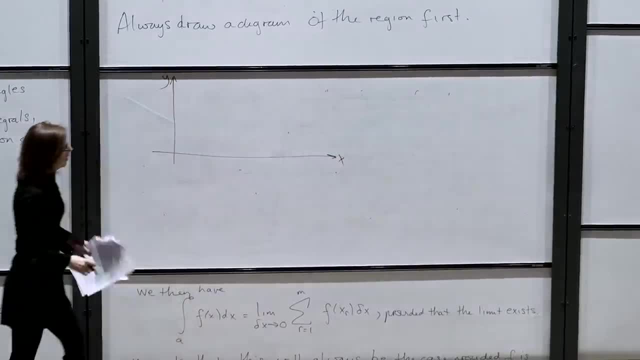 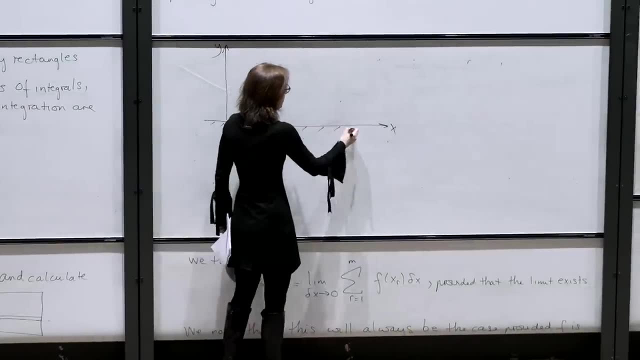 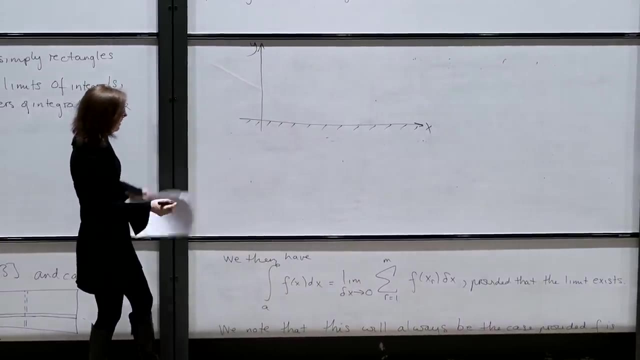 the x-axis. here's the y-axis. So the first bounding line of this region is the x-axis, so we can shade the outside of the region. Then we have the line y equals x minus 2, which looks something like this: so that's. 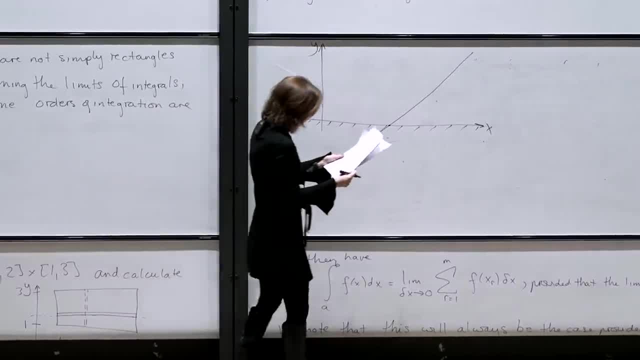 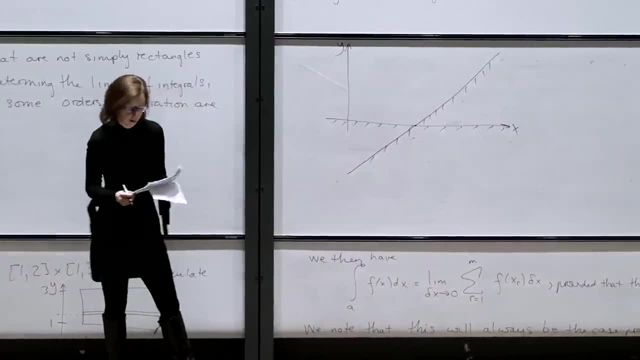 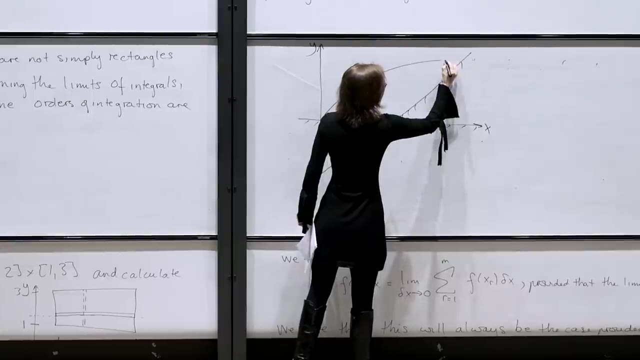 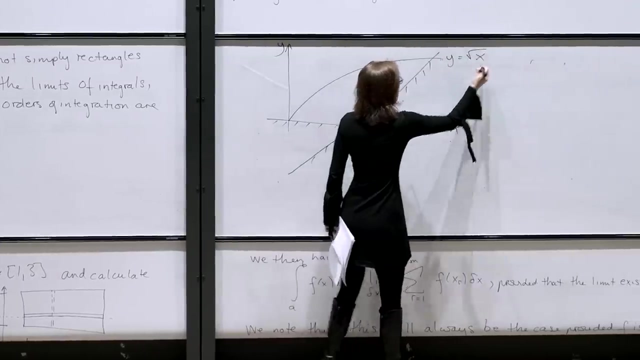 going to go through the point 2, so there's the outside of that region, And then we have the parabola y equals root x, which is something like this: It's got a very strange property, this parabola. So this is the line: y equals the square root of x, and so the shading indicates outside. 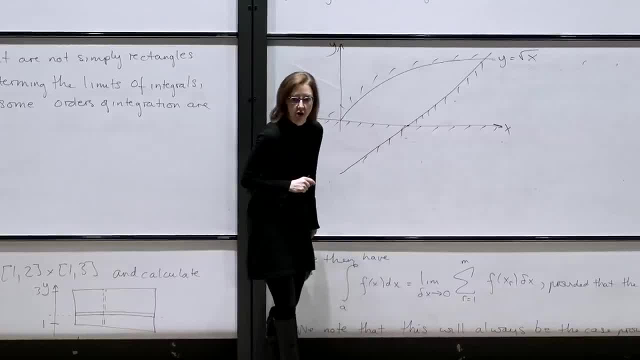 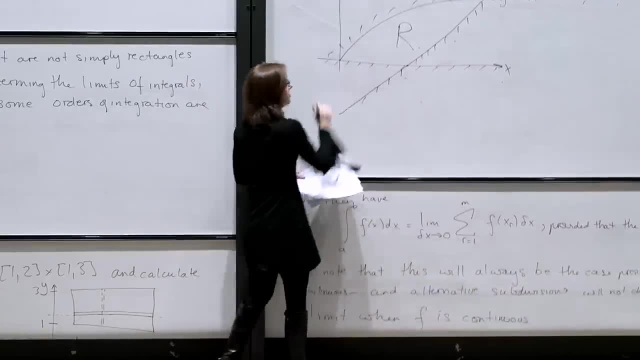 the domain. This is the region of interest that we're trying to find the area of. so this is the r. So, as I said, we can integrate with respect to x and then y or y with respect to x. So we're going to do it both ways and you can decide which you prefer. 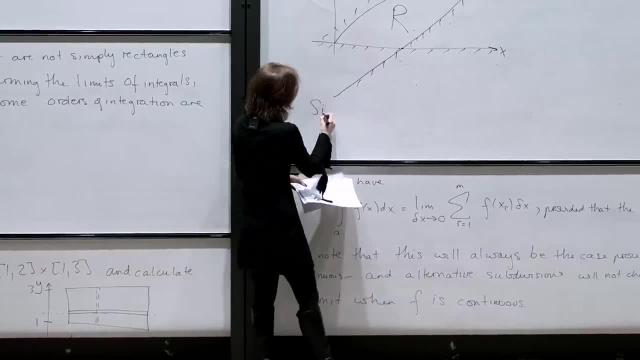 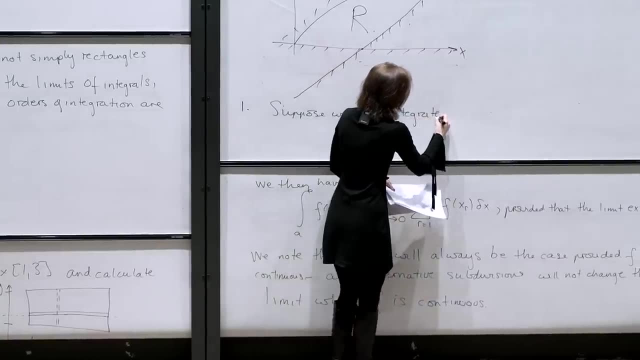 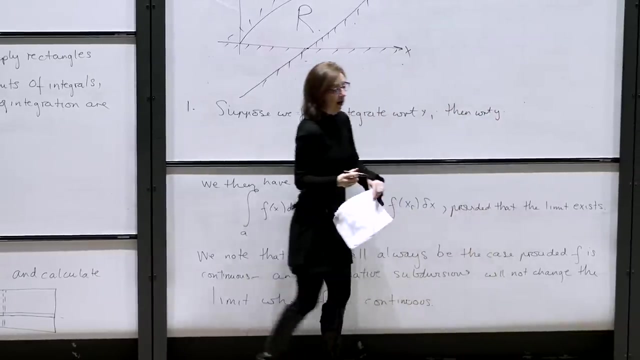 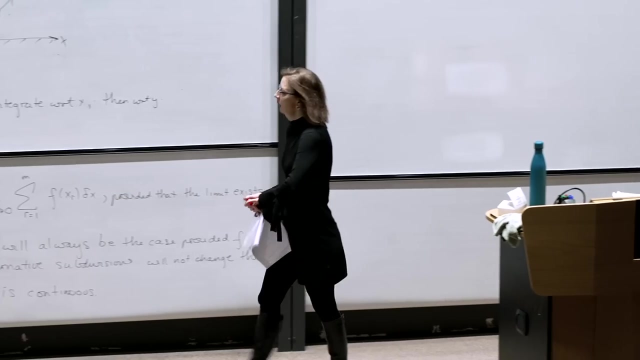 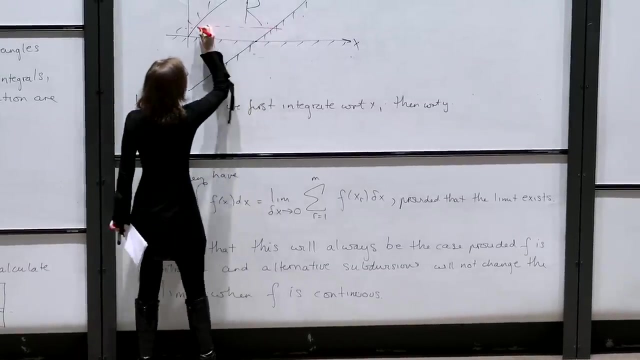 So 1, let's do the first way. So suppose we first integrate with respect to x And then And then with respect to y. So that means that we are dividing this domain into horizontal slithers. So yeah, we're going to fix y and go across this way. 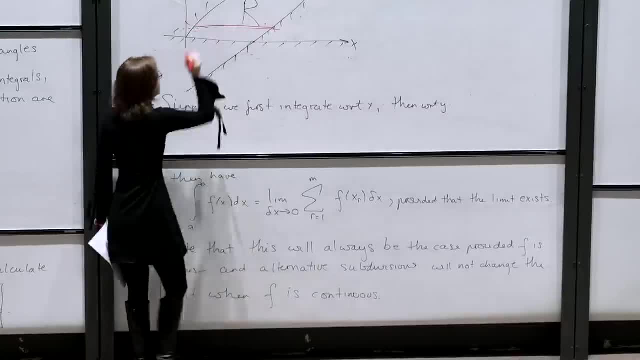 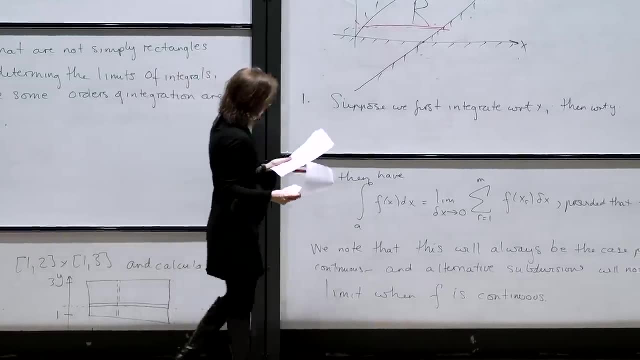 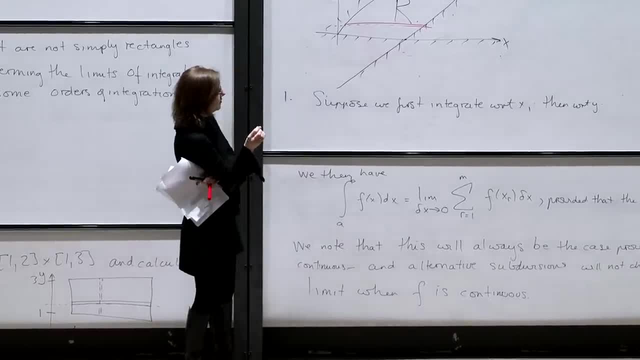 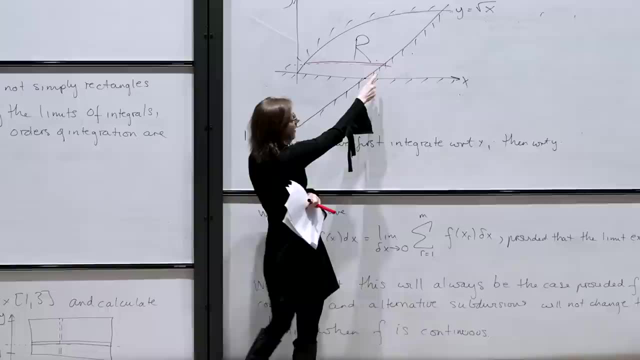 Okay. So we need to now be very careful in defining our limits. So if we're integrating first with respect to x, we're keeping y fixed, So x is going to go between whatever value is over here and whatever value is over here. 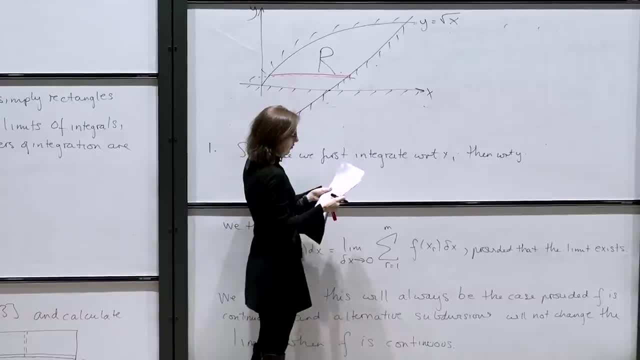 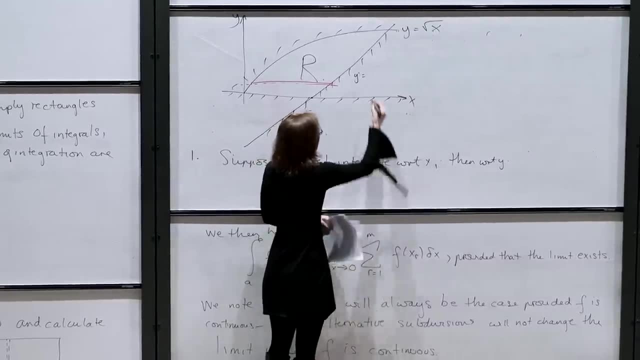 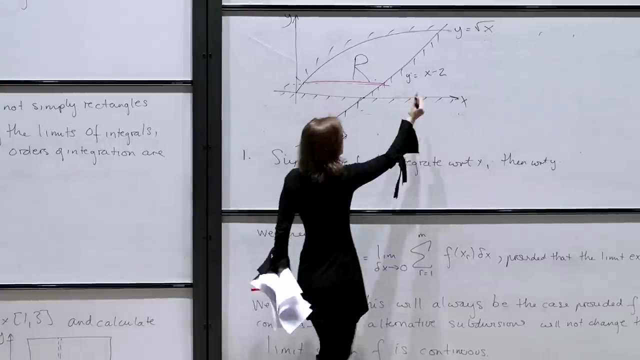 So this one's straightforward. This is just the line. What was it? y equals x minus 2.. Yep, So if I fix y, just treat it now as a number. If I rearrange this, I clearly get that x is y plus 2.. 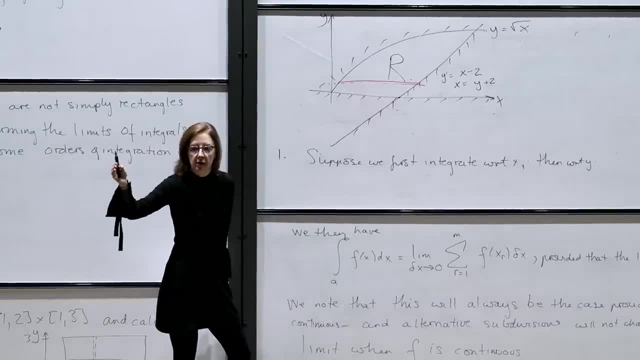 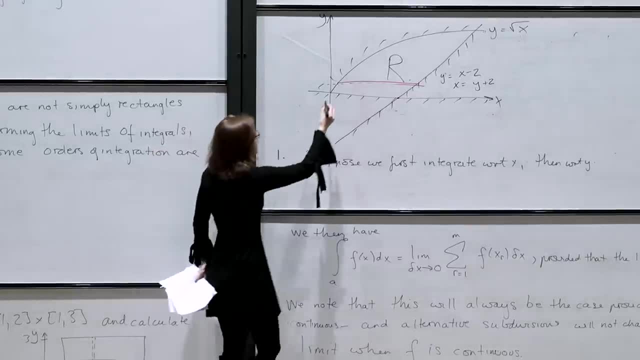 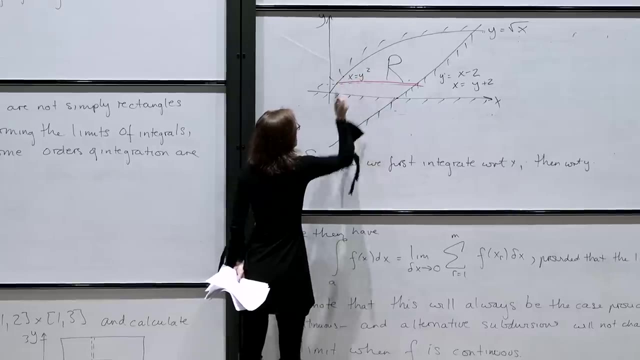 And so my upper limit for my value of x is y plus 2.. Now I go to the other side. So I've got- Currently got- y as a function of x, so y is root x, But I can write this as: x equals y squared. 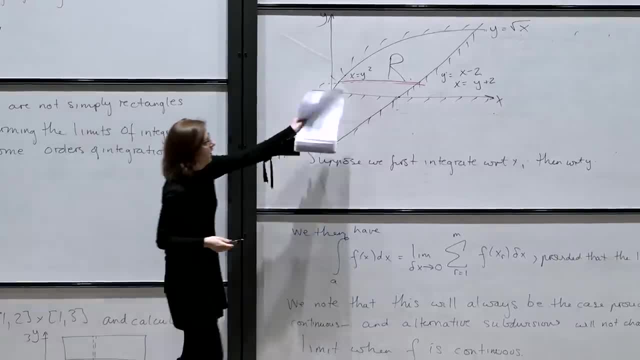 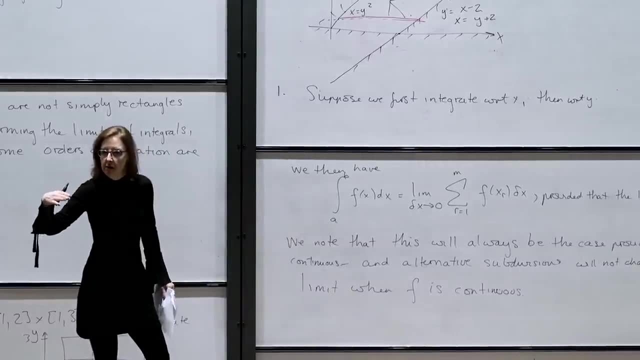 So the lower limit on my x integration is going to be y squared. So the way to think about this, You're fixing y, it's just become a number, and then you're just asking: well, what values does my x go between? 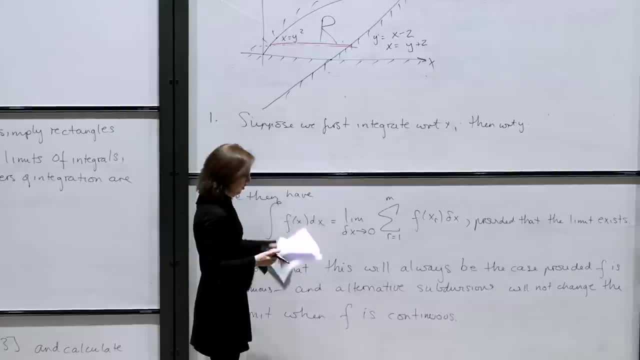 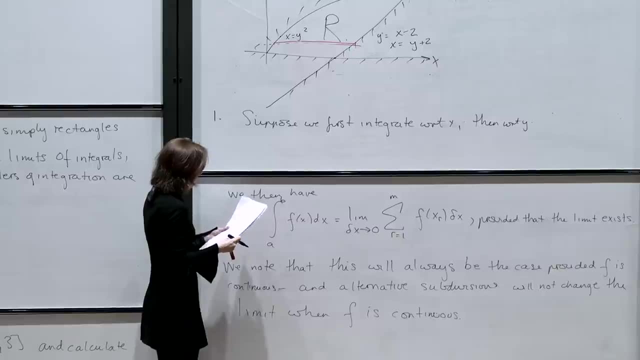 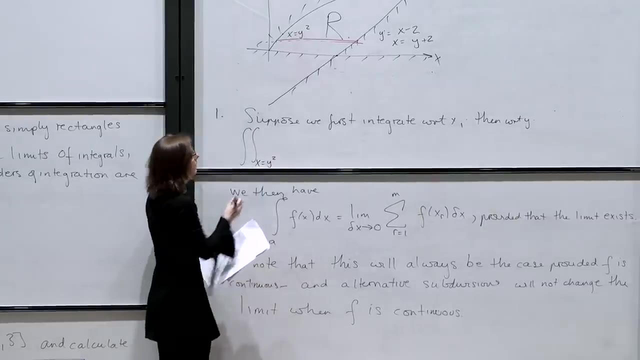 So the lower limit is y squared and the upper limit is y plus 2.. So, having defined that, then we end up with the area being the integral. So the lower limit is x is y squared and the upper limit is y plus 2.. 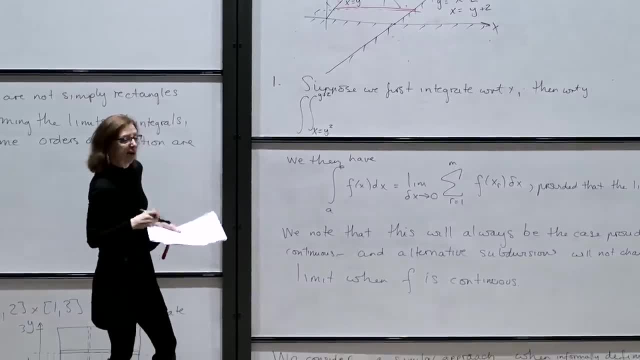 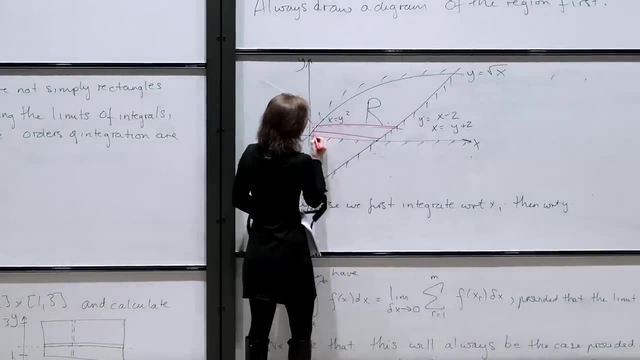 But then I have to do a bit more work because I don't yet know what values- Values of y- I'm going to pick. So I'm going to go through. every sliver is going to go from here all the way up to here. 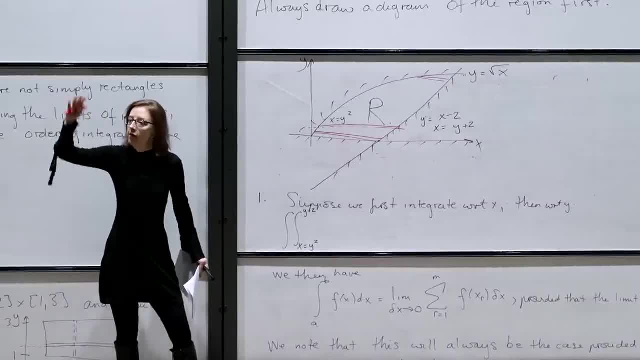 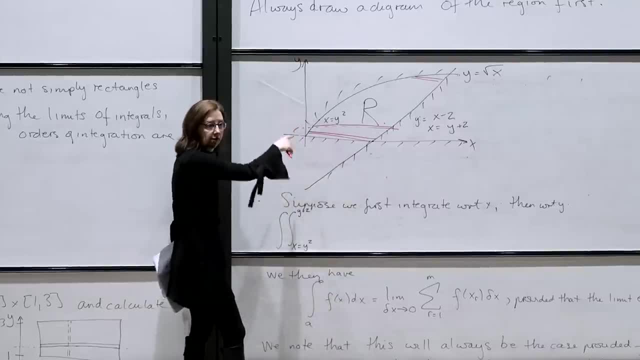 So as I go up, I'm picking through all those y values that the area is covering So clearly. I'm starting at y equals 0 because I start on this. x axis is the boundary of my domain, But what's this value over here? 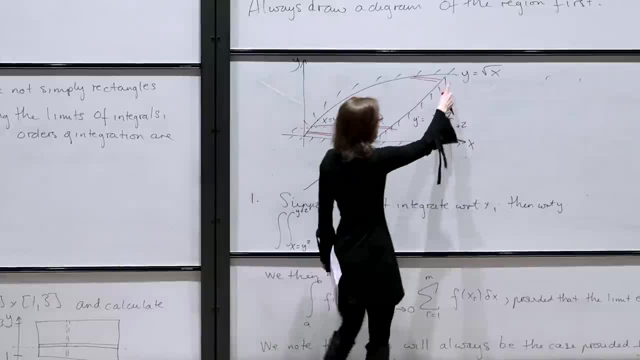 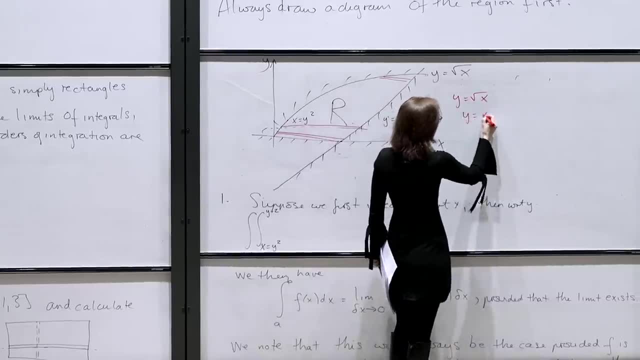 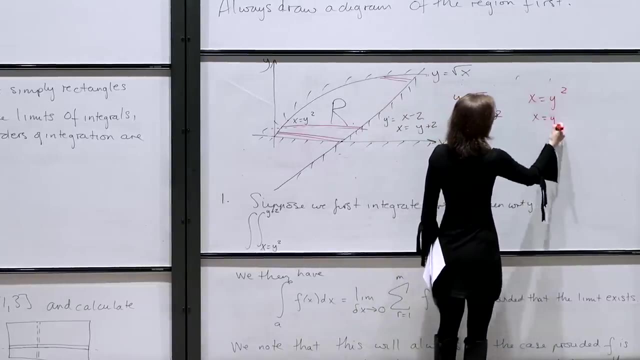 So what's my maximum value of y? So that's going to occur. To work that out, To set y equals root, x has to be equal to y, equals x minus 2, which is probably easier to say: x is equal to y squared x is equal to y plus 2, and solve that. 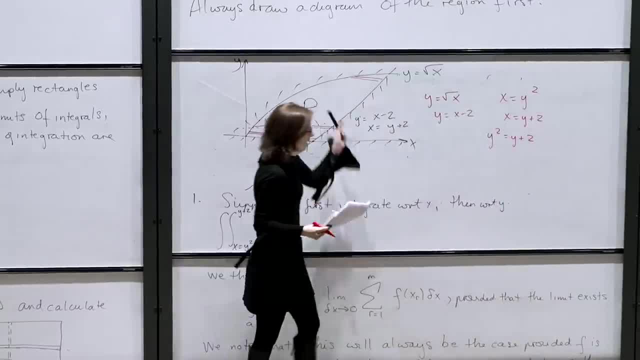 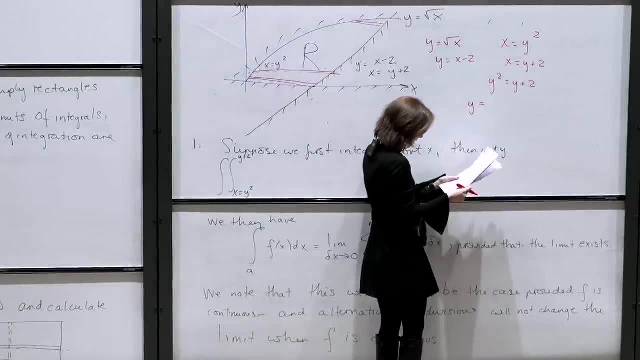 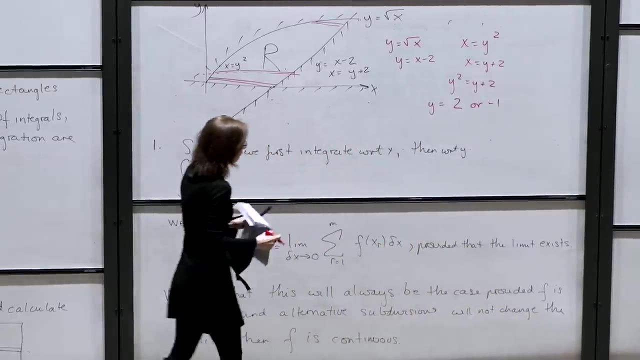 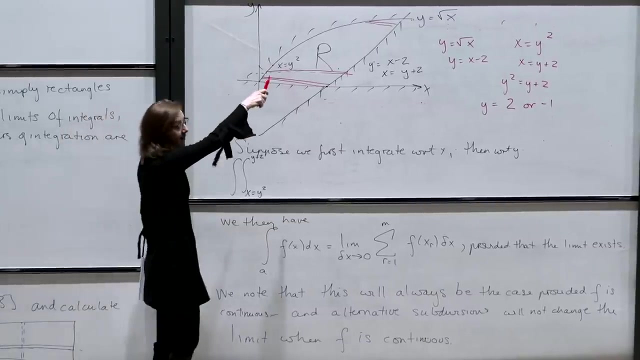 So y squared equals y plus 2.. And so that tells you y is equal to 2 or minus 1.. I think are the solutions of that problem. Now, clearly, y is positive, because I'm going up into this part of the plane- 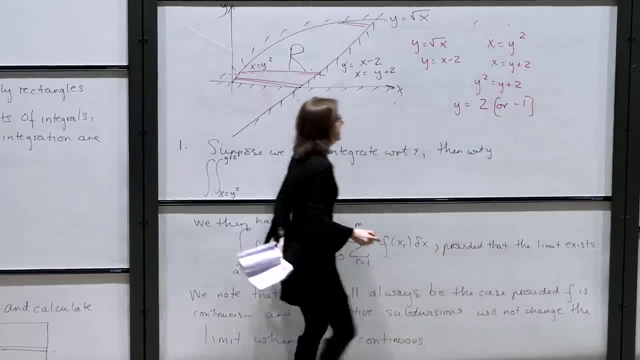 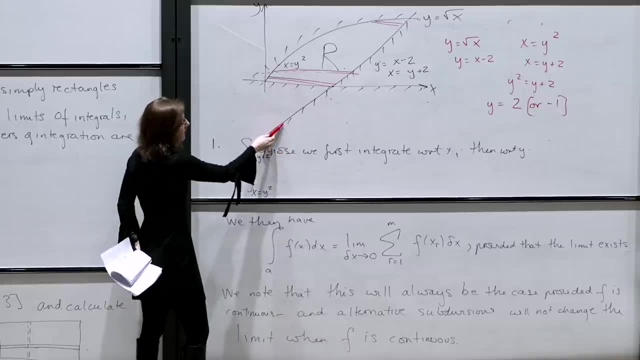 So I don't want this solution. So this one corresponds to the other solution. If I extend this parabola into the lower half of the plane where it interacts with this line would be given by: y equals minus 1.. So we don't want that one. 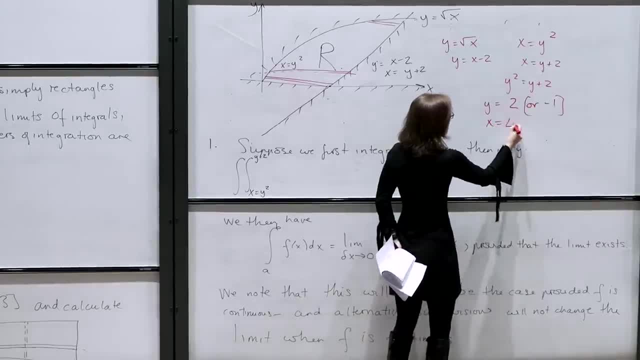 And I also need to know the x value. So when y is 2, then clearly x is equal to 2.. So that's the solution. And if I extend this parabola into the lower half of the plane, then clearly x is 4.. 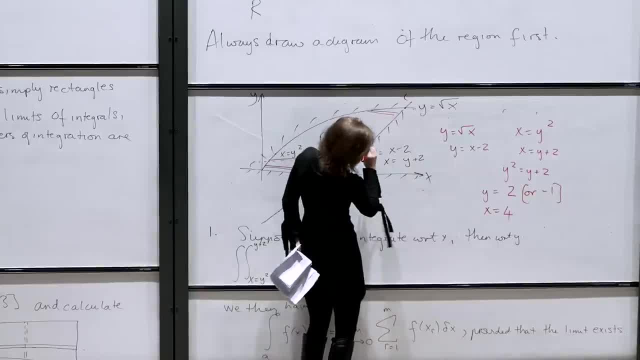 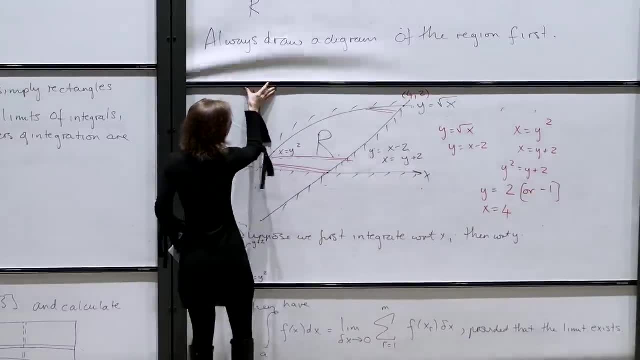 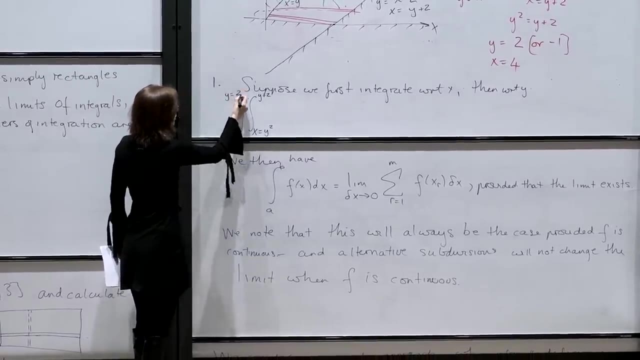 So this point of interest up here corresponds to 4, 2.. So I know that my y limits then go between y equals 0 and y equals 2.. So I take all those horizontal slithers and sum the whole lot up. 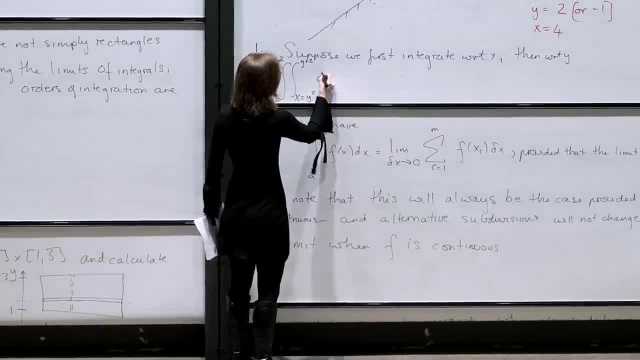 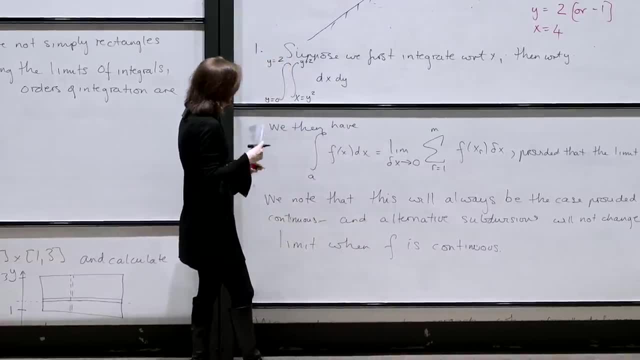 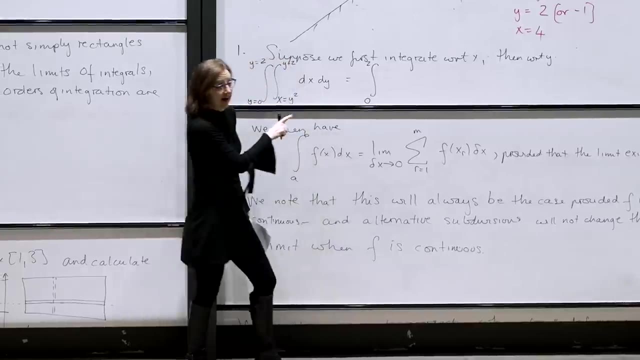 And then I get. What am I integrating? It's just the area. So d, x, d, y, Okay, So that just becomes the integral from 0 to 2 of So now I integrate x with respect to x rather, so it just gives me x. 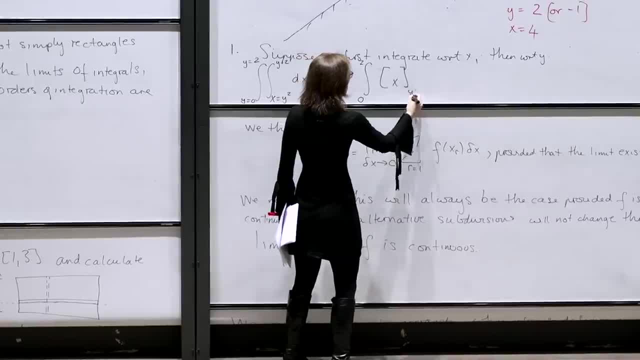 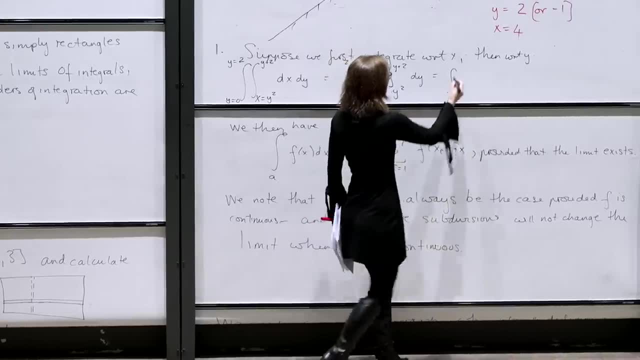 So I get the value of x evaluated at y squared and y plus 2, d y. So that's the integral between 0 and 2 of y plus 2 minus 2.. Okay, Okay, So I get minus y squared d y. 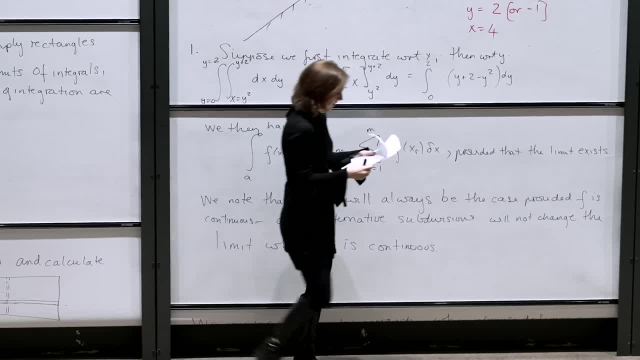 And that's very easy to do, And I won't give all the details. That's just 10 thirds, So the tricky bit of this one was just thinking about the limits. But the good thing about doing it this way was I only had one calculation to do. 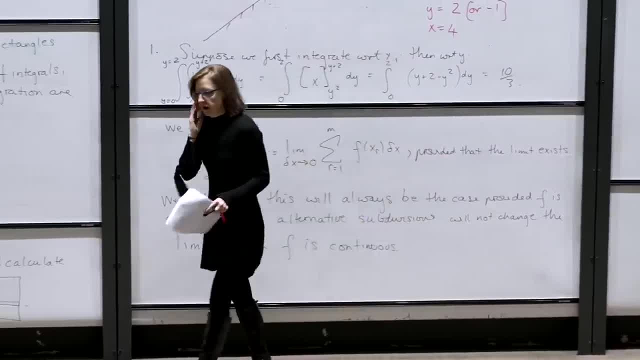 So I only had to. Once I'd worked out my limits, I can crack on and do it, And I only really had to work out one integration, which was here, By which I mean I didn't have to split up my domain. 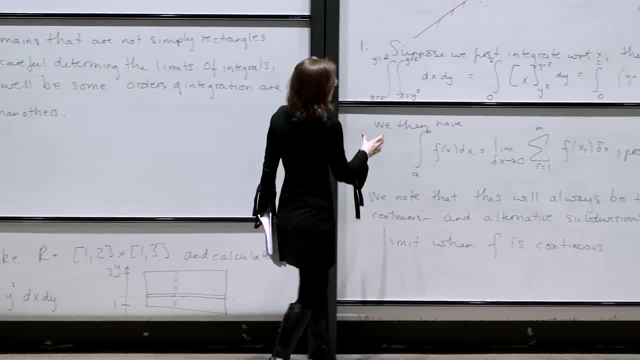 So let's do it the other way round. I'm gonna go back to my previous example, So I can crack on and do it, And I only really had to work out one integration which was here, By which I mean I didn't have to split up my domain. 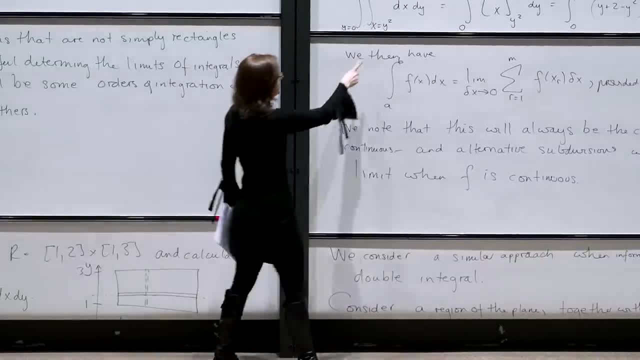 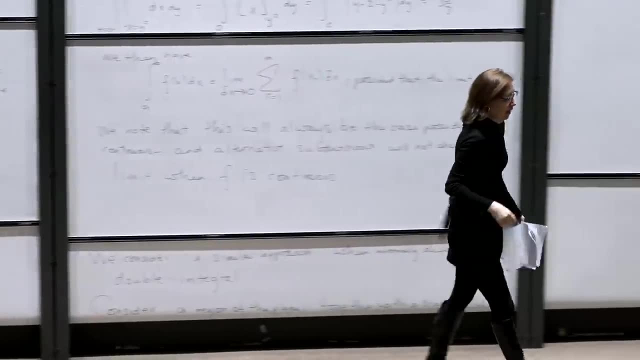 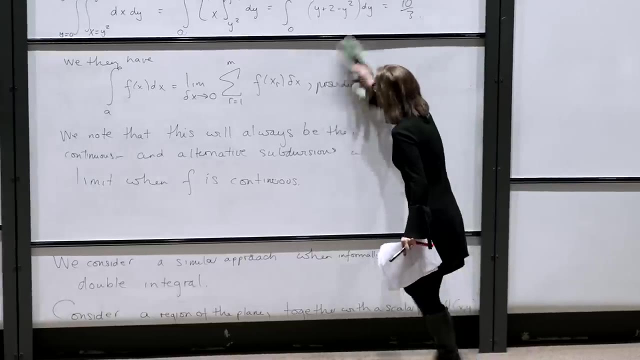 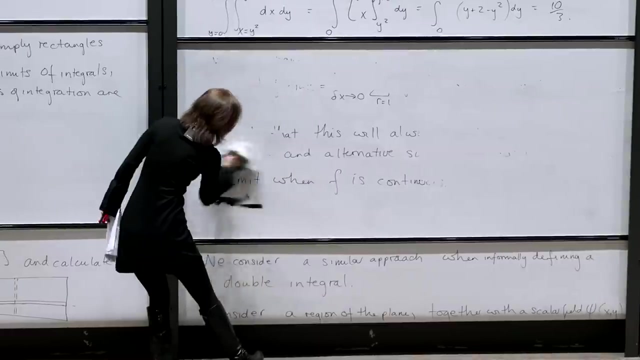 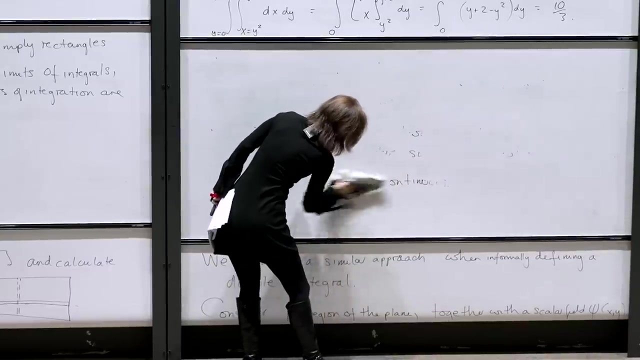 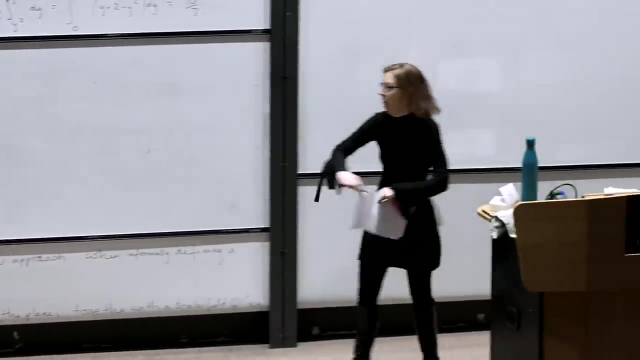 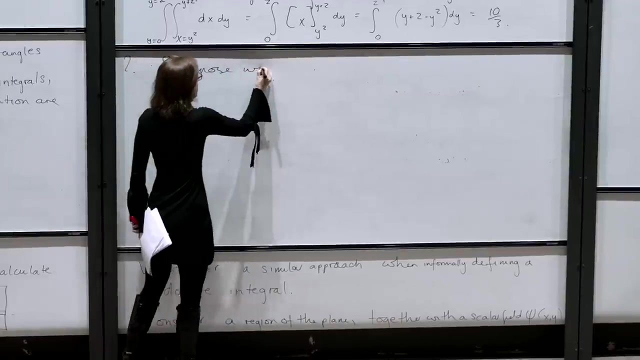 So let's do it the other way round, And I'll illustrate that that way, although perfectly viable, turns out to be a bit more work. Okay, so if I do it the other way, so 2, so suppose we first integrate with respect to 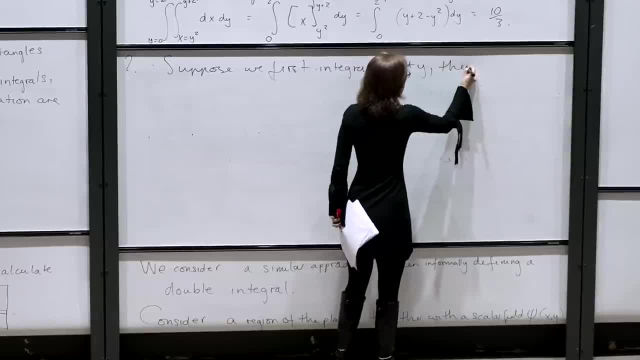 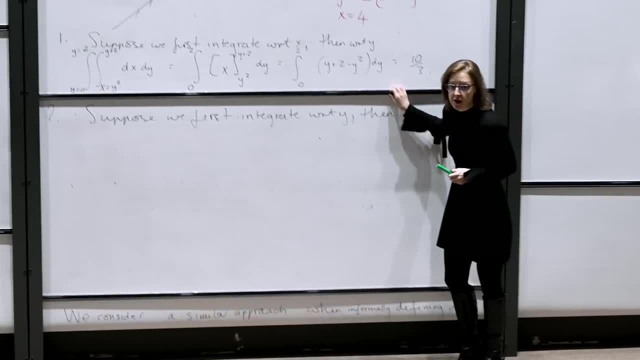 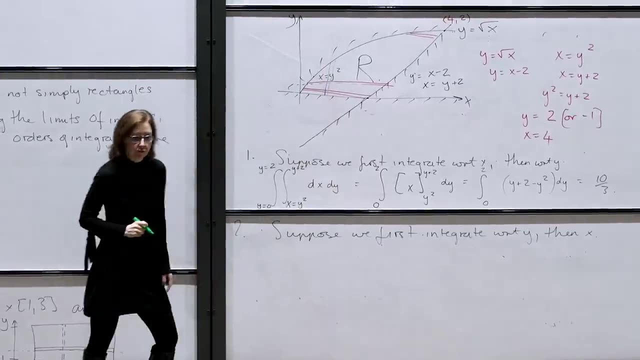 y, then x. So now let's look at my domain again. So now if I'm holding x fixed, I'm doing vertical slivers, So I start to do this kind of problem. So over here it's straightforward because I'm 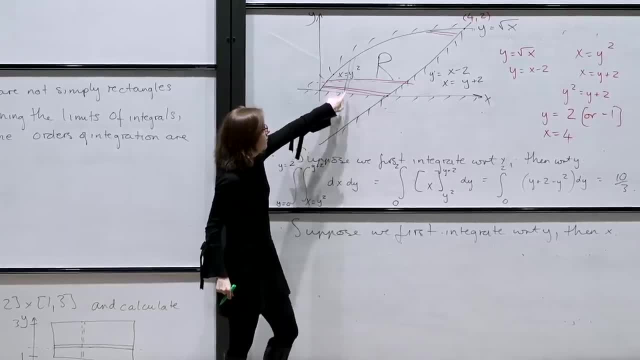 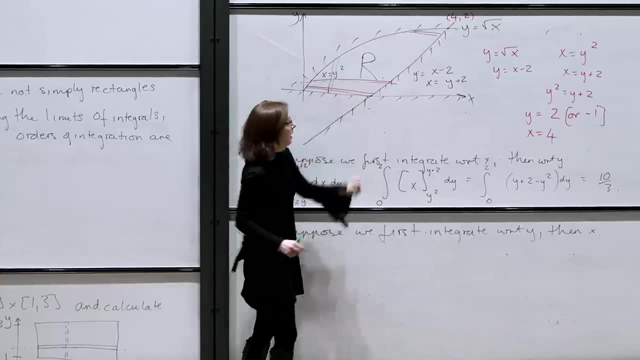 always going between the y-axis being y equals naught and whatever value of y. I have up here which is root x, when I'm holding x fixed. But now, as I go along, I become over here. Oh, that's a terrible pen. 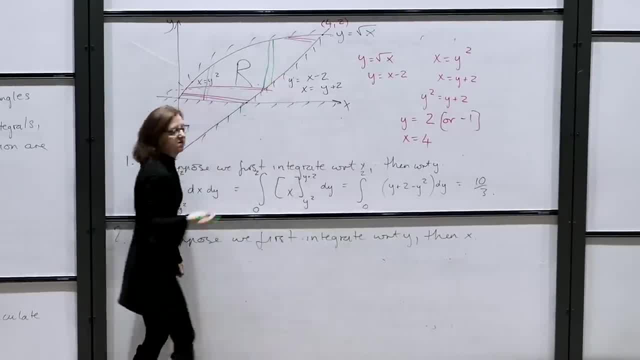 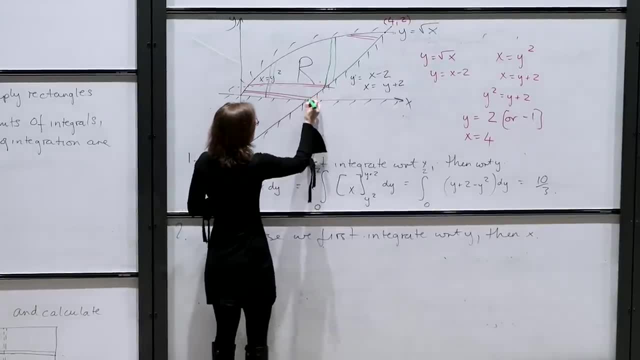 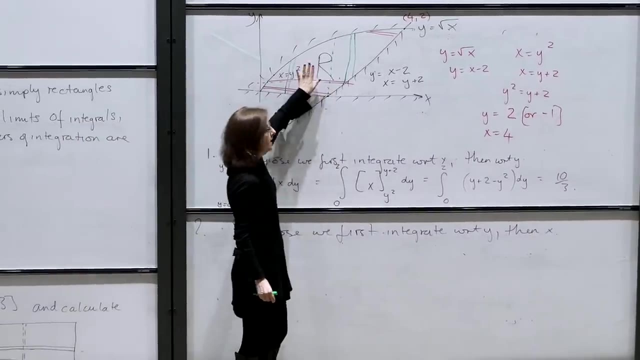 And now my lower limit has changed. Now it's not that hard. We can certainly do it, But what I'm having to do now is split my domain into two parts. So at this point, this is where I can use that property of domain splitting that the integral over r is the same as the integral over 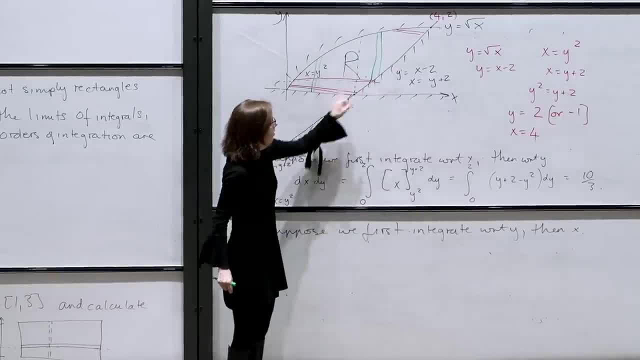 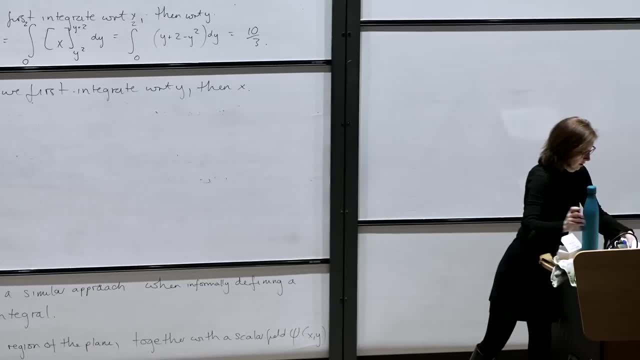 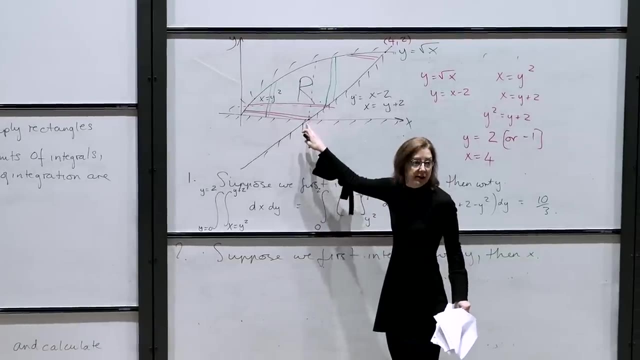 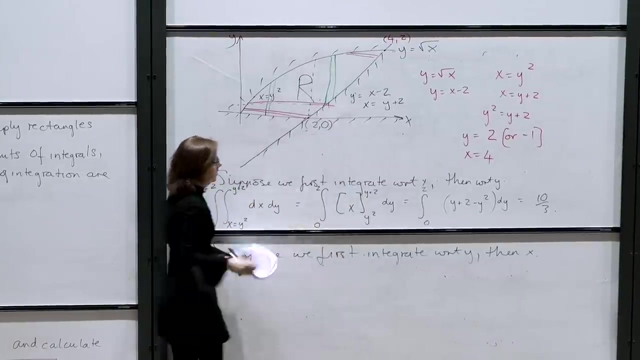 this bit plus the integral over this bit And the limits of my integrals. So I now have to compute this point here, because this point tells me where I have to change the limits on my integral, And so I hit this x-axis at the value 2, 0.. So when I'm thinking about 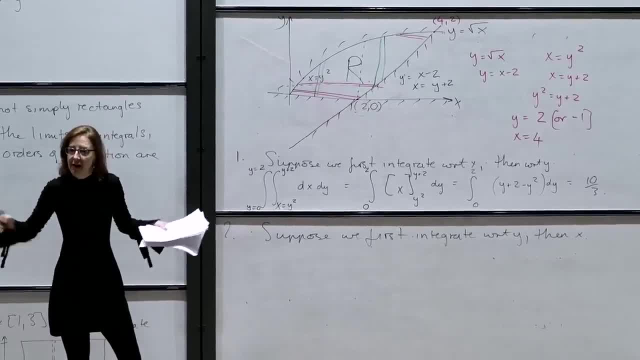 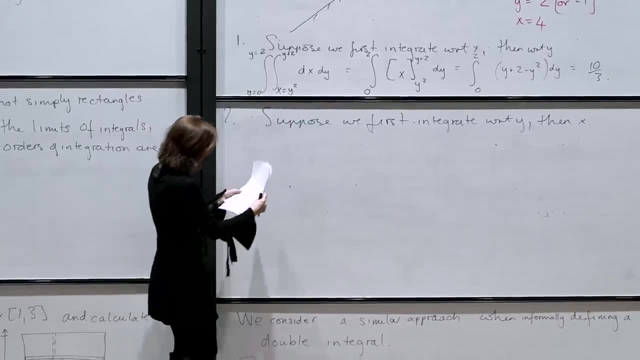 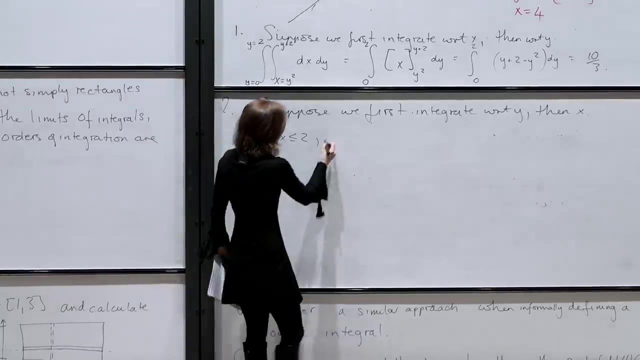 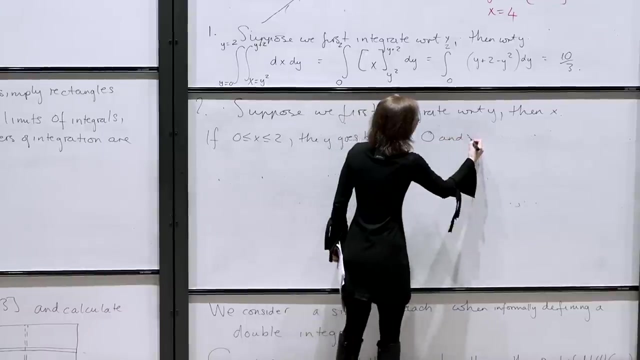 doing my vertical integration and then summing them in the x direction, I have to split my x values up. Okay, so if x is between naught and two, then y goes between 0 and the upper limit, which is root x. 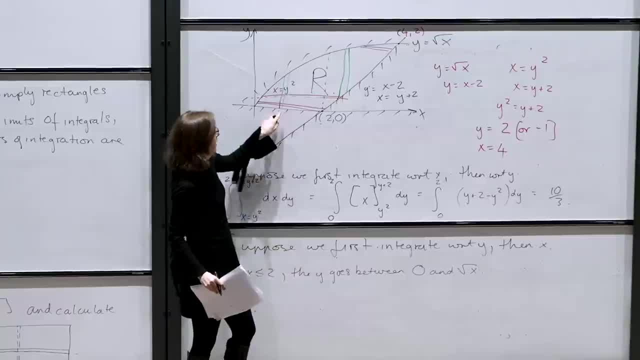 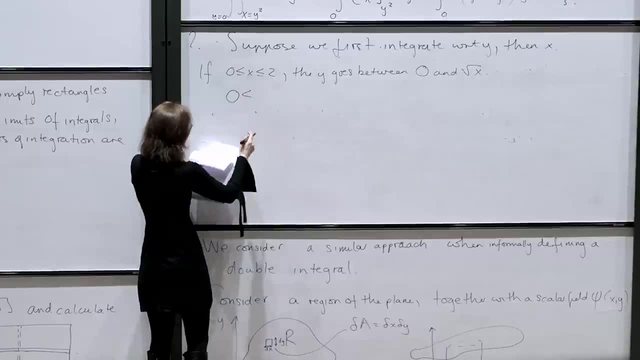 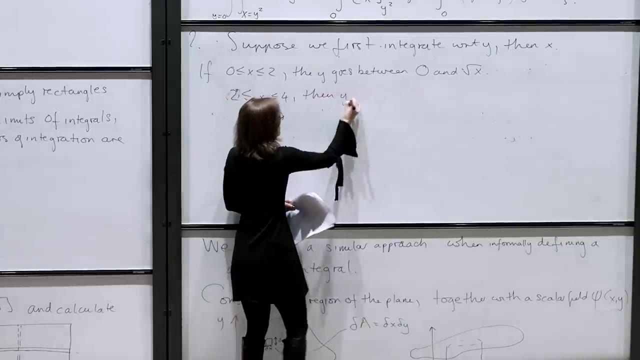 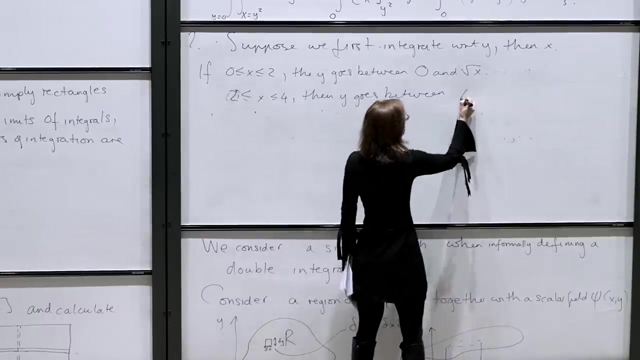 So, provided I'm over here, the lower limit will be 0 and the upper limit will be root x. Now, if x goes between 2, then y goes between. So now the lower limit becomes x minus 2 and the upper limit is still. 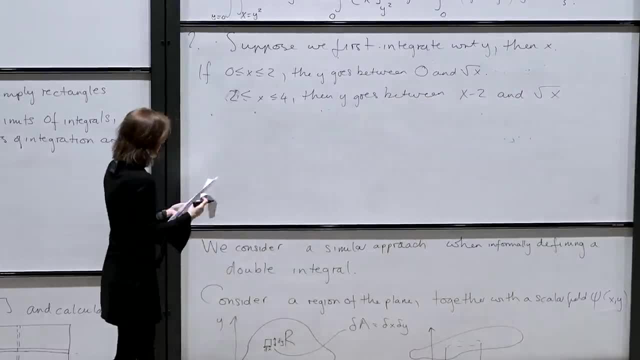 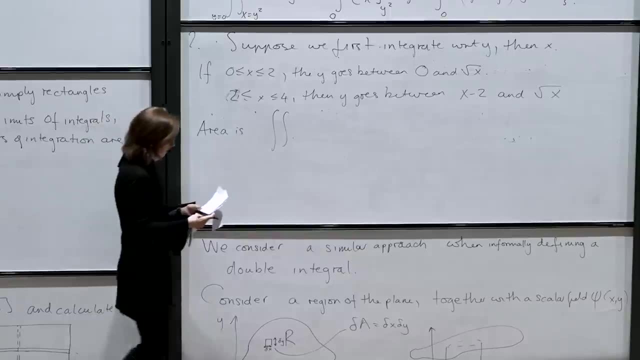 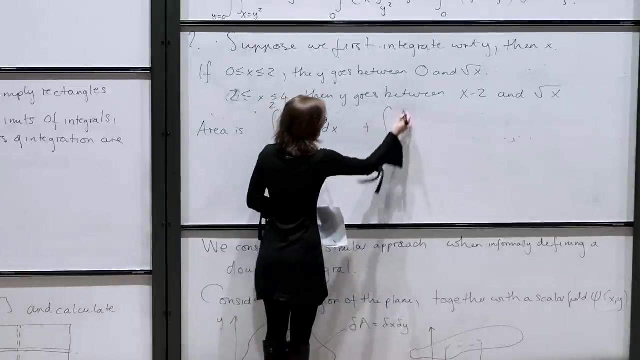 root x. So now the area is the integral, So the first integral. I do so integrating with respect to y first. So I'm going to consider x between 0 and 2. And then my lower limit is 0 and my upper limit is root x for the y integration. And then I have to add to that the other bit. 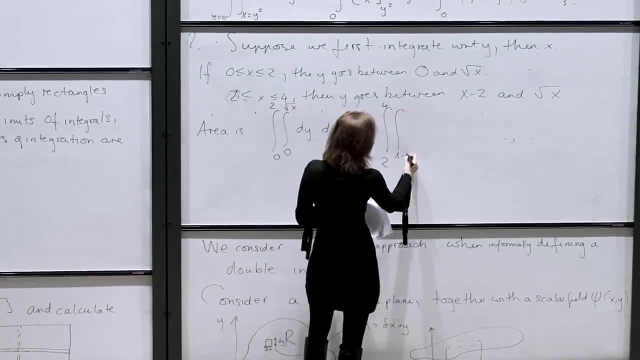 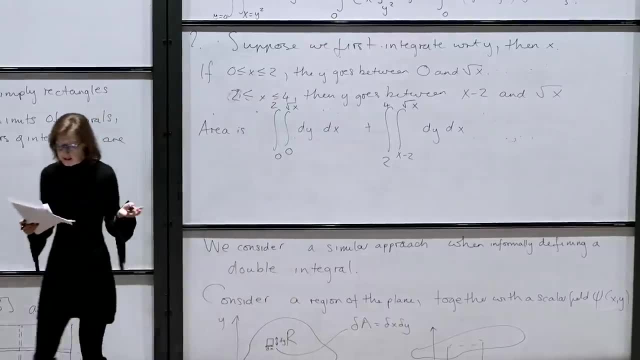 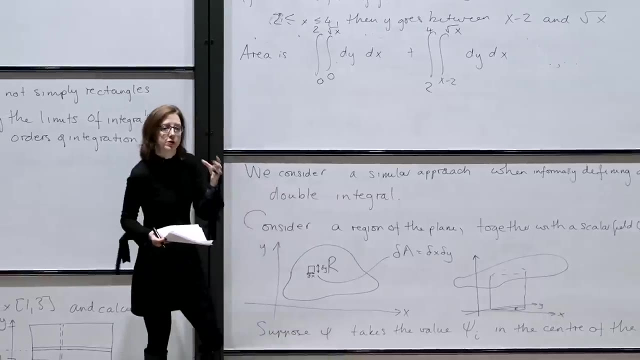 where now my lower limit is x minus 2 and my upper limit is root, x, dy, dx. OK, so this particular example, I mean it's fine, You can do these two integrals, It won't take very long, But there is an additional step to doing it this way. So if you work all that through, 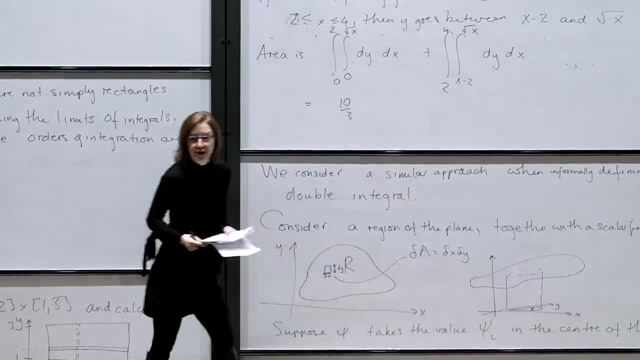 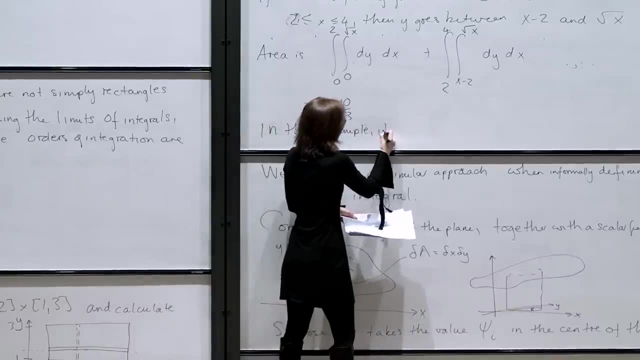 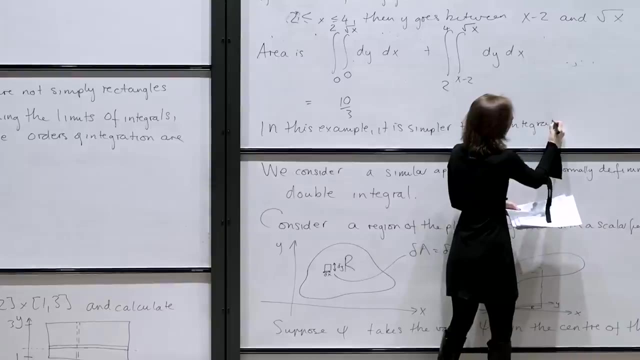 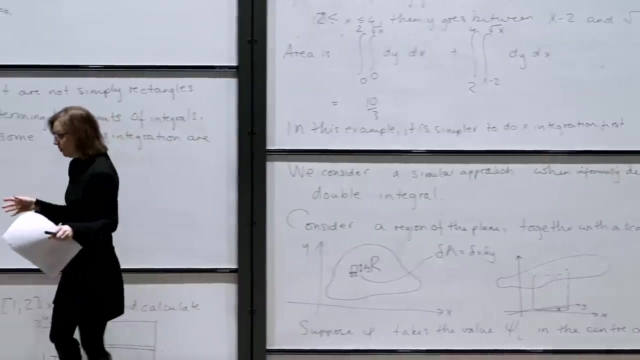 and I won't do all the detail, you'll get the answer: 10 thirds, as you'd expect. So in this example, it is simpler to do the x integration first. OK, So what we've done today, So what we've done today is we've thought about integrating over simple regions, which 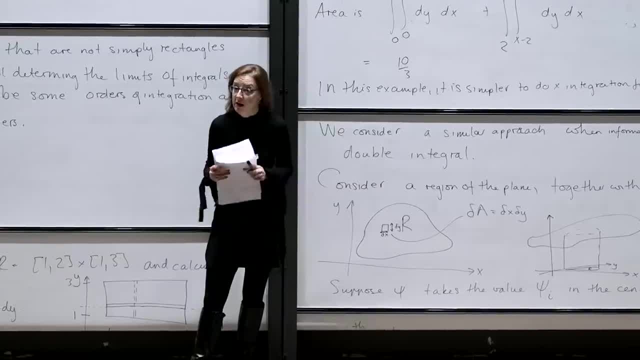 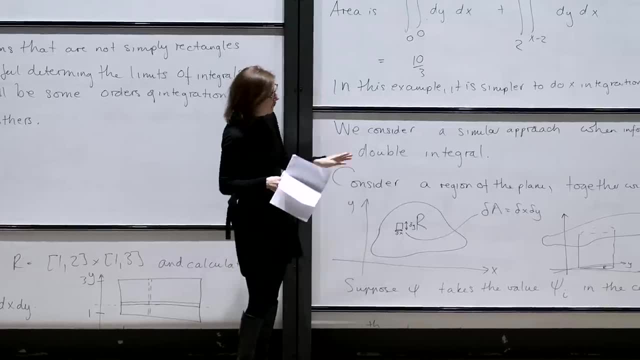 are just rectangular, where everything provided f, is well behaved, everything is well behaved, And we thought about how to think about more complex domains, where you now need to think about the order of integration. Often we think about integrating over domains, So sometimes 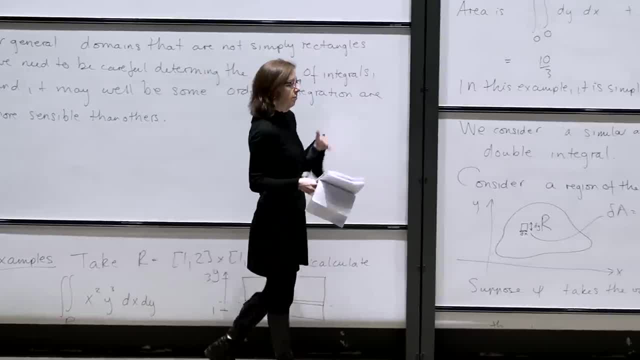 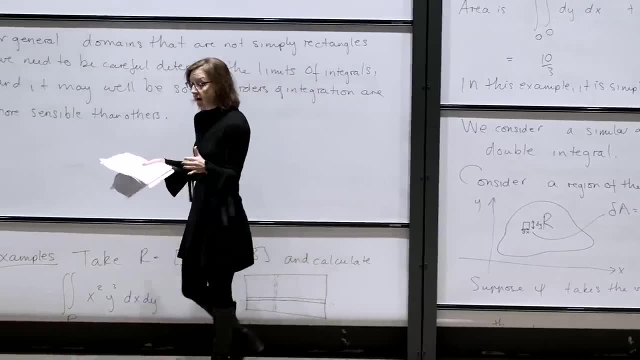 the domains are circular or they have a particular geometry, where it's more appropriate to actually use a different coordinate system altogether. And you'll have seen already how you can. instead of integrating over Cartesian coordinates, you could use, for example, polar coordinates. 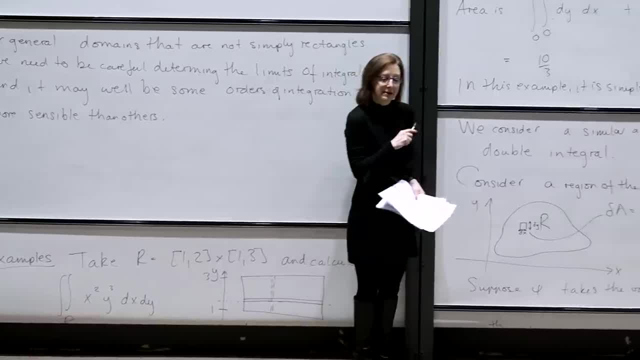 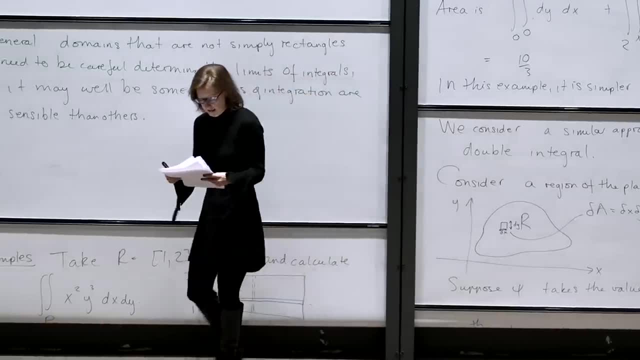 And so what we're going to do in the next lecture is think about more complex domains where making a change of coordinate system and exploiting the Jacobian actually makes your integration step a lot easier. So we'll stop there, and tomorrow I'll pick that up. Thank you.